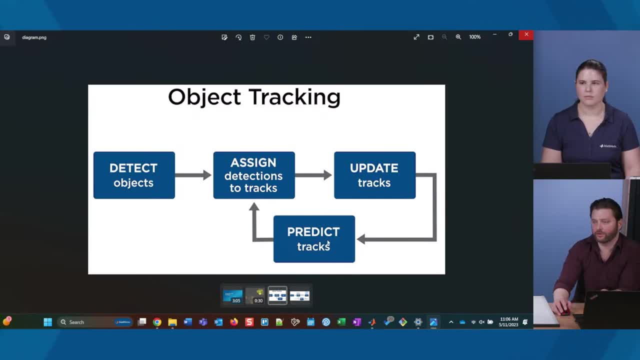 saw me walk behind her, you probably assumed I was going to come out the other side. That's your prediction. So then when you detect me again on the other side, you assign that's me again, right, And you update that in your mind. So that's roughly what this process is doing. But you know you do it a lot better than computers do. but we have to try with computers. 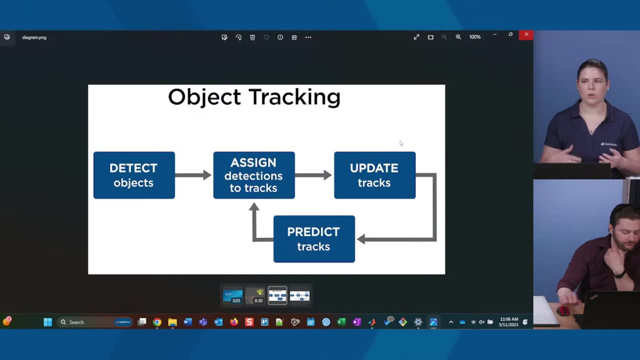 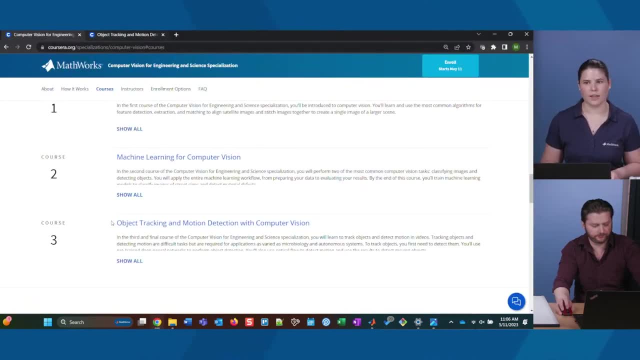 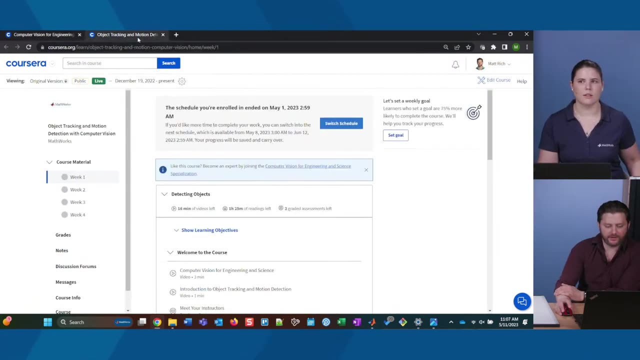 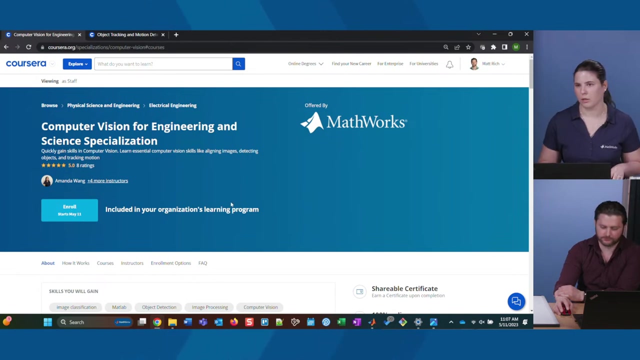 And just for those of you tuning in now, the course that we're referencing is part of the specialization on Coursera: Computer Vision for Engineering and Science. So when we say that course, we mean it, We mean this specialization. And then the specific course we're talking about today is object tracking and motion detection with computer vision. Yeah, But there's other stuff in there that you'll find really interesting If you're into computer vision. we do some machine learning both for classification and object detection. We talk about features. There's lots of good stuff we won't have time to get into today, So check it out. So we've talked a lot about, or a little bit about, the theory of detection- I'd like it to be a little, and tracking I'd like to be a little more concrete. 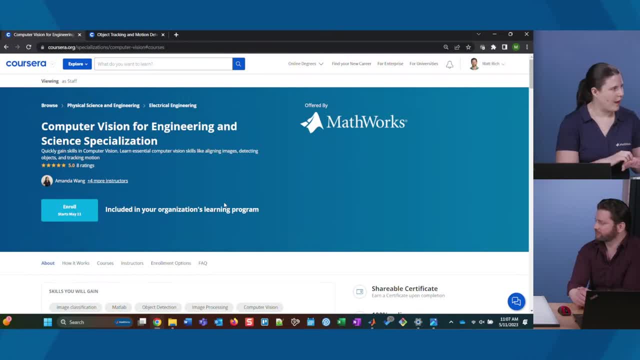 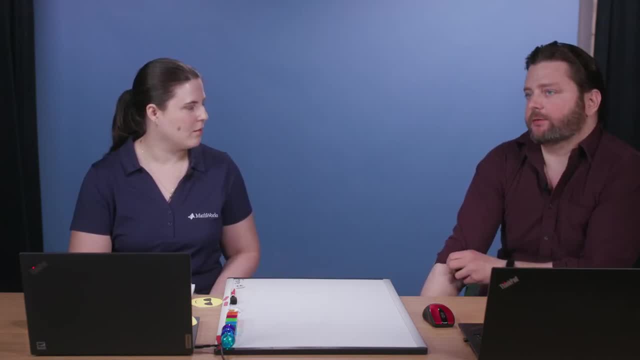 So why can't we just track an object? Why can't we just detect an object in every single frame, Like: what's, what do you get from tracking it? What's? Well, you know you get the object, permanence, but you also you know you might not see it every frame and you might not see it perfectly every frame. Now, the examples we're doing here are pretty simple. right, We've got a webcam five feet from us, but you can imagine, generally, when you're tracking objects, you know you might not see them perfectly. You might not be using a purely visual camera either, So you know you could get some detections that are actually you know not where you think the object is. 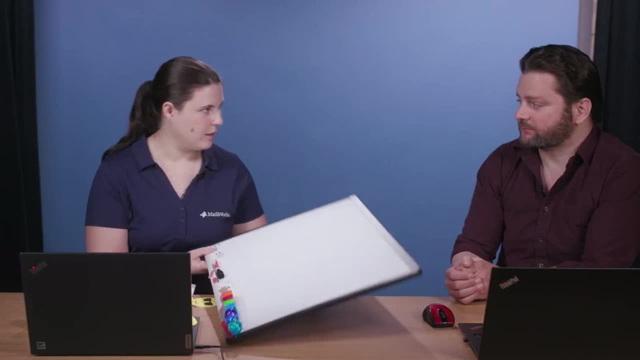 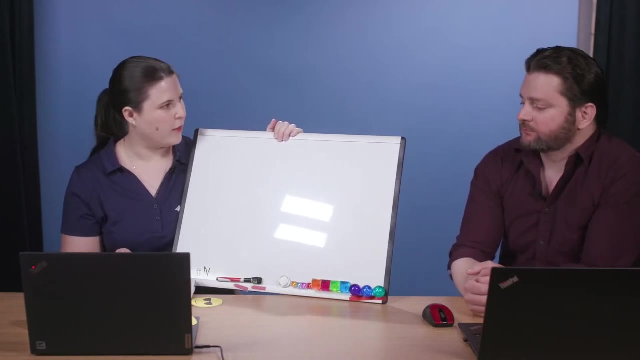 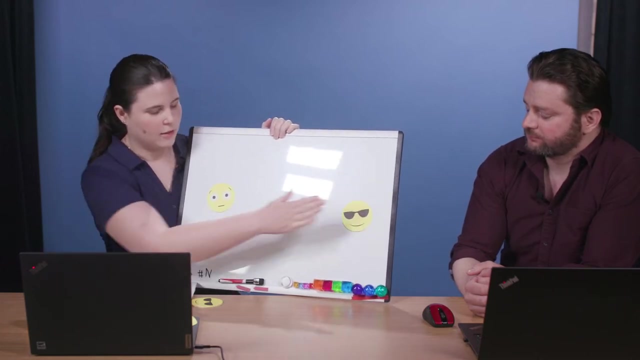 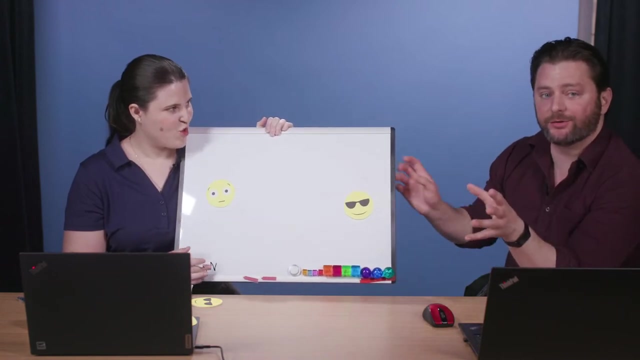 It should be. So detection is part of tracking. Let's talk about some of the other parts. We talked about the workflow. Let's make this a little more concrete. So let's say we are, we have a video of some real world objects. So this is going to be. this is me here, This is Matt. So we've got a video and in the video. But remember that the computer doesn't really see this. You do and you see it on the video display, But what the computer is seeing when it's detecting these things, it could be some sort of segmentation. 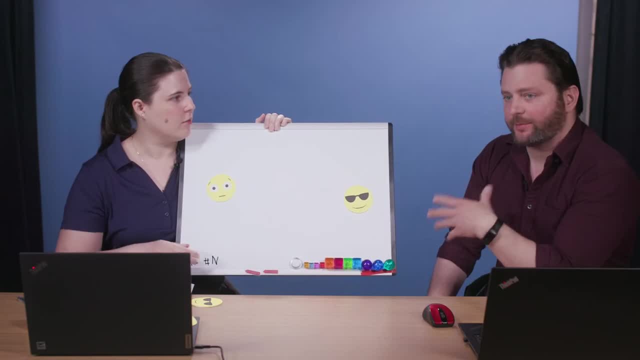 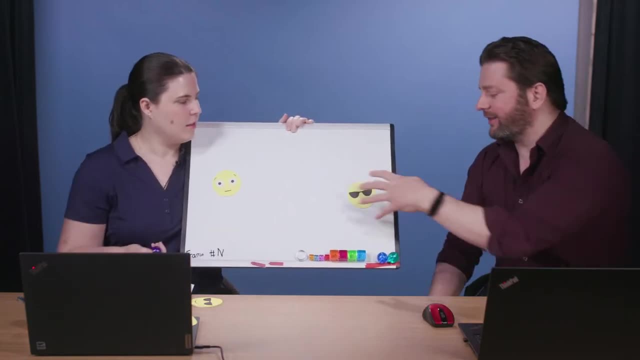 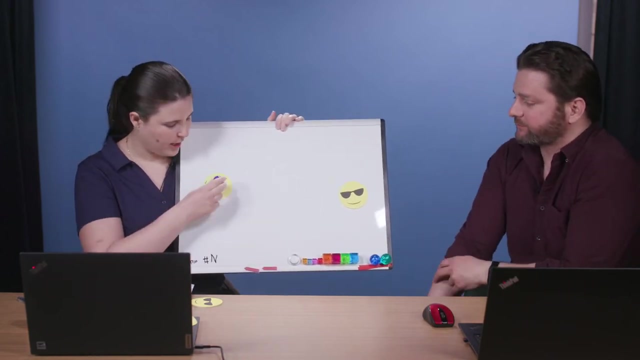 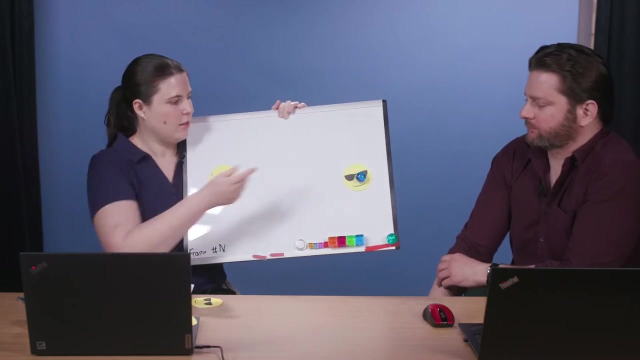 If you know what segmentation is. it could be a deep learning network. is some abstract features in your deep learning network that says, oh look, that's a person And I think it's approximate centroid is here, Right. So bear in mind, these are the real objects, So we know where they are. But this is you know, the computer doesn't really know that. Yeah, The computer doesn't see the smileys. What it does see is the detection. So for the rest of this demo we are going to be using these circular magnets for detections. So it's it's. it can be not very good, It can be pretty good, for now It's detected. 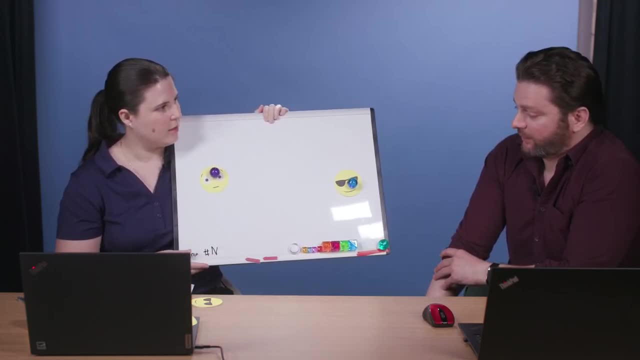 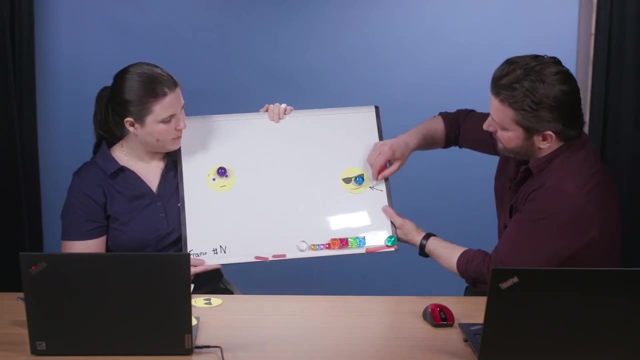 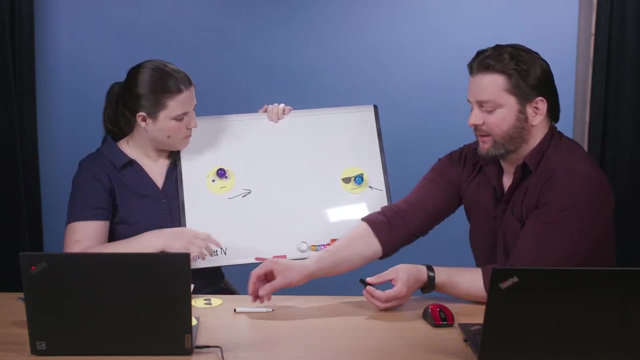 Two people in this frame. So what happens next? So this is frame N, And what we would have observed up until that point- I can do it on the right- is that maybe this one was moving with this kind of velocity here And then that that person- I guess we have to sign these ourselves- was moving like that. So the track, the tracking algorithm, then makes a prediction about where we expect them to be. 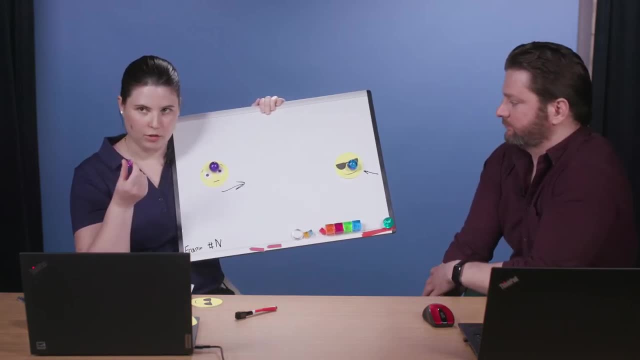 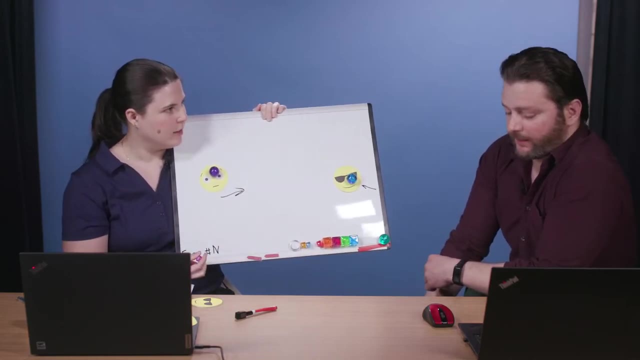 So I'm going to be using, for predictions, I'm going to be using these little squares And then for the tracks itself, I'm going to be using the big squares. So when I say a track, what is a track? Track is the computer's notion of the object persisting over time. 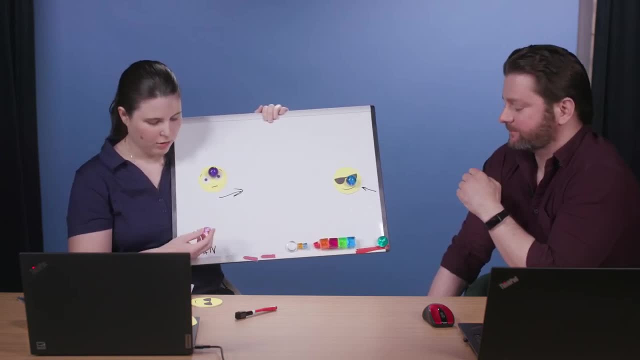 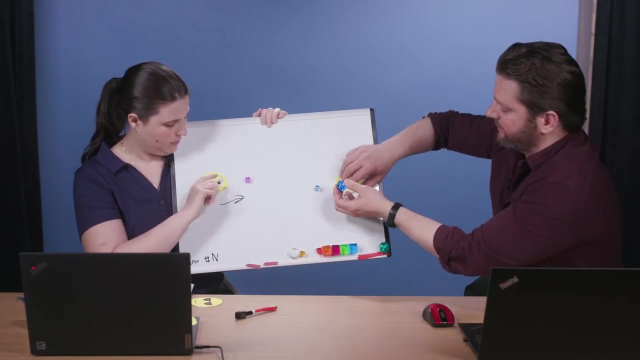 OK, so objects over time tracks. So if they make a prediction you've been moving, Your computer thinks you're probably going to keep moving, Right, Yes, Seems fair. OK, so it's made some predictions And now what's going to happen is these things are actually going to move somewhere, and maybe not exactly where we predicted. 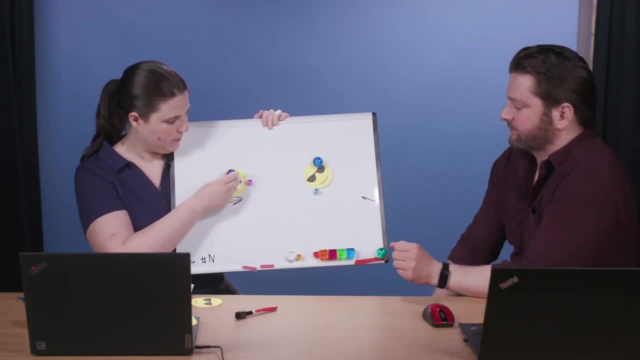 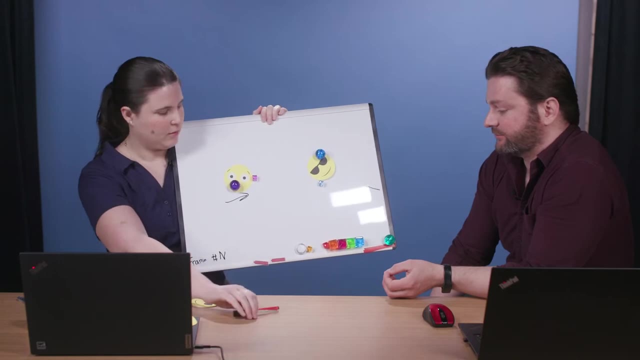 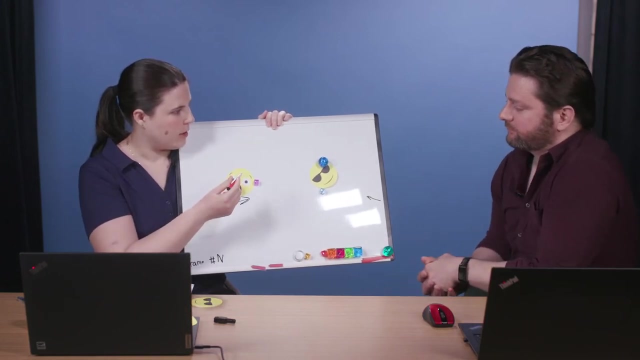 And then we detect them Again somewhere, maybe not exactly where they are. So the tracking algorithm also takes into account that there's uncertainty in both the detection and the estimate of where it will be. So that uncertainty is going to depend on a number of factors, right, Like it's going to depend on how good your detection is. 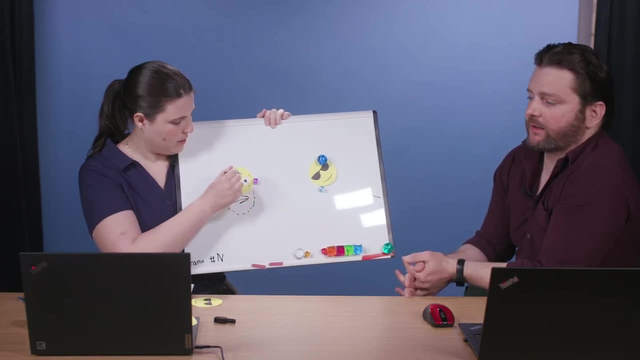 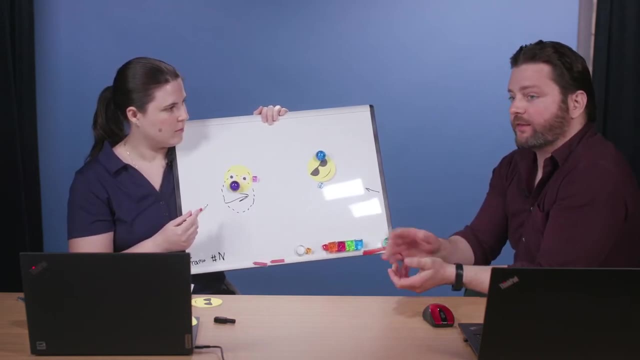 Yeah. So if you know you have like super high quality sensors, you might say, hey, I trust them As long as I get a detection from it. I think that's basically almost exactly where it is. Sometimes you might think my detector is really bad. 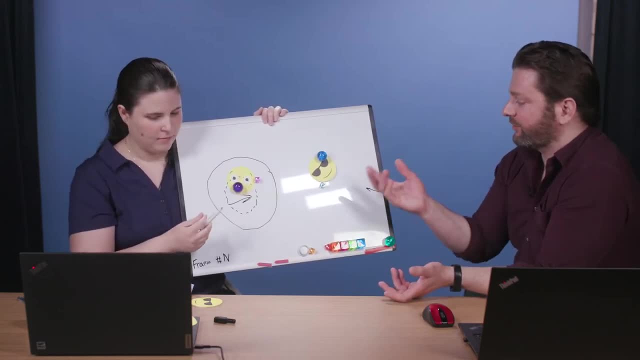 Right, Right now It's so noisy I don't know where the thing is. I'm going to trust my prediction, So that's the opposite. Yeah, So that would be a really bad detection. This would be a good detector and a really terrible prediction. 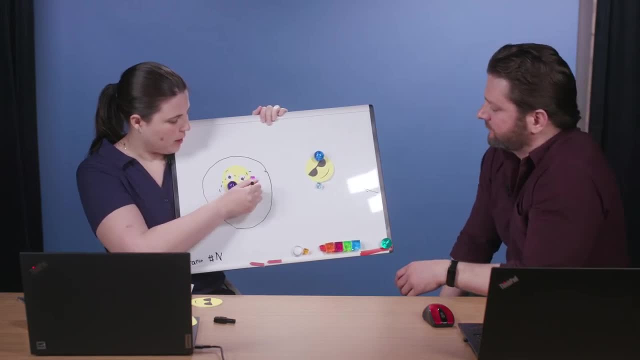 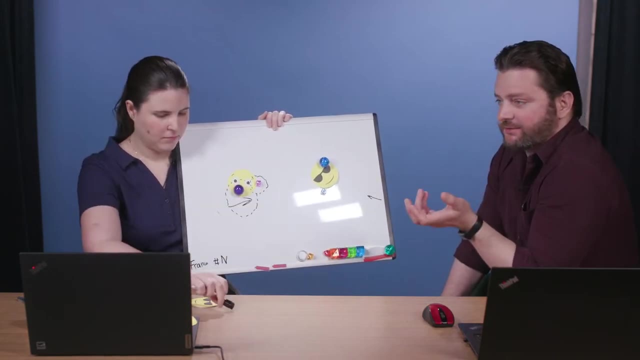 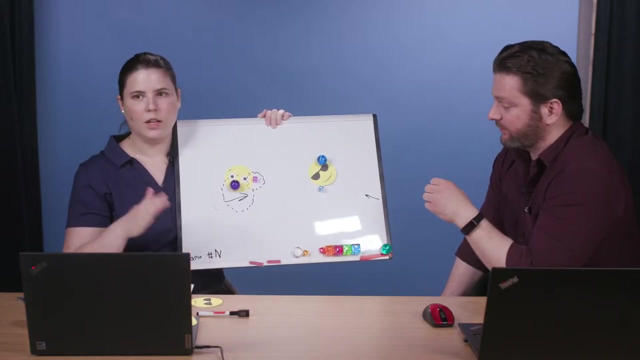 OK So, but if you have a really good prediction, it would be more like this, right, Yeah? So what it does is it takes both of those uncertainties into account And through the magic of some sort of state estimation. most of the time we use a Kalman filter, but you can use other ones, nonlinear estimators as well. 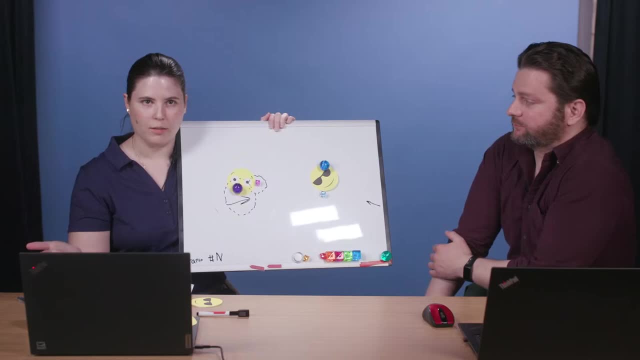 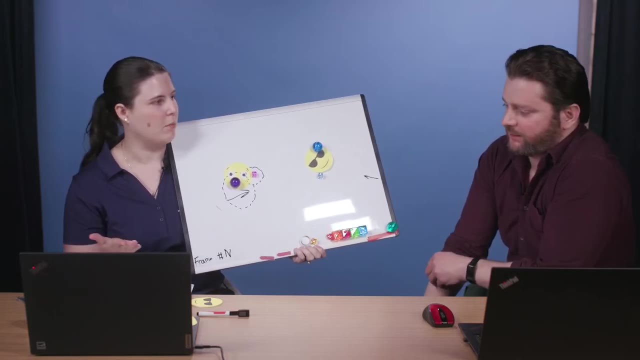 And you don't know the details, need to know the details of that. Yeah, So we don't know the details of the algorithm for this discussion. We're just saying we are using an algorithm. You can swap out your own algorithm. if it works best, We will be using Kalman filter here. 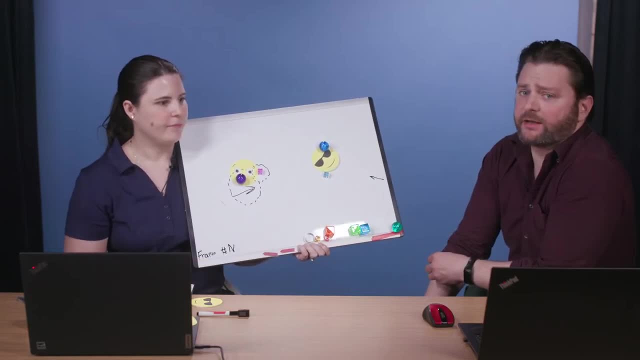 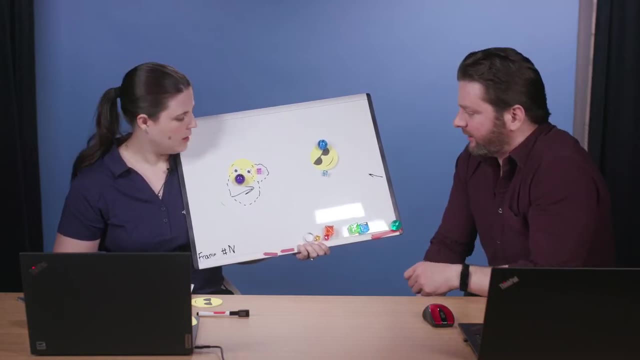 Yeah, And you'll learn a little bit more about that in the course. MATLAB makes it pretty easy to do tracking even without being an expert in state estimation, but it helps to know a little bit about it. Yeah, All right So. 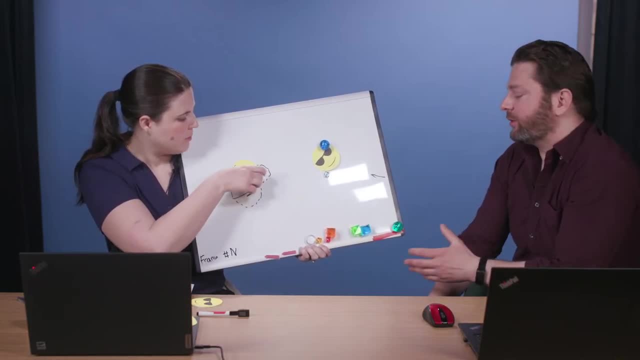 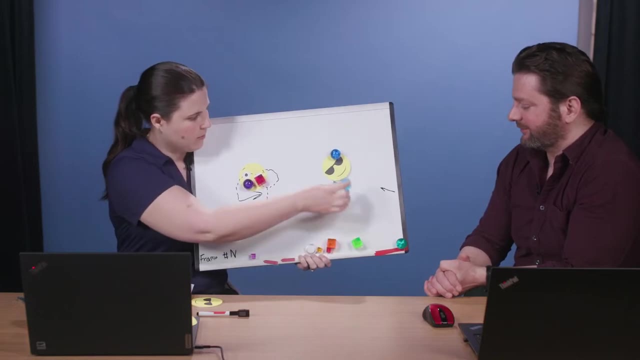 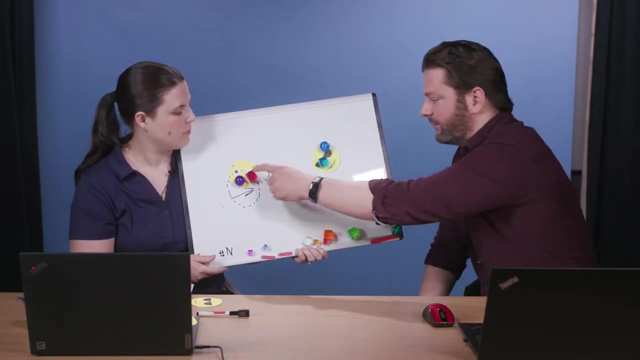 You have a prediction, You have a detection, Your track should be somewhere in the middle. Yeah, I mean you could think of it like that, roughly speaking, some sort of weighted average of the two, based on, you know, Your various assumed uncertainties. So now this is where we believe these objects are. This is the computer believes that I'm here and Megan is there. 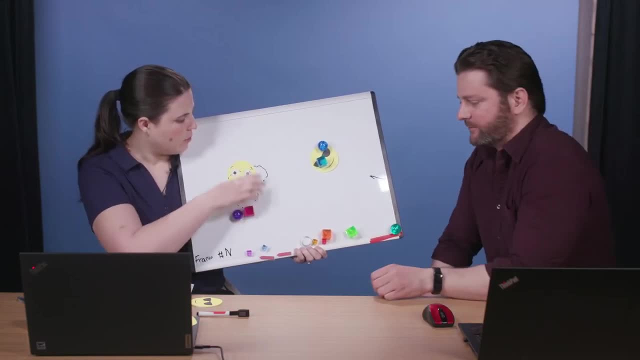 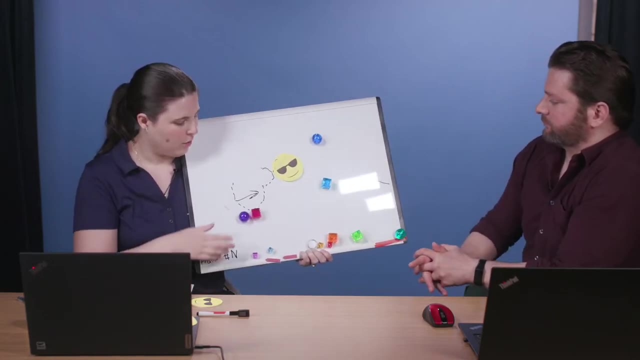 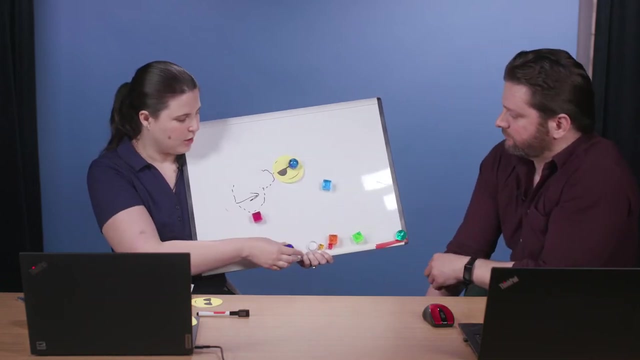 Okay, And then this process just repeats over and over again. right, All right. So what happens if something? we stood in front of each other a little bit earlier and the detection was lost? what happens then to these detections? So I think one person gets detected, the other person's hidden. we lost the detection. What happens to the tracks then? 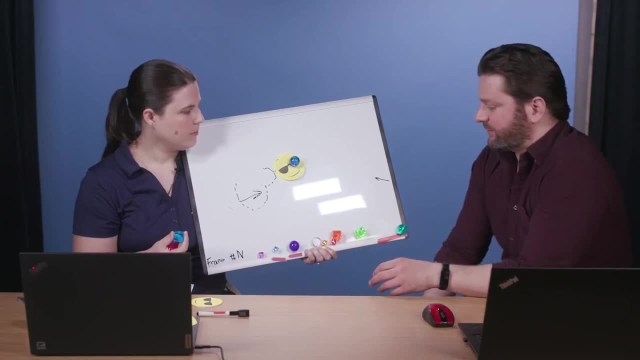 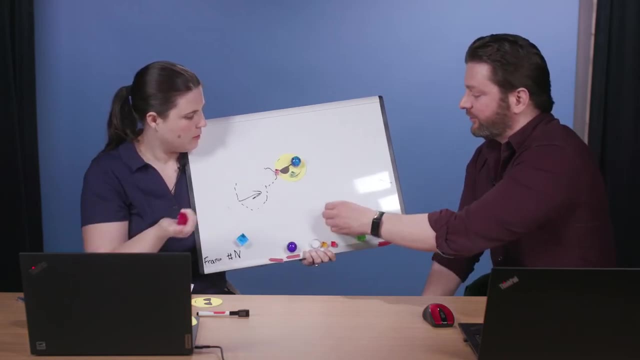 Yeah, So well, we'll just leave out the estimation part, but there would have been estimated locations. There's only one detection. That's fine, because the tracks remember. the tracks would always: where did I, which one was I again? 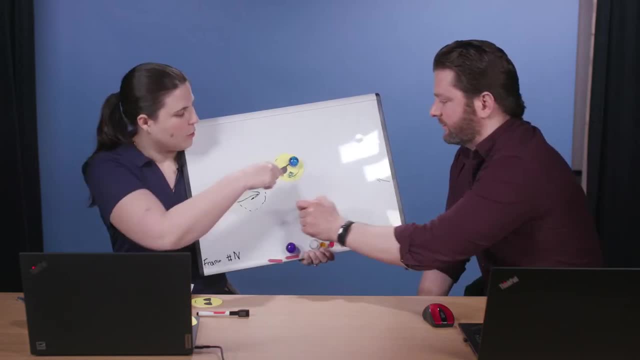 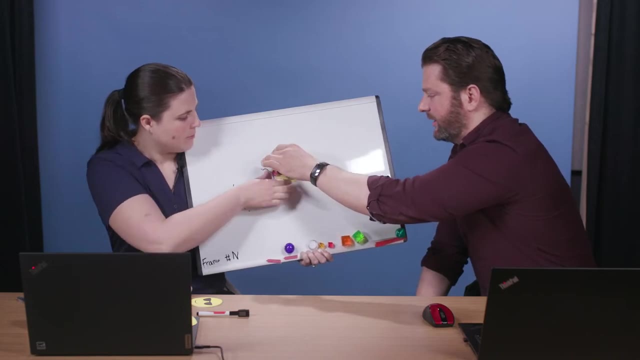 You were This track, I think, right. Yeah, You were the blue cool dude, Okay, But both of the tracks would have been updated to be basically here, right? So, even though- and this is getting a little crowded- even though it's only detecting me, or well, it doesn't know what it's detecting, right, It's a detection. 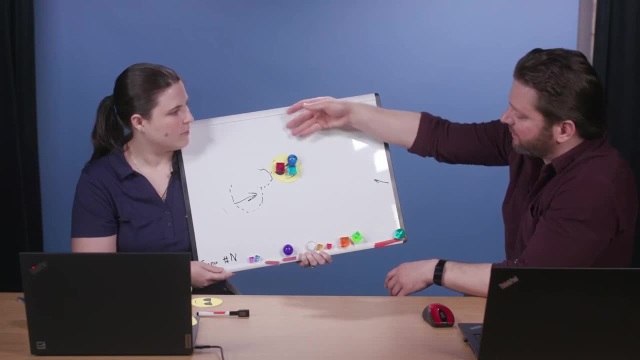 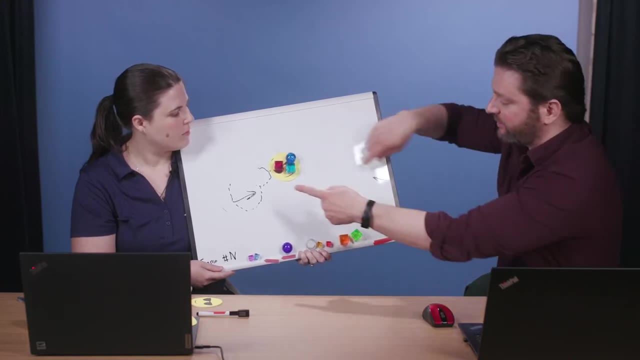 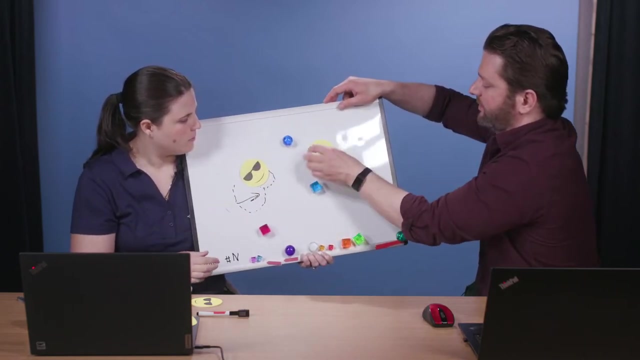 Mm-hmm, And so this detection would get assigned to this track. blah, blah, blah. Her track still exists, even though it can't see her Mm-hmm, And you'll see this when we demo this in a moment. That's a very important concept, because then, as we keep moving, all right, may I go this way, And maybe she's over here now And I get detected somewhere and somewhere. 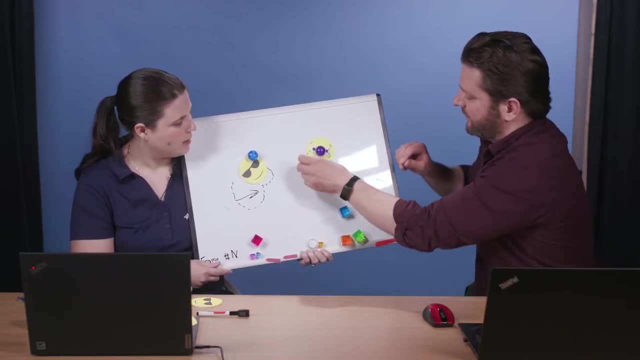 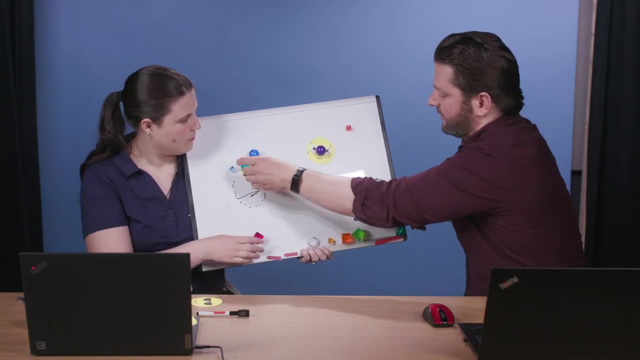 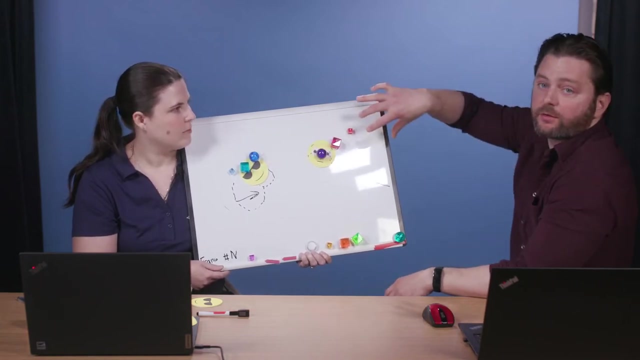 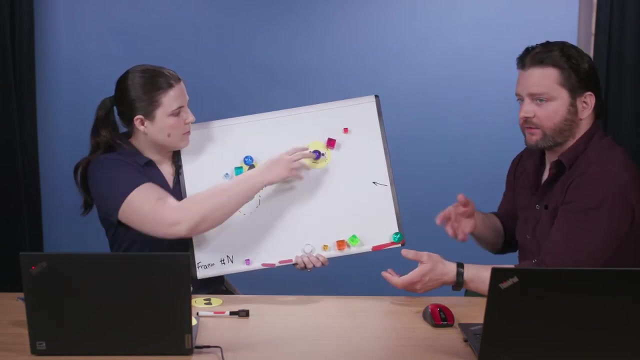 It's picked me up again, I've been redetected And maybe you know, maybe it even estimated. she went further and estimated And estimated I went over there And so then we get updated yet again And that's where it believes we are. But these tracks are persistent over time. Now there are parameters you set to say like hey, if she disappears or I disappear for long enough, we'll actually delete the track out of our system. 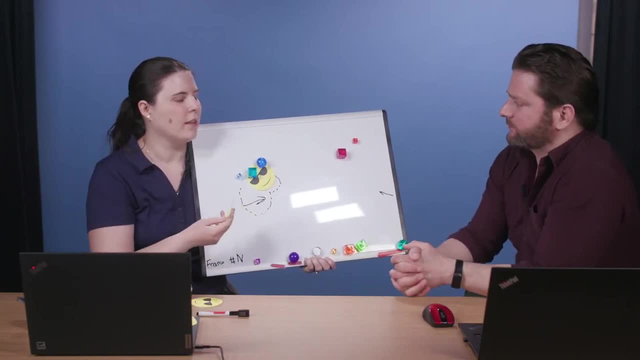 So if I go like-- And that's a parameter you set right- So if I go spend like 10 times without a detection, it figures Megan's gone. She's no longer in the video. Yeah, That'd be the simplest way to do it. 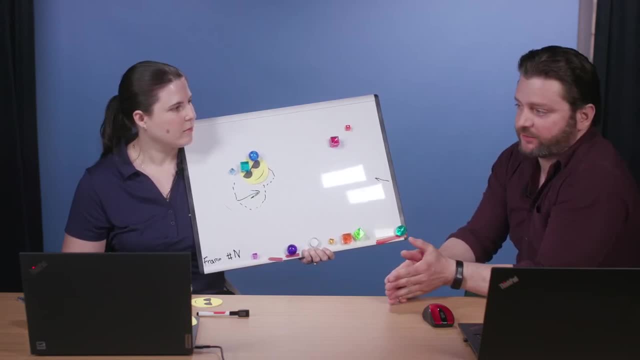 Yeah, The simplest way to do it is just say, hey, if I don't see that object for a certain span of time, just assume it's gone forever And you can remake a new track if you see it again. but you'll assume it's gone. 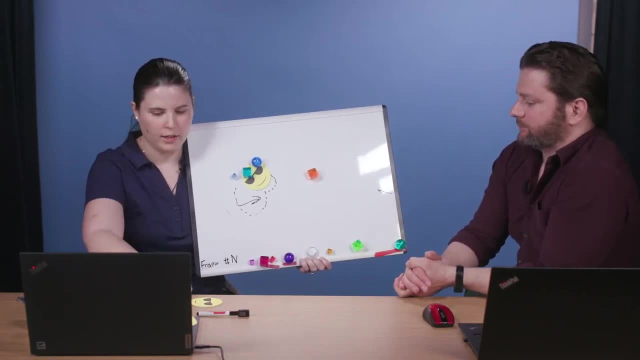 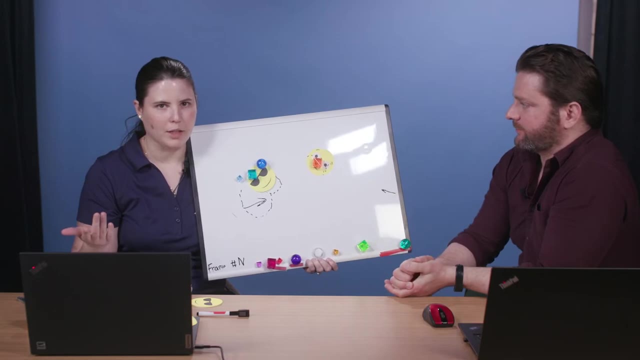 But then if I'm gone for so long, it deletes my track. if I reappeared, I get a new track. Yeah, You'd be a new track at that point. Okay, But that has to- you can set that to be as long as you like. 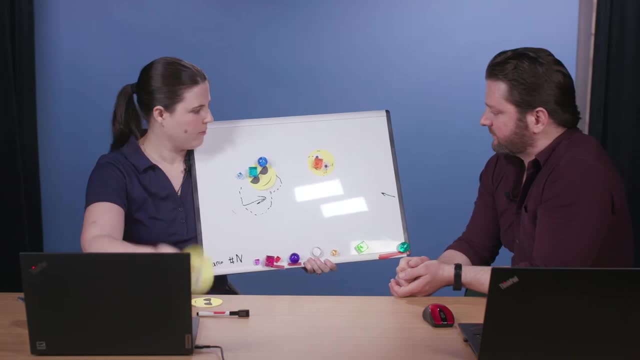 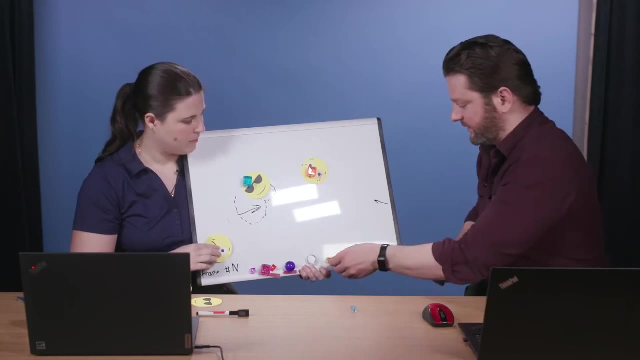 Mm-hmm. All right, Now what if- where's our third face? So say, we're both being reliably tracked at this point, And then another- well, we get a detection, not this one New detection, We get some detection over here. 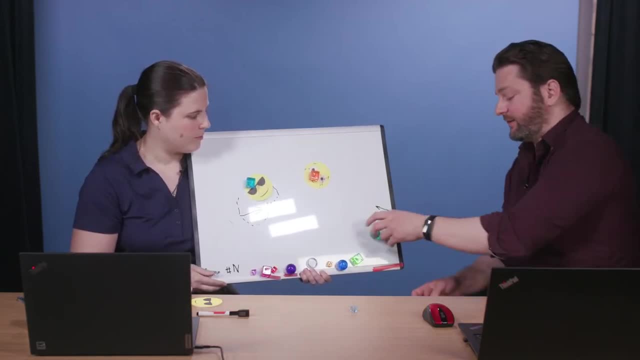 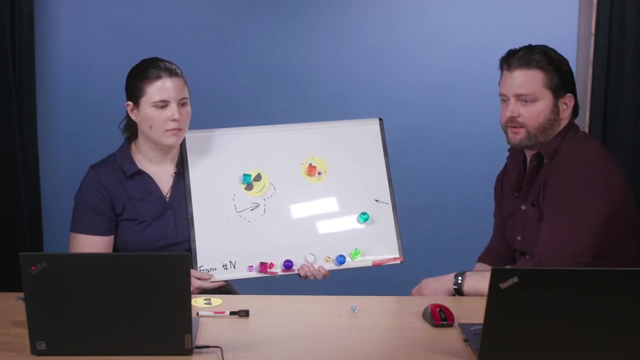 Yeah, Okay, And that may be coming from something-. well, let's say, we just get a detection and there's nothing actually there. So you know you don't create a new track right away. So that's another thing that goes into these algorithms which you know will- maybe I should bring up the diagram again. 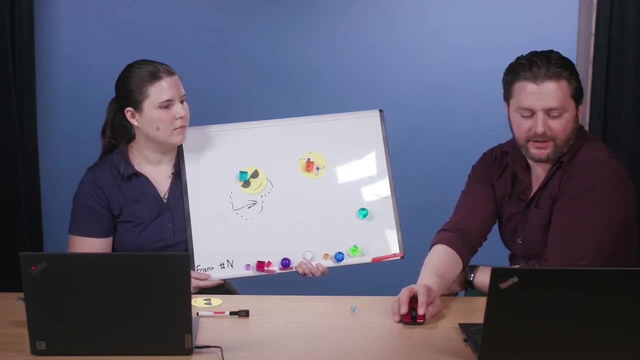 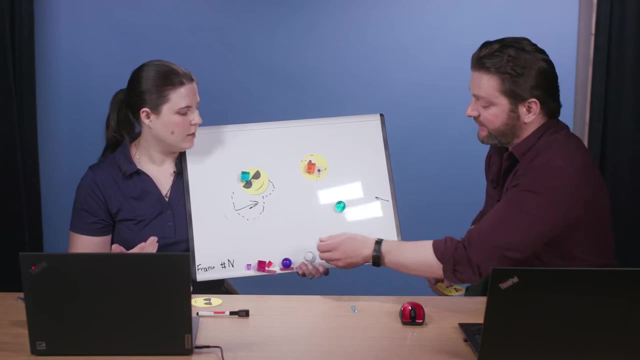 Basically, you set a lot of things in the assignment and update and prediction steps. that makes sure that this has to be there, and maybe two, three, maybe- Yeah, A certain number of times and then you say, oh, that's an object. 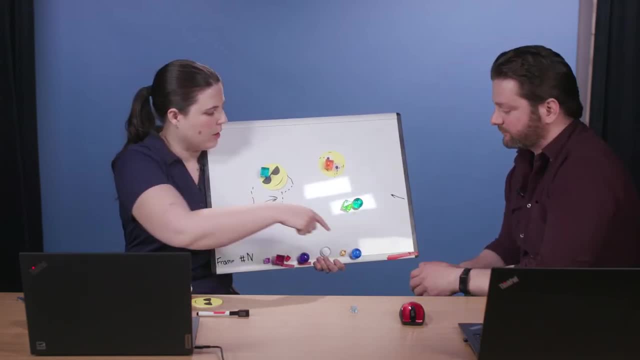 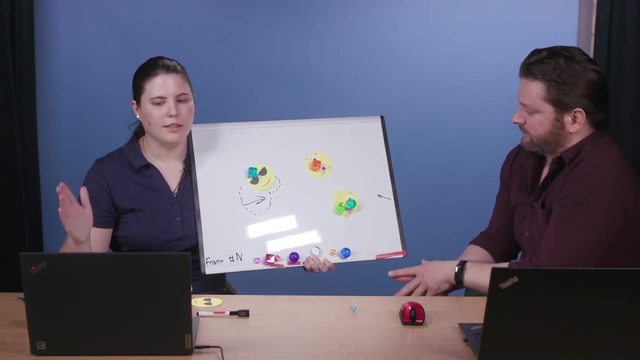 That's another track, Like I'm confident enough that there's really- if you want to put a goofy person there, Well, assuming there was something there- yes, If you do it long enough, your algorithm becomes confident, Like that's not noise, That's not something weird happening, That's a real object there. 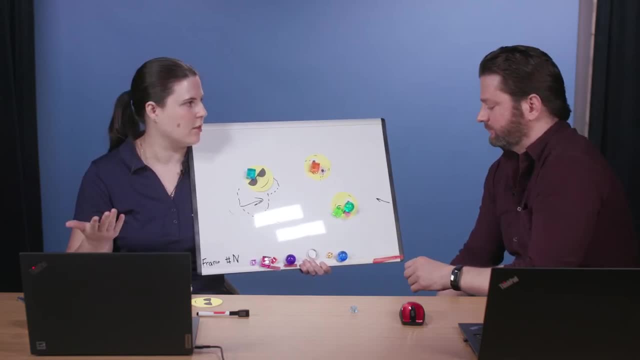 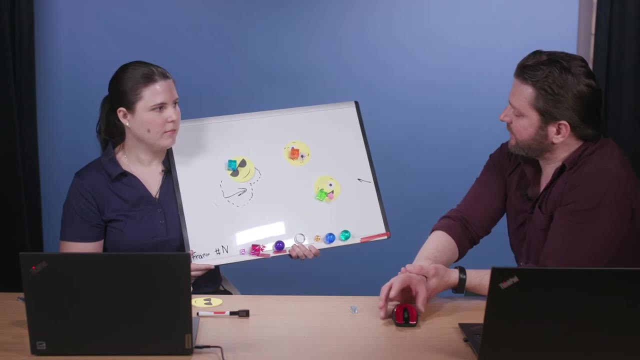 And then at that point, after a set number of detections that kind of make sense, it gets assigned its own track. So now everybody is tracked And I guess, as you've sort of seen and we've been hand waving through the assignment process is-. 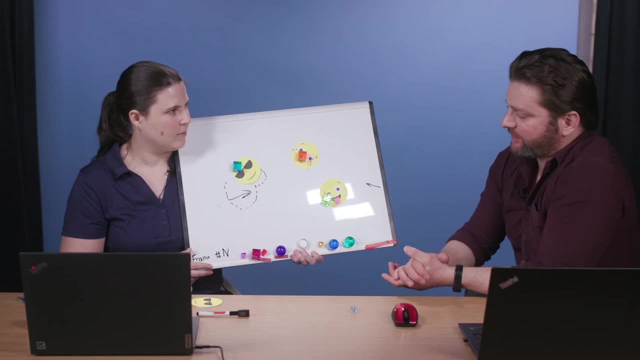 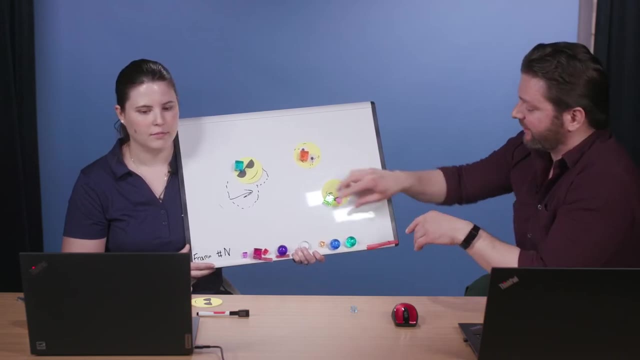 Well, it's also done primarily for you in MATLAB, but it's more or less done based spatially on you know which detections are closest to which existing tracks, And so you know. that's how you'd say: well, if I get a detection way over here, that's either nothing or it will be a new track at some point, right. 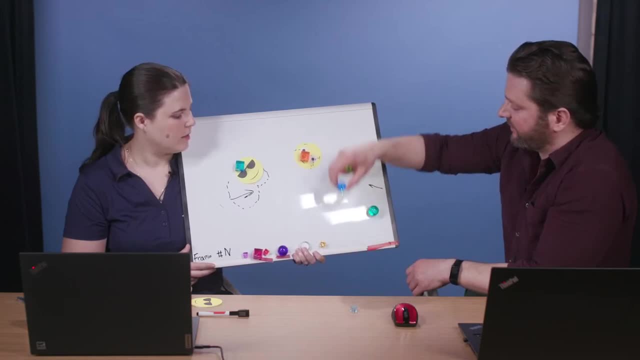 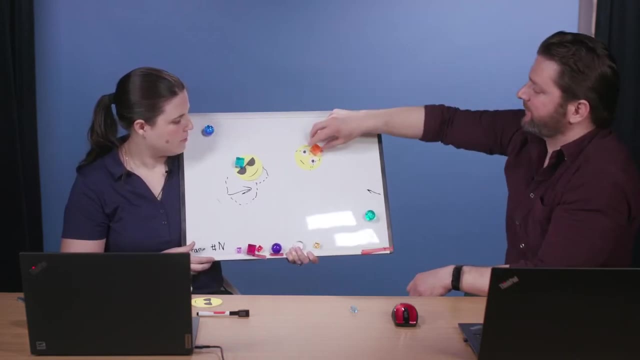 It's not one of these two, Yeah, But then if I detect something here, well, I'd say that's close enough to be Matt, Yeah, But if I was really over here, actually I wouldn't necessarily say that, Yeah. 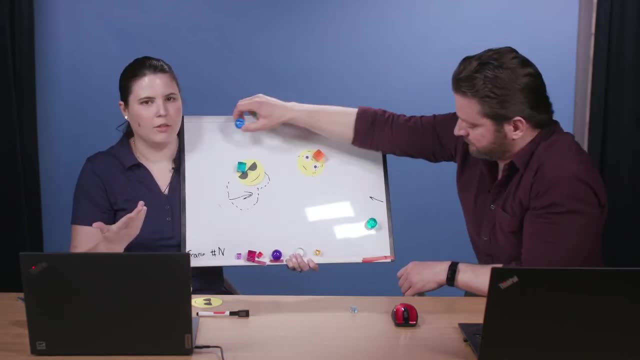 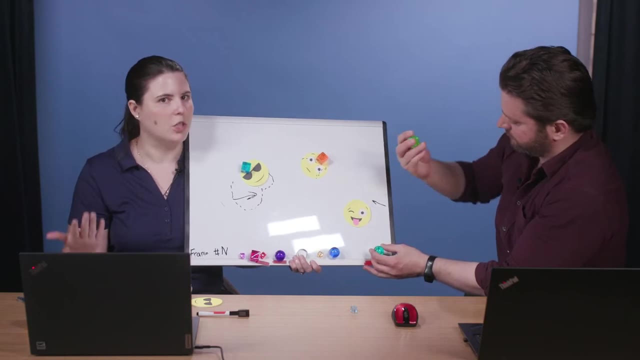 We've never assigned this detection to this track because it doesn't make sense with what we predicted. It doesn't make sense with where the track is: It's too far away. So your algorithm gets pretty smart about knowing which detections go with which tracks based on the predictions. 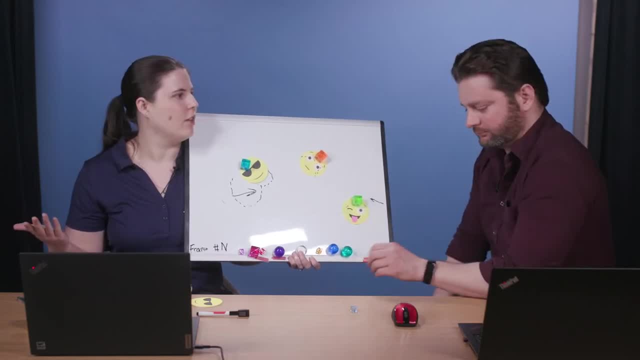 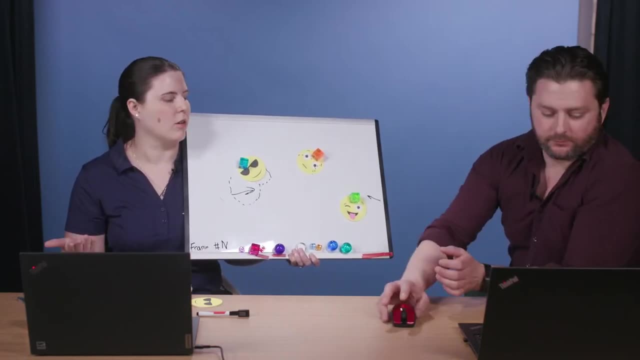 And again this will be discussed in- you know much more detail And you get to actually tweak some of these parameters and move them around. see what it does in the course, which is part of the Computer Vision for Engineering Science specialization. 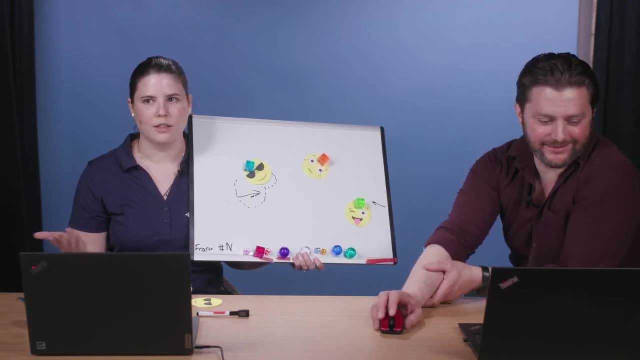 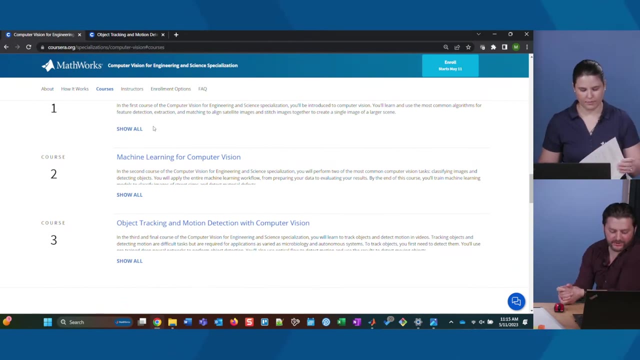 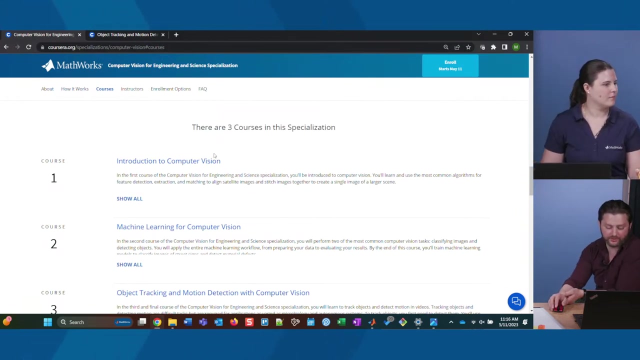 It's part of the specialization. yes, And specifically it is the-. Yeah, Well, I'll just scroll down to it. It is the third course: Object Tracking and Motion Detection with Computer Vision. If you are not already familiar with the first two course topics, or even if you are, there's probably still some interesting stuff in those as well. 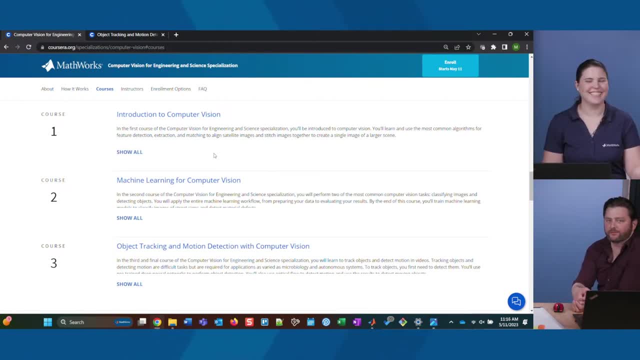 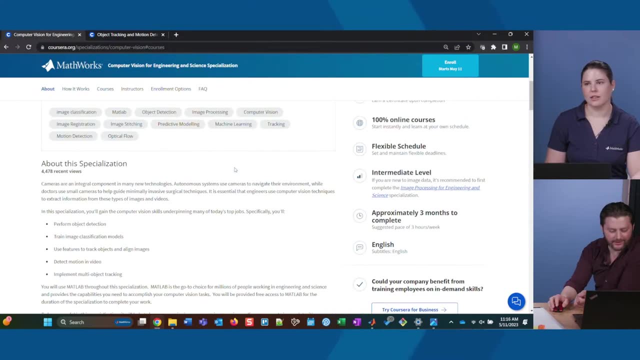 I mean- And while I'm plugging us, if you don't even-if you feel like man, it's been forever since I've done image processing, or I've never done image processing. we also have a specialization on image processing which I don't know. 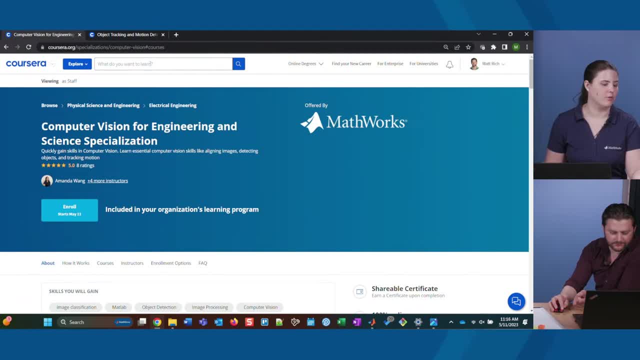 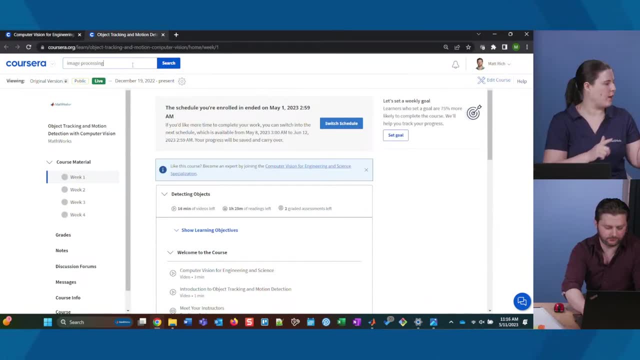 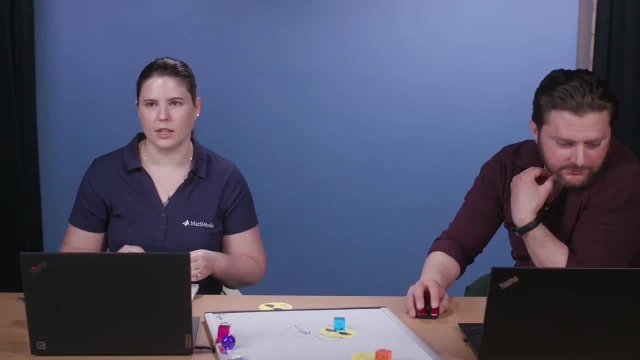 Yeah, So image processing is something that we're talking about can just be image processing algorithms For something like the Smiley Face application. image processing would be really good at finding circles, at finding the difference between the sunglasses person and the person, because just based on intensity, colors, all that fun stuff. 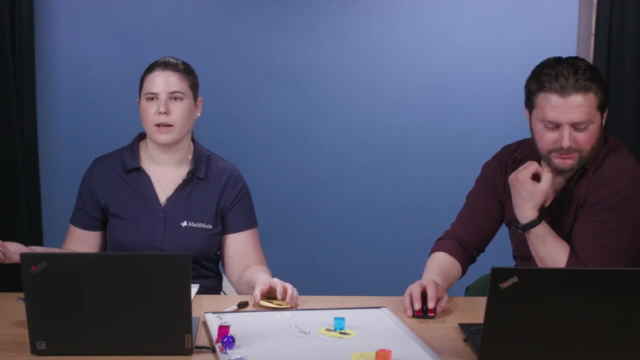 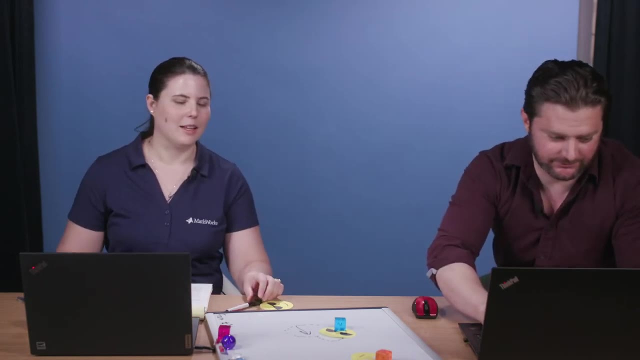 So if you want to look at it more from an image processing perspective, you can find a lot of that good stuff in Image Processing for Engineering and Science. That's what it's called. Yeah, Yeah, And I think that's a really good example of how you can support that course board. 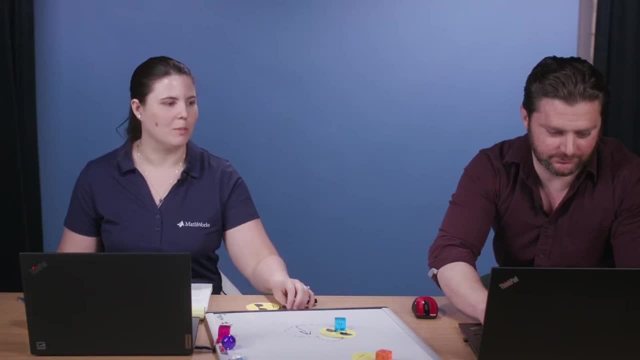 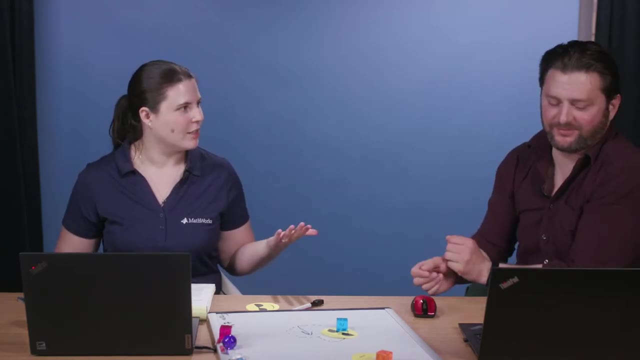 So if you go there, you'll get to say hi to me in the discussion boards, but it also means that I've typed that title a hundred bazillion times. So we talked about the code that you'll get to use in the course. 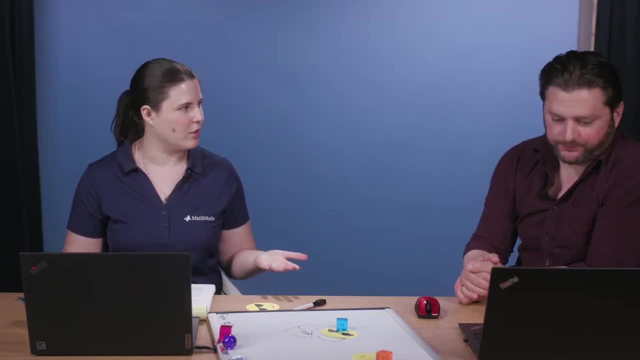 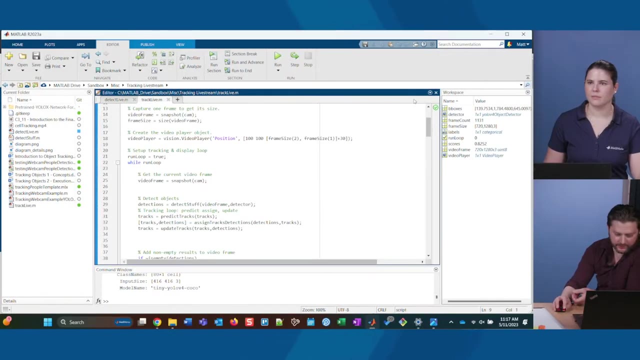 What? can-can we see an example of that? Can we see how all these fun functions work in reality? Yeah, So, code-wise it's actually pretty simple. Let me just make this larger. Maybe Can you just control plus. Is that what does it? 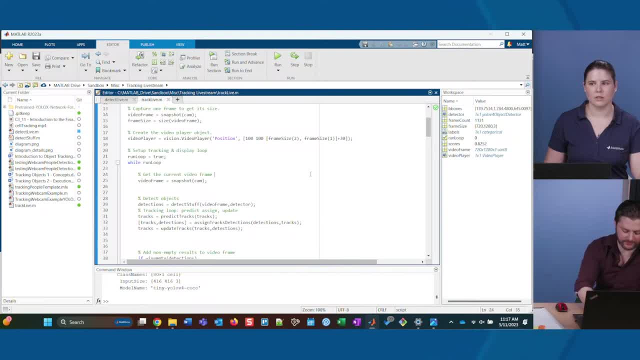 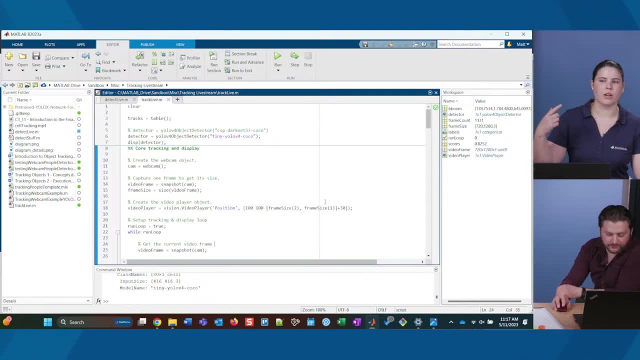 Yeah, That'll zoom in. Oh, Doesn't for me. Anyway, you see that for each frame, that's the run loop. we're running through each frame, in this case, of the webcam in the course. Yes, You'll be doing it from a recorded video. 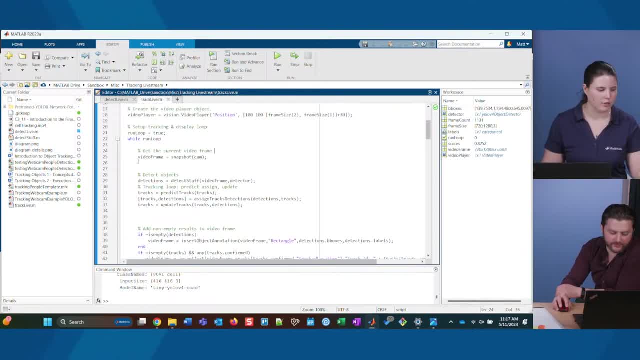 So, yeah, We're getting frame information here, That's. you know, whatever, This is the algorithm you just saw. This is this thing right With these. four blocks are basically done with these four lines of code here. So this is an example. 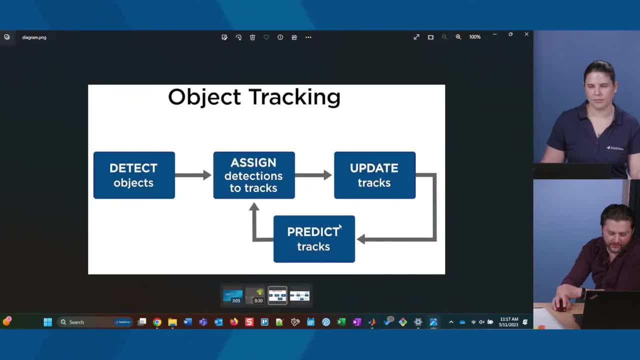 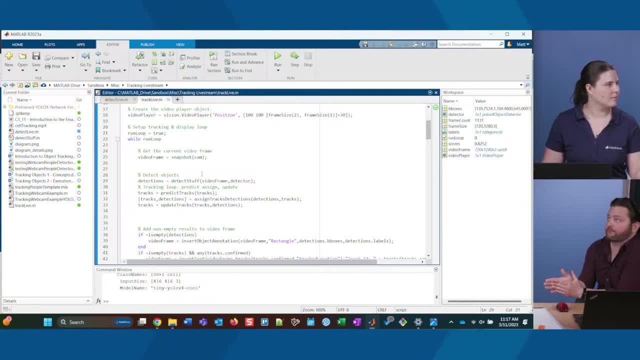 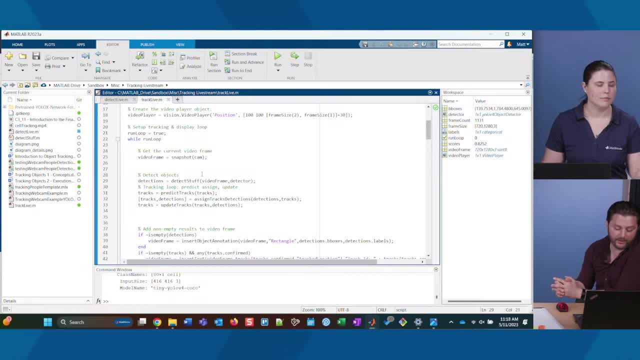 You'll learn how to use the same pre-trained deep learning network we're using right now to detect objects, Which is YOLO for all of you. I'm curious. Yes, It is. yes, You only look once. That's awful. 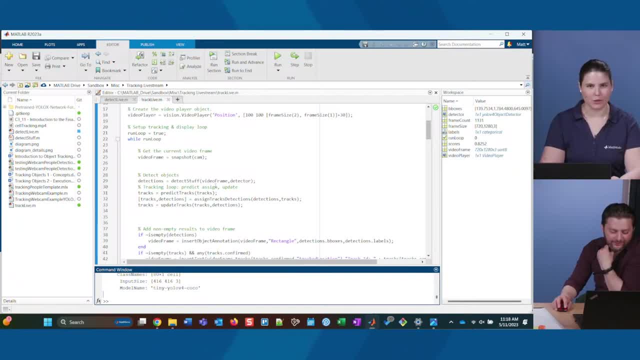 I didn't name it. I know Sorry to the creators of YOLO. We love your work, I'm not Sorry, But anyway. Predictor. Then you have a prediction function which, again, I'm not going to go into all the details of it. 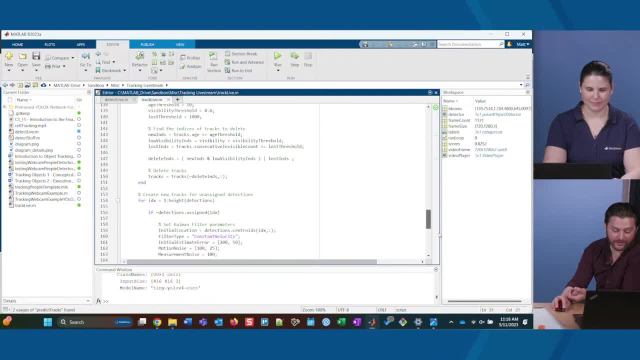 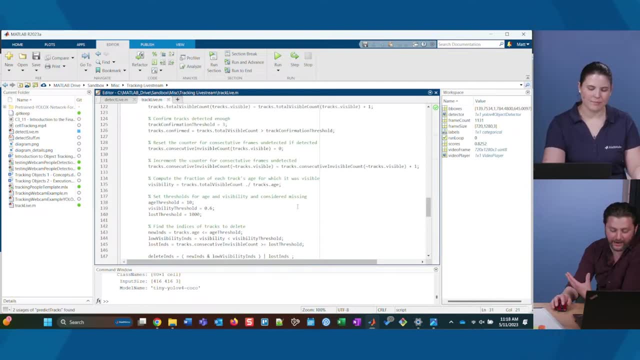 But these three functions. if I scroll down there is quite a bit to them, But we go through all of this, basically every line of it in the course, and explain how, what you're doing, why you would do it, And you'll know how to tweak these parameters. 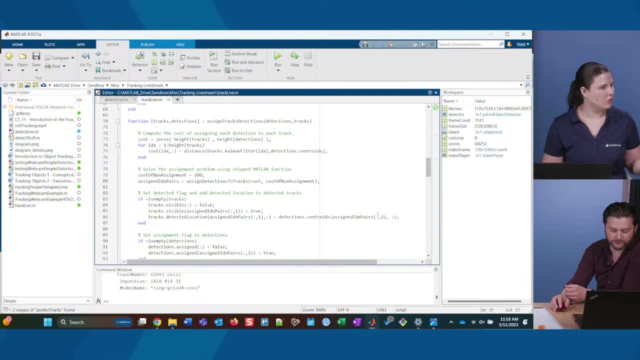 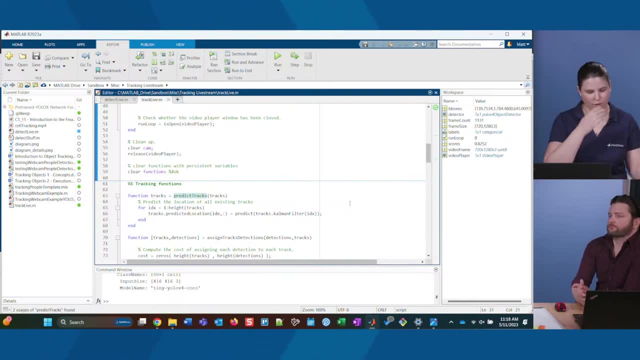 when you get there. And we did have a question from the chat about who is this aimed at, this demonstration and this course? Is it for basic learners? It asks if it's for kids. I think of myself as a child at heart. 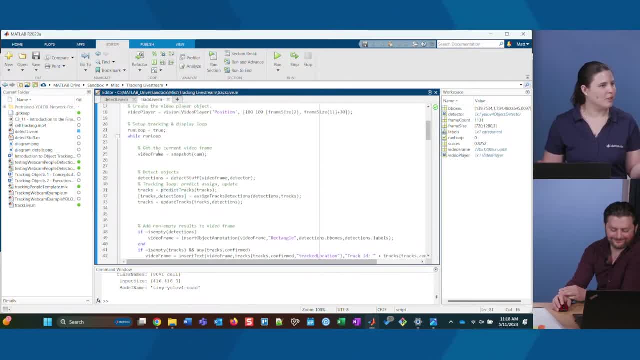 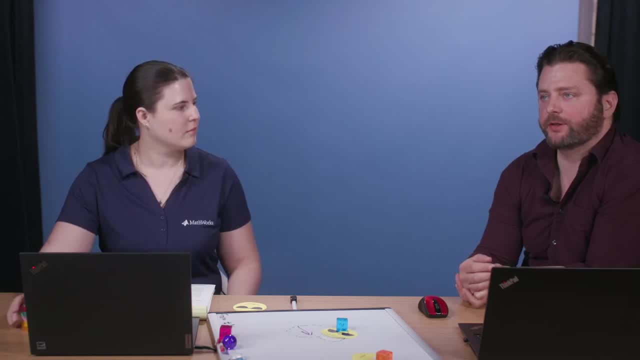 so that might explain the colorful magnets. But who should take this course? The course material itself is going to be a little bit more geared towards your college level working professionals. You don't have to be. We get people in high school. So if you want to take it and you're younger, 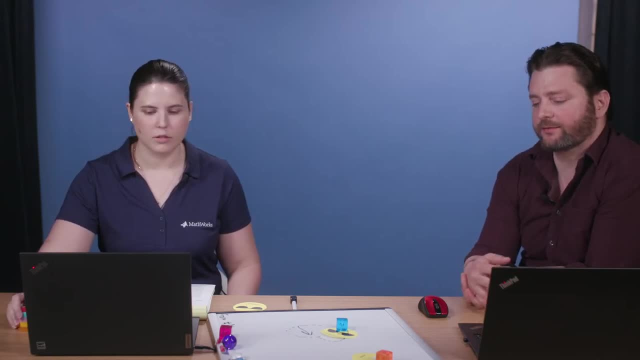 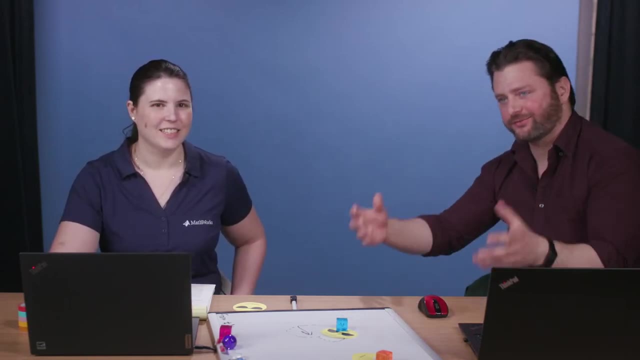 that's perfectly fine. It's a little ambitious though, But the course material, just to be clear, and nothing against our demo. I thought it was great, But the course isn't like this demo. The course is a little more polished and professional. 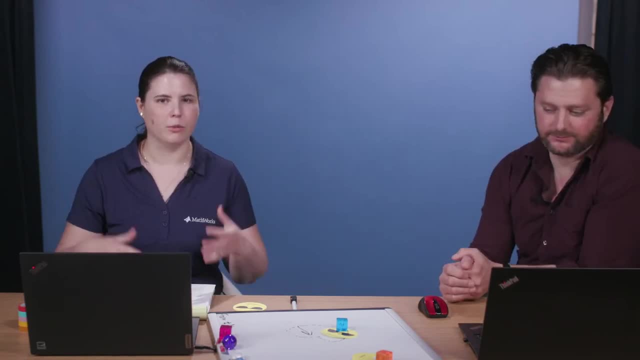 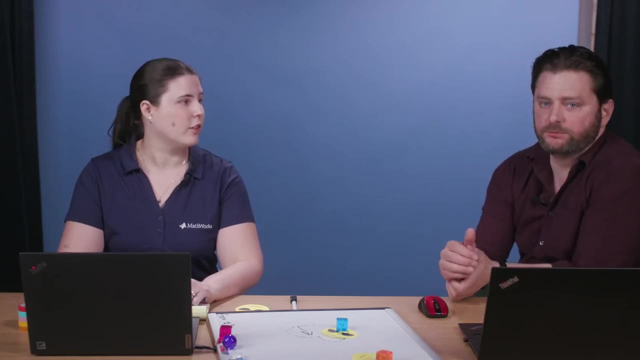 It's just we thought it would be a little boring to bring you to a live event to then show you a bunch of videos. So that's where the smiley faces came in. You'll get to do actual, real world examples like tracking pedestrians, tracking moving vehicles. 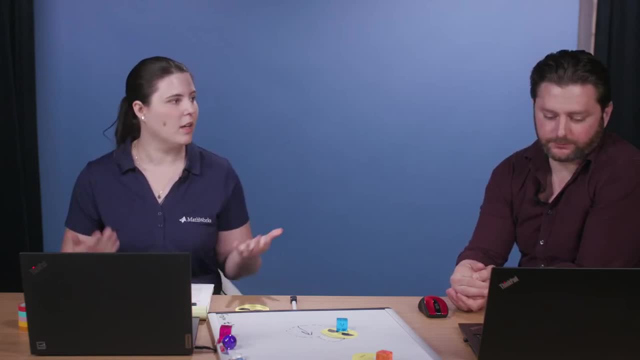 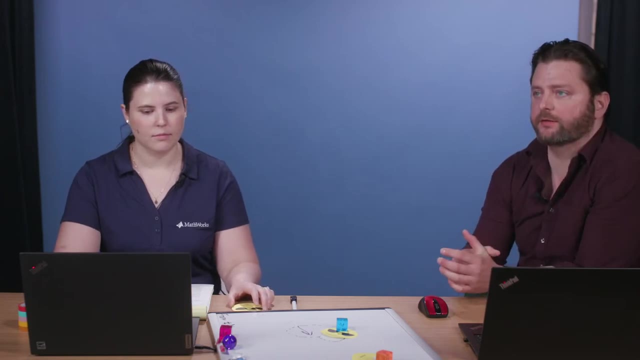 e-sales. The examples in the course are much more applied to different fields. Yeah, I forgot to mention that you do the e-sales as I showed, And I don't have a video of it right now pulled up, But the final project for the course. 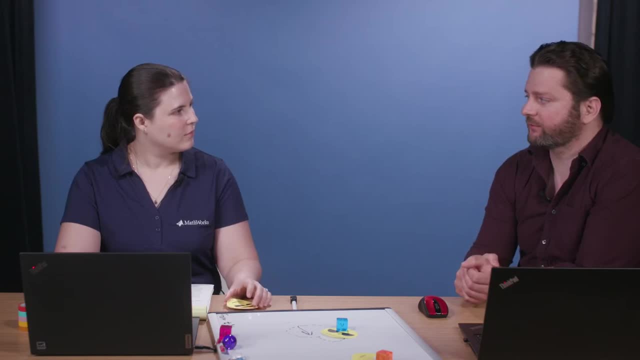 is you actually count the cars moving in different directions on the road outside of MathWorks Canvas, which is one of the applications where you need tracking, Because if you detect it well, you detect a car every frame And you'd count several thousand cars every second. 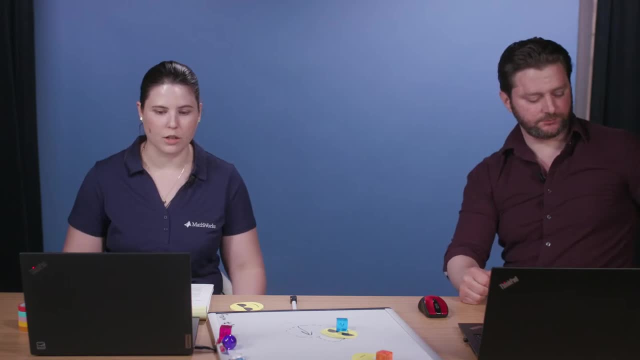 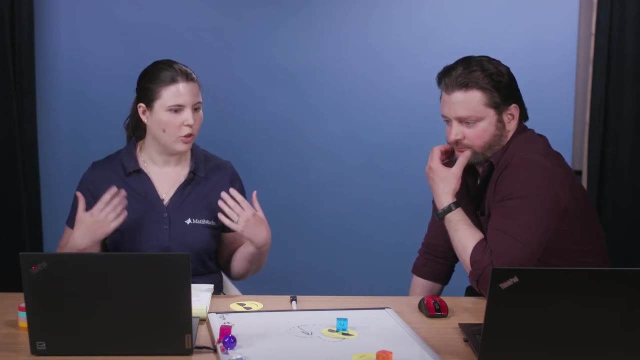 So that wouldn't be good. We have a really great question here about speaking of image processing, But how do you handle the light effect when an object's moving, Like things look different in different frames based on the lighting around it, So that can really mess with your detection algorithm. 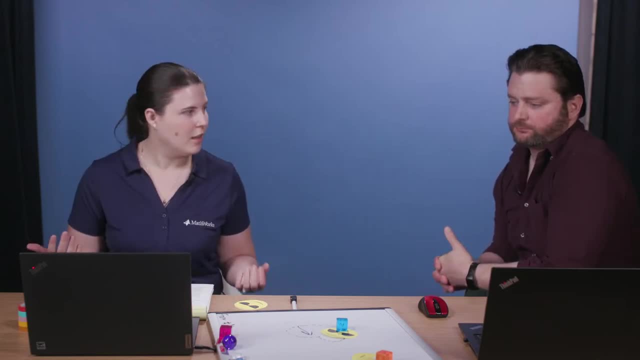 depending on how well-trained it is and how prepared it is for the lighting. There's a couple of things you can do. You can do image processing to kind of clean that up. But that's one of the nice things about tracking is that if there's a flaw in your detection algorithm, 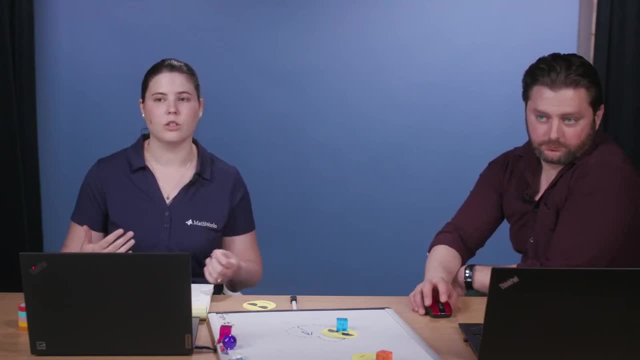 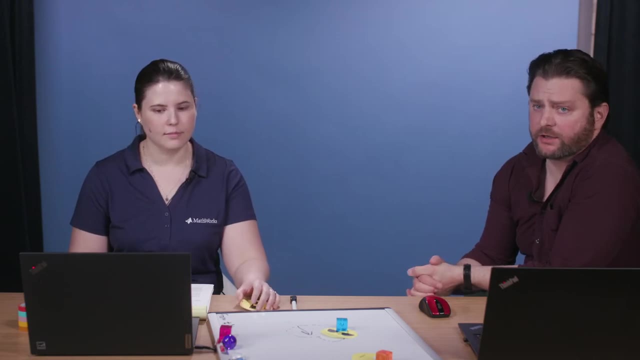 and you lose something. the track should still be able to handle that and should still be able to pick it up again when the detector goes, like there it is. That is one of the main things about tracking, which we're not really showcasing here much because, again, we have a nice set. 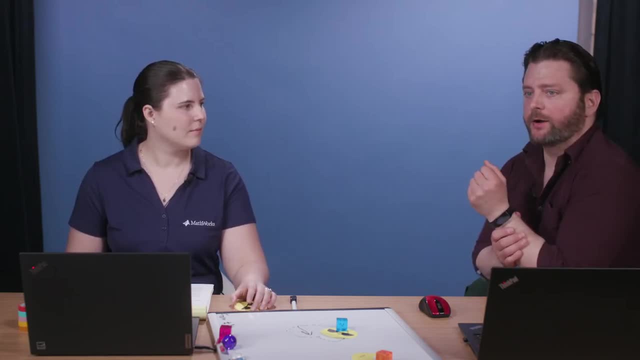 up. we're in a studio, we're five feet away from the camera and our detector is a neural network, So we're overdoing it as far as that is concerned. I mean, we won't have as many problems with lighting in that sense. 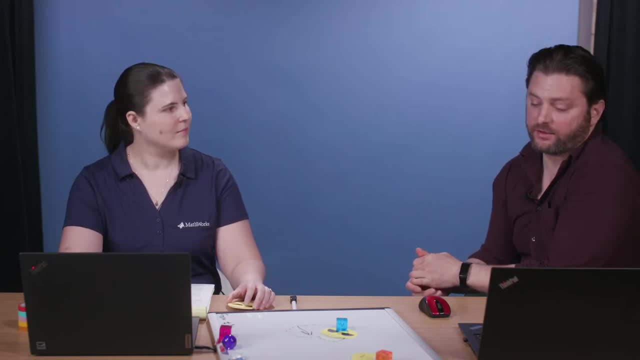 Yeah, I mean, if you were using- basically just if you were using- image processing, lighting is going to be much more of a problem. It will still be a problem if you're using deep learning, But you can kind of well, You can- find ways to prepare your algorithm. 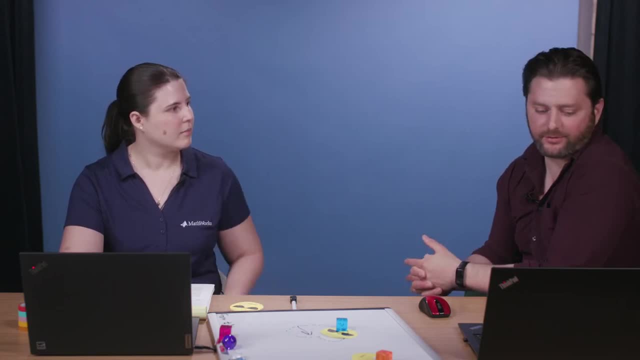 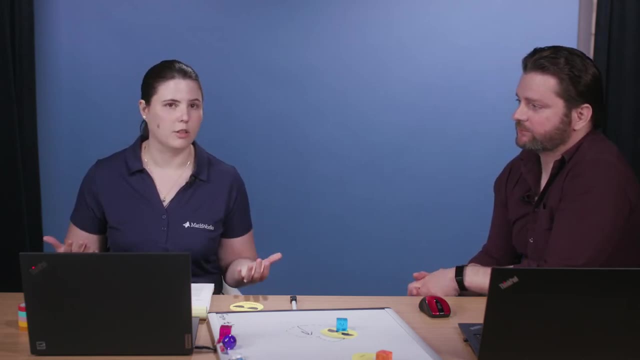 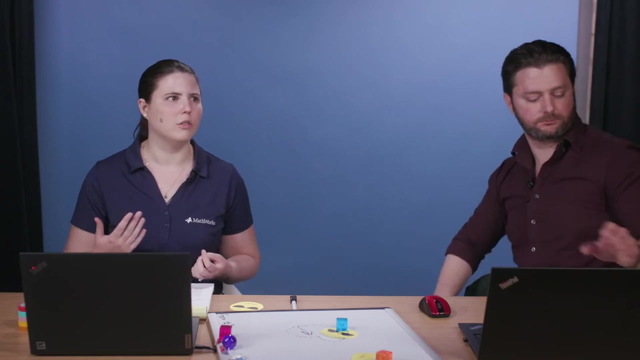 You can train that, You can use the. But we do have in terms of more traditional machine learning. in this computer vision specialization there is a course on machine learning for computer vision applications And that includes training models to tell when the lighting is a little bit different. 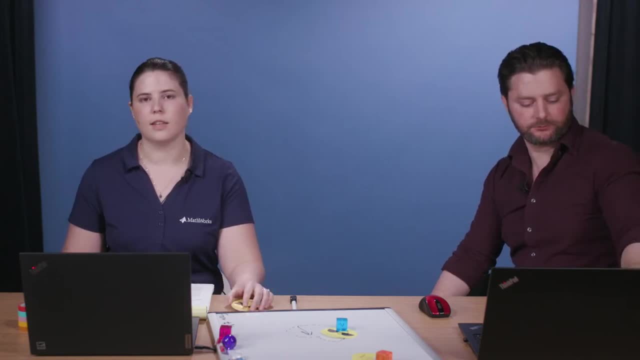 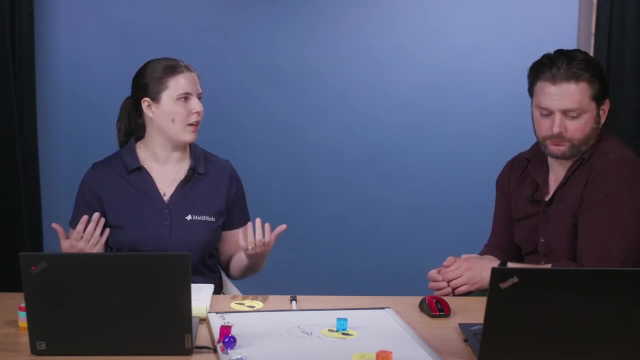 and still be able to pick up what you're seeing. There's a great example for roadside safety of even when it's sunny in some pictures and cloudy in others, you should still be able to detect roadside conditions Like I think we use snow if the road is covered in snow or not. 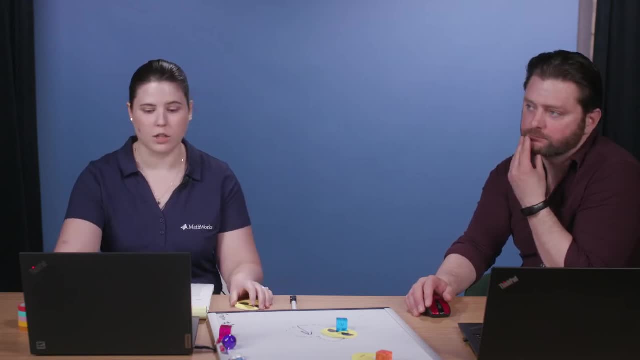 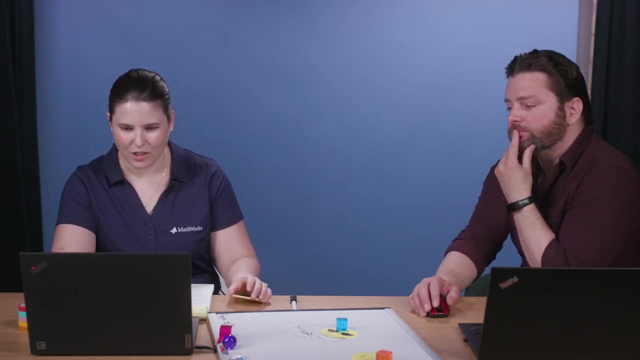 And so we do talk about that in the course. But it's a great question, All right, Hi, I need to track the speed of people who are moving in a video. The output of the program should be like a rectangle covering the detected human. 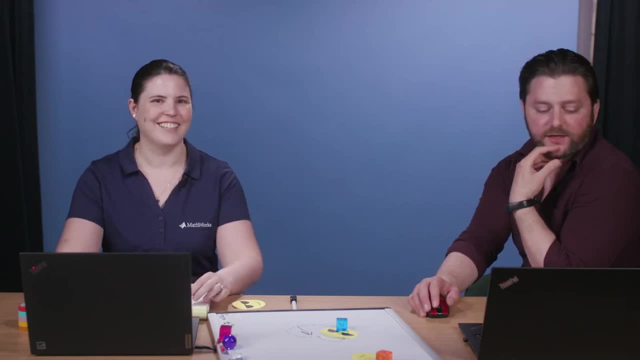 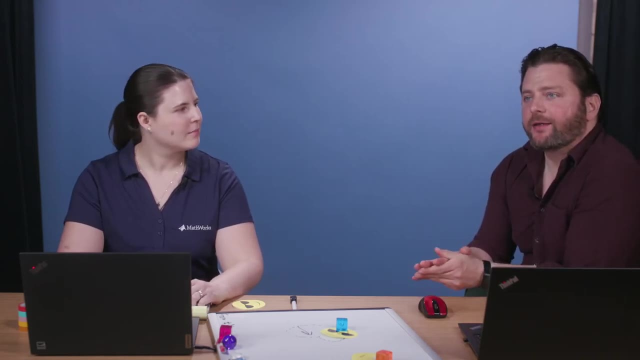 and annotating the speed of the person detected. That's actually very easy to do with this. I'm not going to do it in real time because I probably, you know, Typing in front of people is a dangerous thing to do. But actually, yeah, the speed and if you do our project. 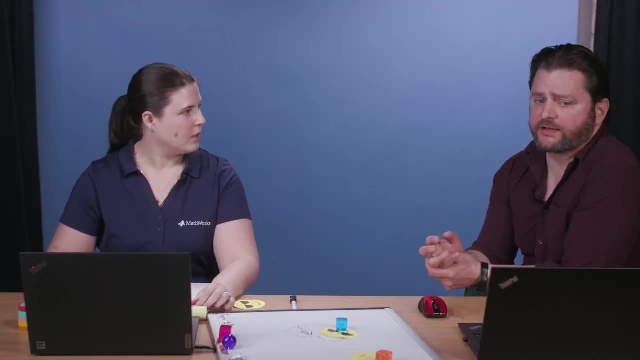 it's not even just the project, But part of the project is actually getting the velocity of the cars to tell if they're moving east or westbound. As far as displaying that, there's a function that you could easily insert- object annotation or something- and you could just display the observed speed. 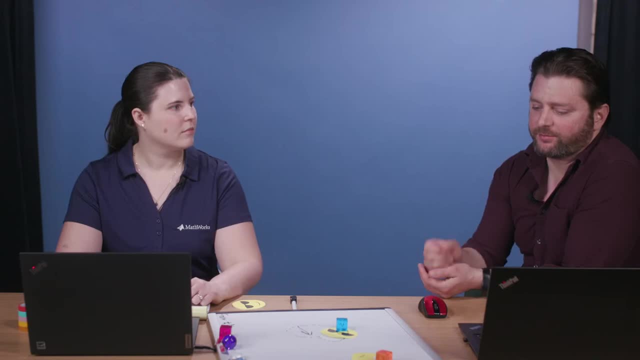 Now there would be some nuance there- that because you're using a camera, you're not getting the mile per hour speed. You'd have to have some additional calculations to convert your pixel velocity into something. If you're using a camera, you'd have to have some additional. 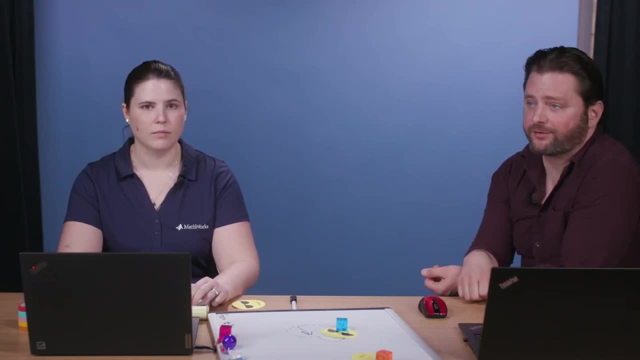 calculations to convert your pixel velocity into something else, if you really wanted to do that. But yeah, in that course, you put bounding boxes on things, you label them, you can annotate them however you like and you absolutely are required to calculate the speed. 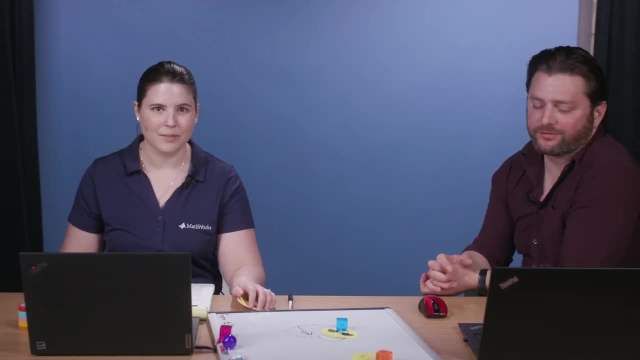 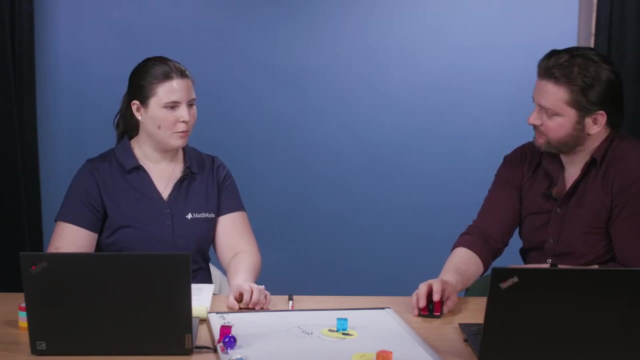 Yeah, and that's something that Kalman filters are actually really good at. I mean the Kalman filter state. it includes the velocity in this case. Yeah, Great. So should we do our demo? Let's do our demo. So before we just showed detection: 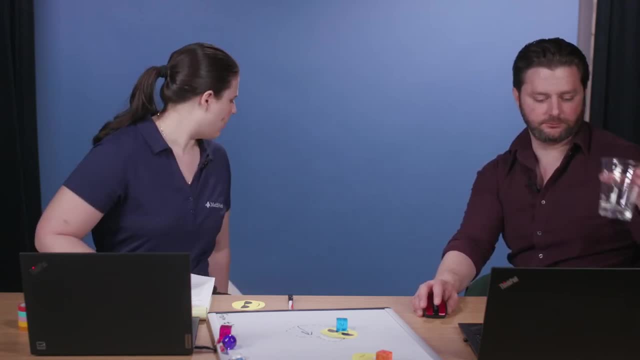 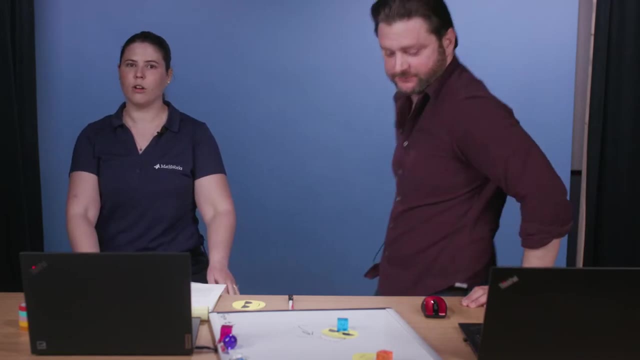 Now we're going to add in tracking. We're going to need some pedestrians. I think we're going to be the pedestrians, because I have been walking successfully for several weeks now. She's gotten good at it. I've been practicing for all of you out there. 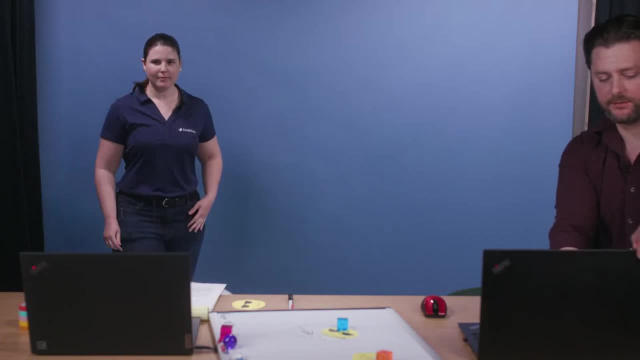 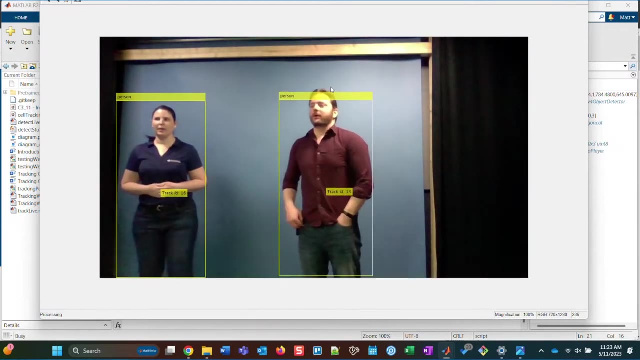 I've been practicing walking in a straight line. All right, let me get this down. Oh, so you see, it already knows that I am track 16.. It knows who I am. If I move, I'm still going to be track 16.. 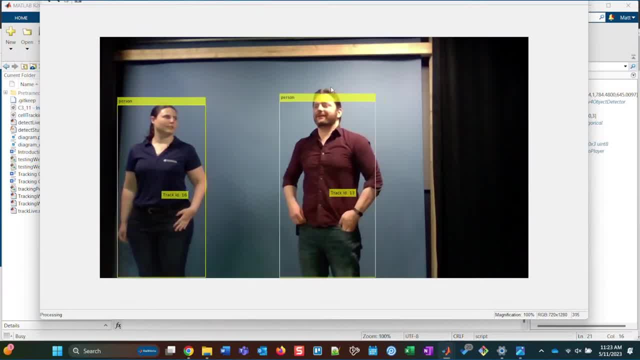 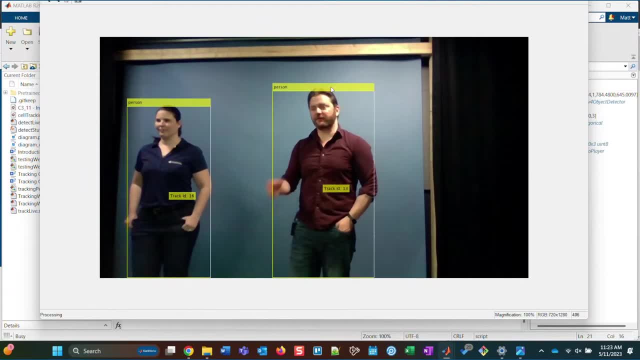 And what am I? 13?, You're 13.. You're unlucky? Yeah, damn. The reason that we aren't number one and two in this case is because the code I have set up actually doesn't confirm tracks until so long. 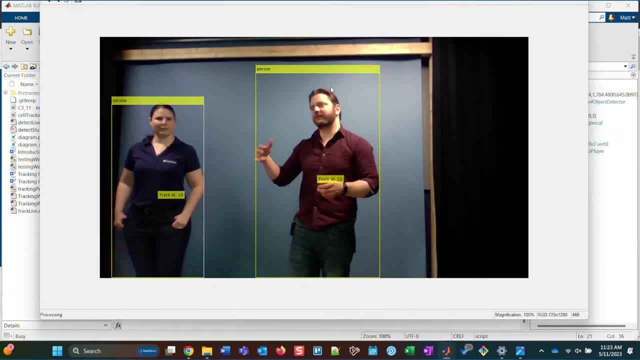 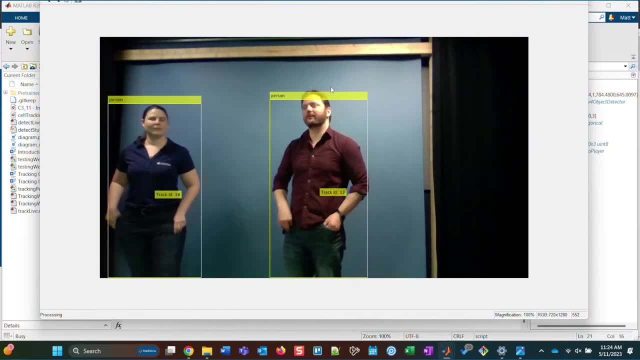 It's that process I talked about, where, even after it says there's a track there, I still wait to display it until I'm more sure. So I guess while we were moving around and jostling things, it saw a few other things that it wasn't confident enough. 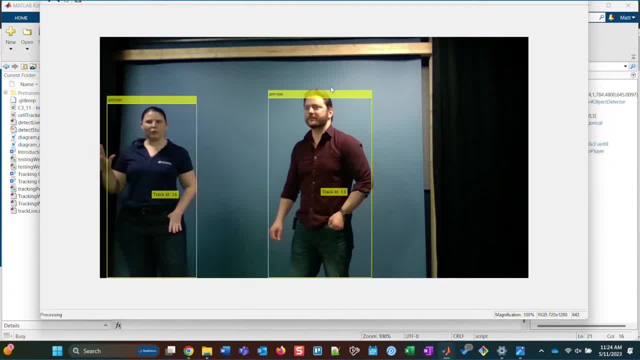 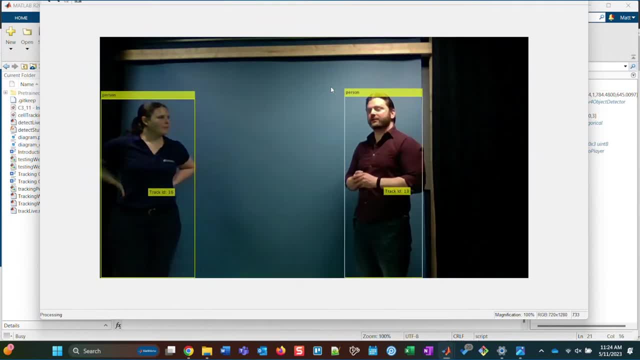 in to display. It's like that might be a track, but I'm going to wait to make sure- And it correctly identified like yep, that's really Megan and Matt. So well done algorithm. So the first thing that you see is yes. 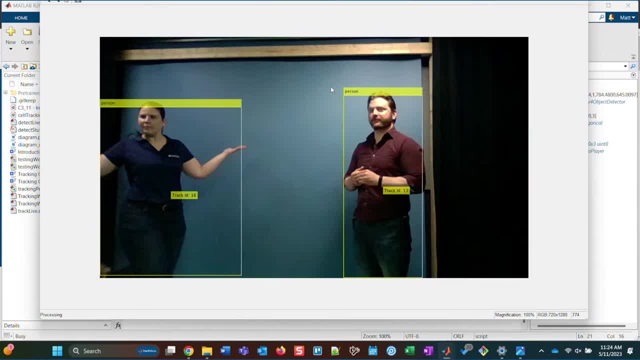 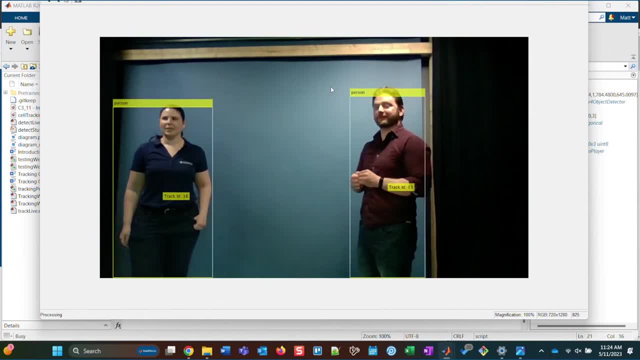 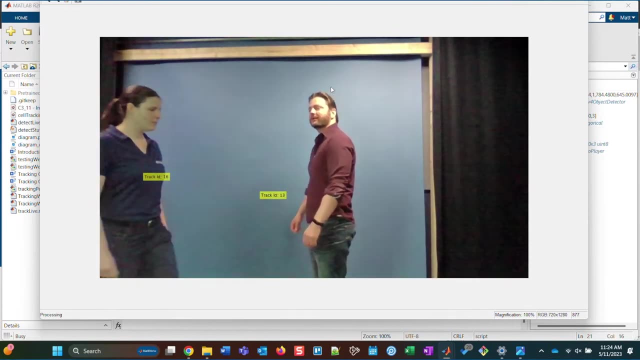 it does tell us apart. We have different numbers, We've been numbered. It's not advanced enough to know our names, but it does keep us distinguished. So now you'll see, if we walk behind each other, that we should stay. Yeah, why am I lost now? 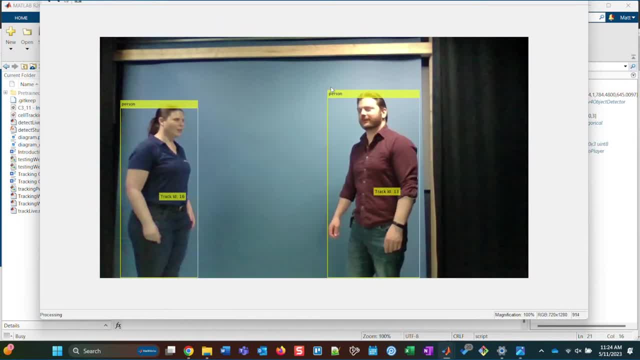 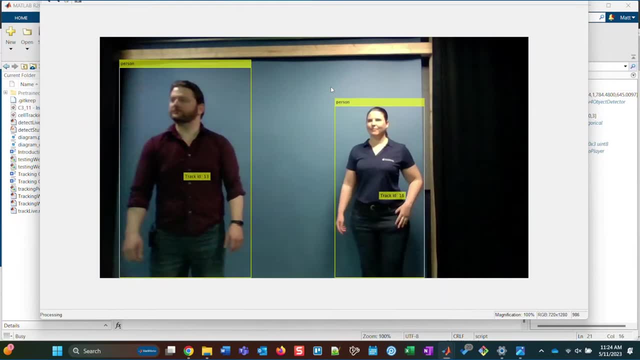 Because we're too close to the camera. I think Anyway, All right, are you walking in front of me or behind? I'll go behind Or in front. We should stay the same track. I'm still 16. A little bit older. 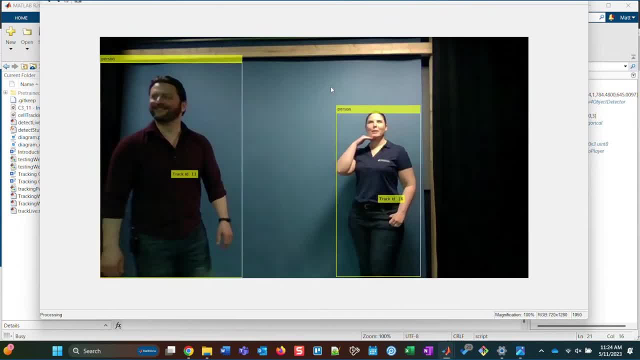 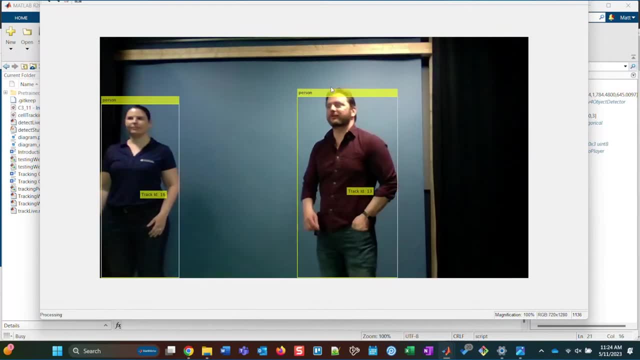 Huh, Nothing, I know, It's my youthful glow, All right, So we can do it again And we should stay Yep. Now, just to mention it, we can screw it up a little now. We are making a fairly simple assumption here. 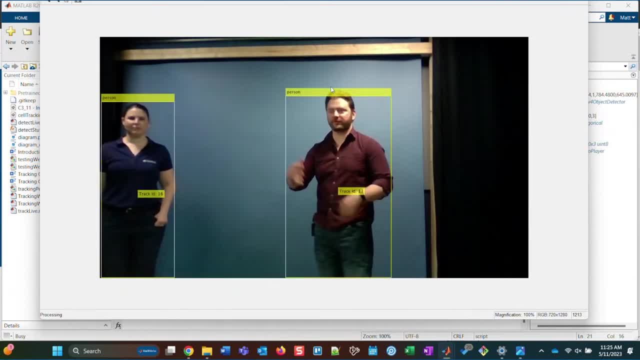 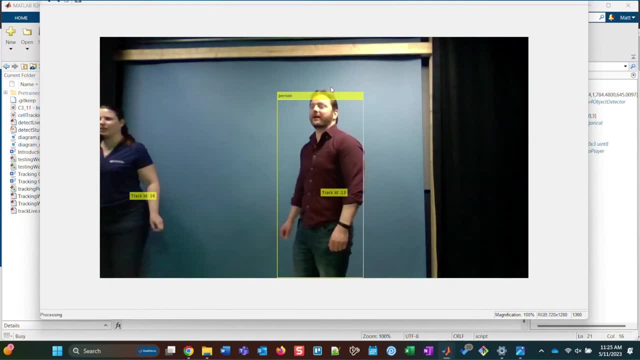 that we have a constant velocity. That's the Kalman filter we're using. It just assumes we have constant velocity, So we probably can get it to switch us if we like do weird things. But it might not. It's doing a pretty good job. 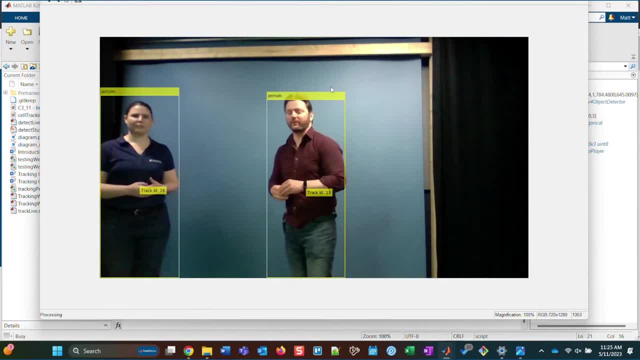 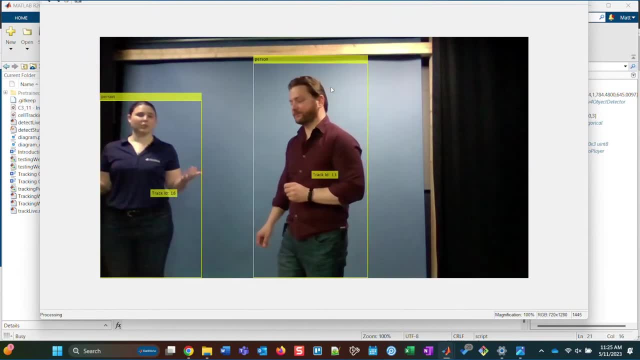 It's doing a pretty good job anyway, But that's one of the things you have to take account of when you are doing this yourself- is your motion model is actually a crucial component of your ability to make accurate predictions, And you can change that. 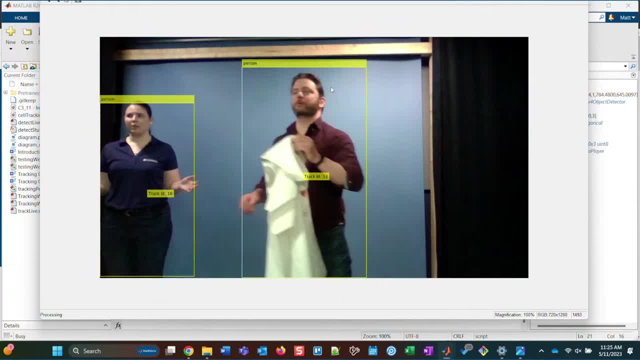 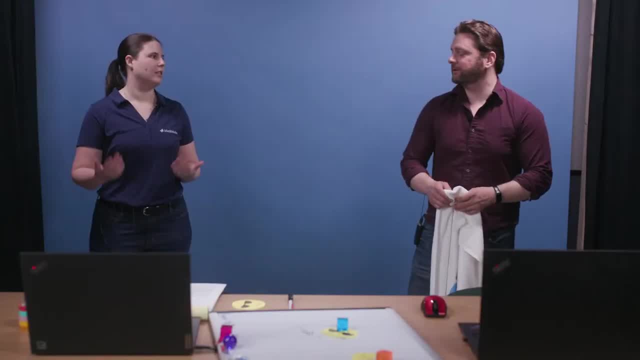 There's a lot of options out there for changing your motion models. We're using a simpler one because it works great for our application, but also because it's, you know, easy to talk about and explain in this kind of venue. But you can come up with whatever detection model. 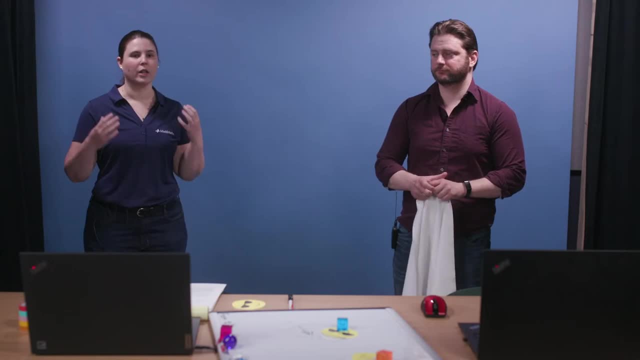 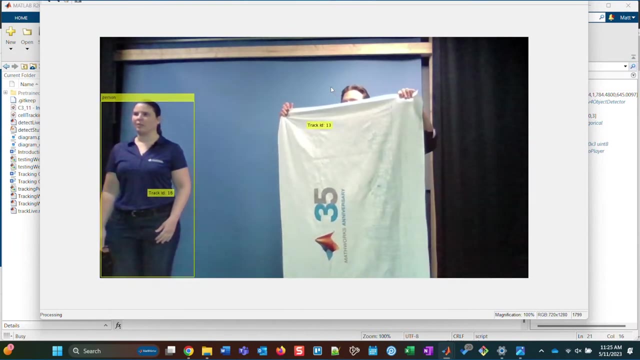 works best for your data and whatever motion model Like. if you're working with very jerky motion, you're going to want a motion model that accommodates that. We've lost Matt. He's no longer here, according to detection, But tracking still knows he's there. 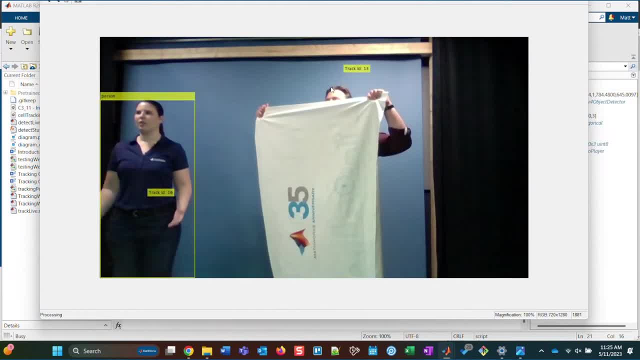 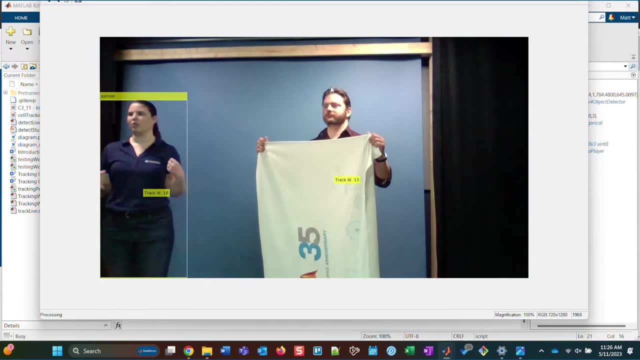 So what is that doing, though, when it's drifting? So what happened is I went way too fast, Yeah. So what happened? is it lost the detection. It assumed he was going to continue at the motion that he was doing before. 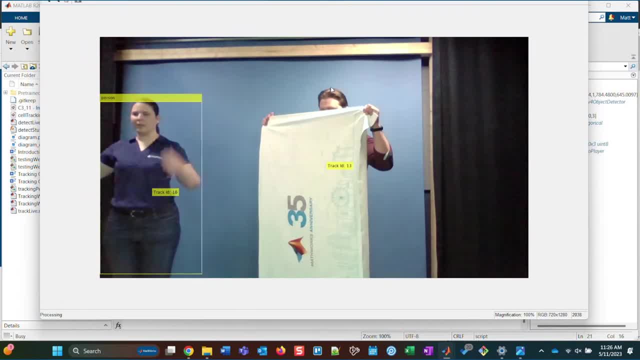 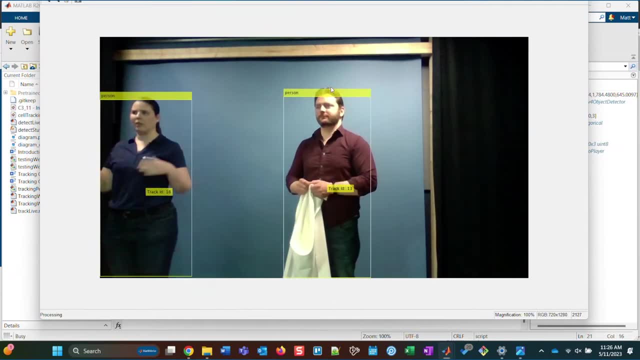 So when he was moving, like going like this with the blanket, it assumed he was going to keep moving. That's why the track drifted up. But when he did the blanket, it covered himself really slowly And even though we are using, you know, 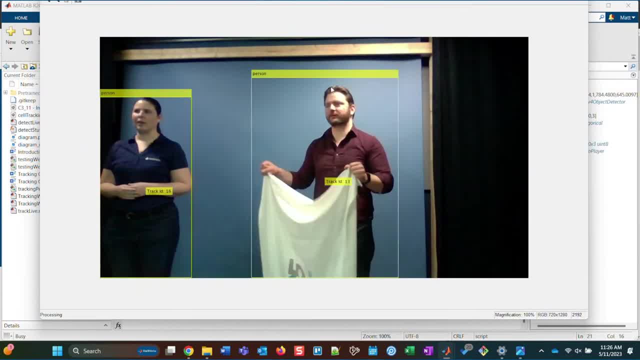 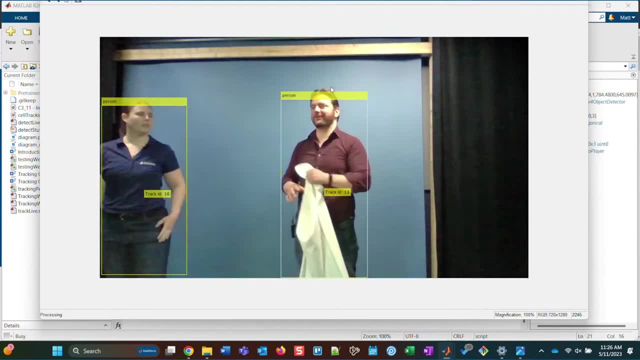 a pretty good detector here. it's still. You can see it's noisy. right There's some jitter, But when he did it. you know slower It does if I go up fast, But you could adjust that too. 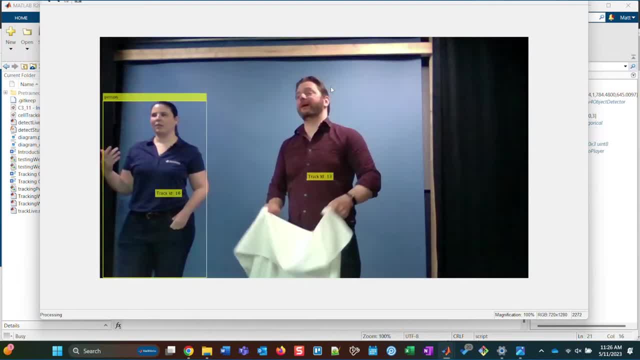 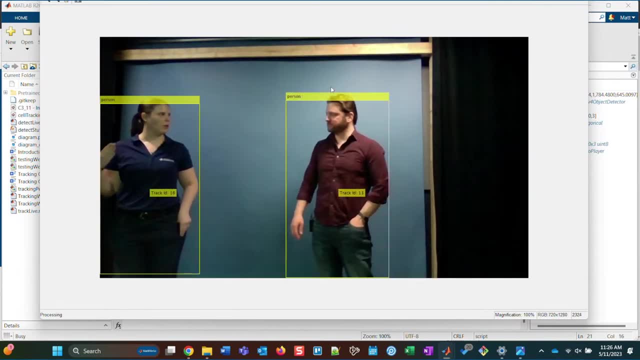 But anyway it finds me after I come back out from the towel and it knows I'm the same person. The track thinks you're going to continue doing whatever you were doing when the detection lost you And then, when the detection finds you again, it resets. 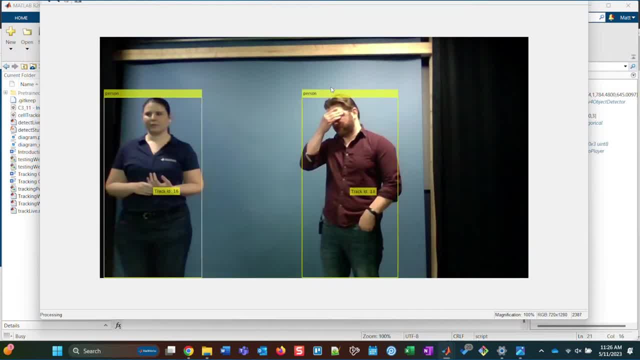 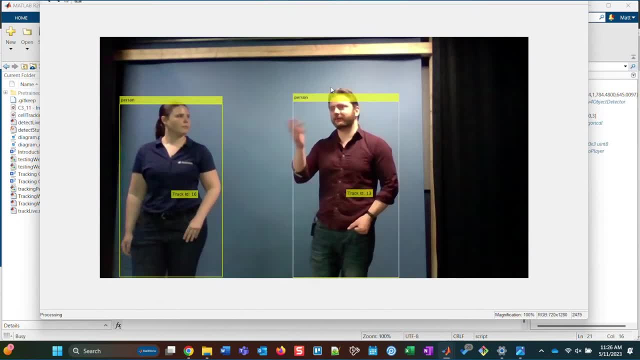 And I should mention, for those of you out there who are, you know, experts in Kalman filtering: yeah, if you have a more complicated model of your objects and you know inputs to them, you know you don't have to assume that it's going to keep doing what you saw last. 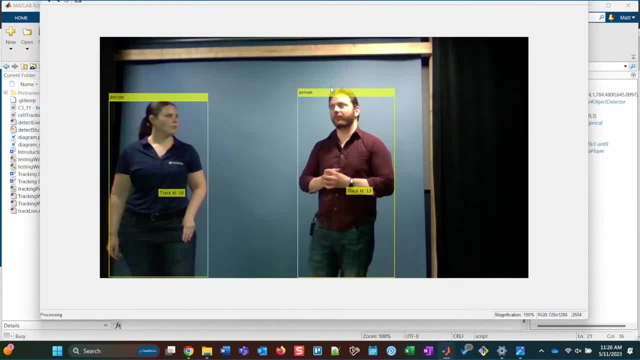 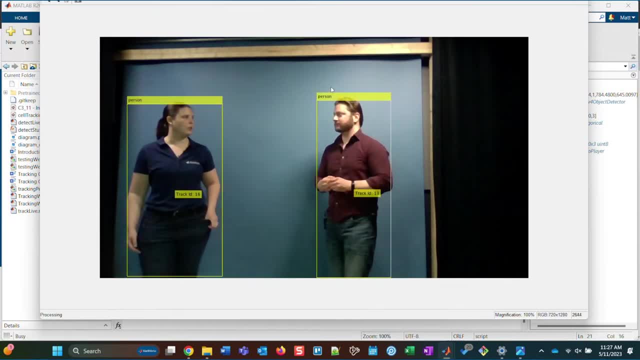 You may have more information and you can incorporate as much information as you want to into your track motion model. When I was still a speech researcher, we used a Kalman filter to measure the motion of the parts of your throat and mouth to figure out what words people were saying. 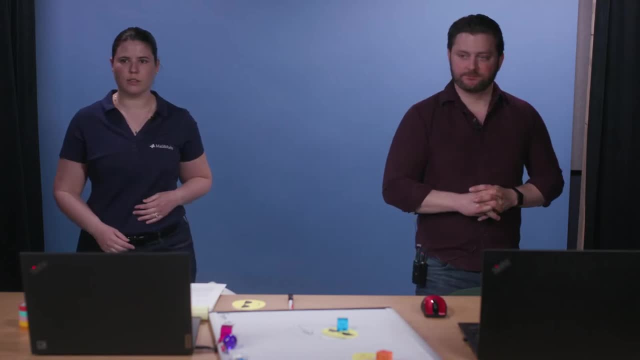 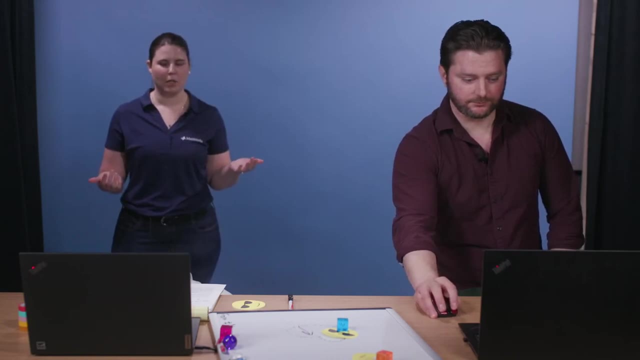 Nice. So there's a lot of wide-ranging uses for this And for the obstruction. it seems sort of silly for us to hide behind a beach towel. You know we're basically playing peek-a-boo with the computer, But that's you can imagine. that would be really important. 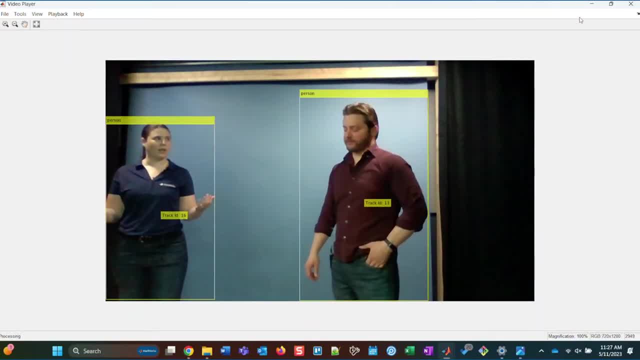 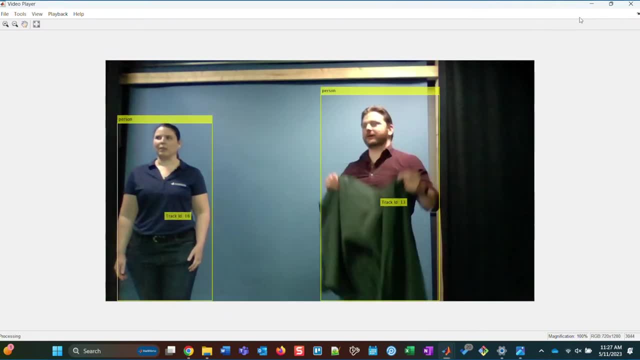 if this were, example, in a dash cam and they needed someone who you know if they had their coat up? Yeah, or I walk behind something like a bush here. Yeah, You want to have me reappear again. You know, you want to have some notion. 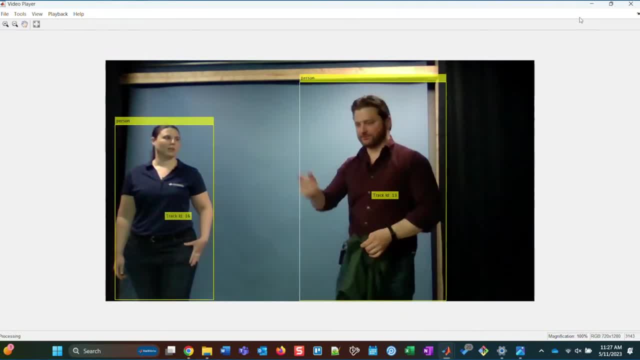 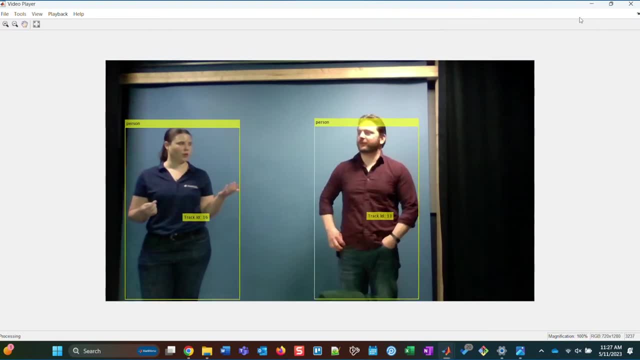 that I haven't disappeared completely. Just because a pedestrian's behind a bush, there's still going to be a pedestrian And they, you want to know the pedestrian's there. so you're, you know, safe with your car, So you can activate the brakes. 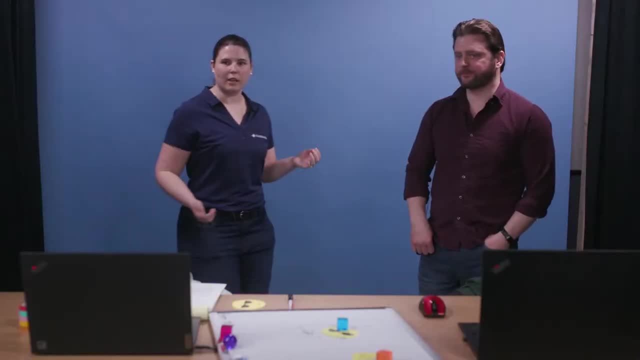 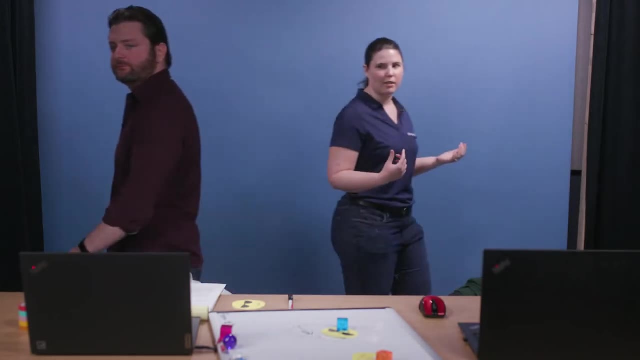 So you can activate the brakes on the car. But also the idea of the track is: it says, if you're moving, you're probably going to continue moving. So the track will actually predict in a minute he's going to walk out from behind the bush. 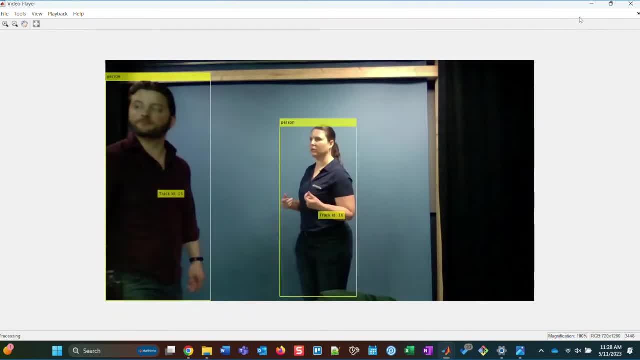 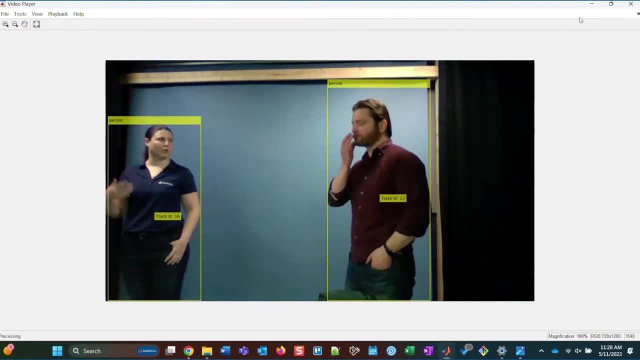 So the track correctly predicted where I was going to be after I walked behind Matt, So it could say like, hey, that pedestrian's walking towards the street, They walked behind a parked car. I think they're going to appear in the street. 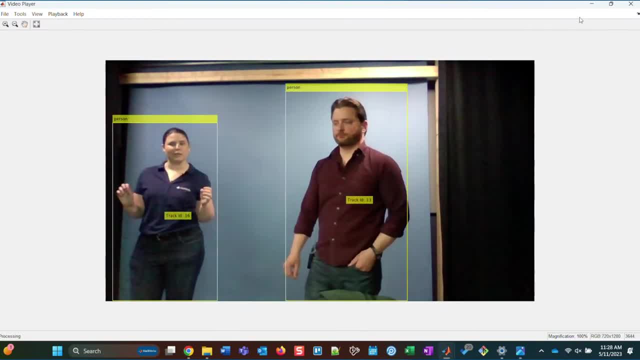 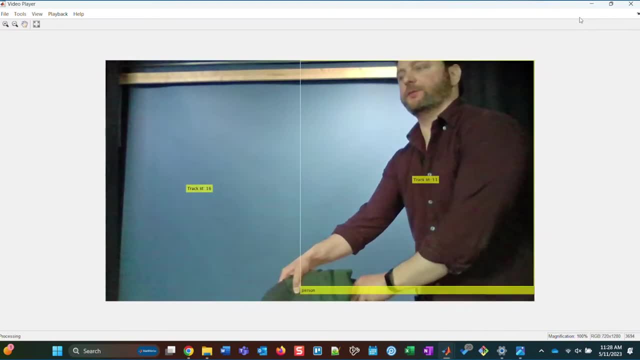 And so they still hit the brakes even though they're not currently detecting the pedestrian. Yeah, that's a great point. Okay, and again We have more questions. We're just tuning in Ask questions. We love questions. Ooh, we've got some good ones. 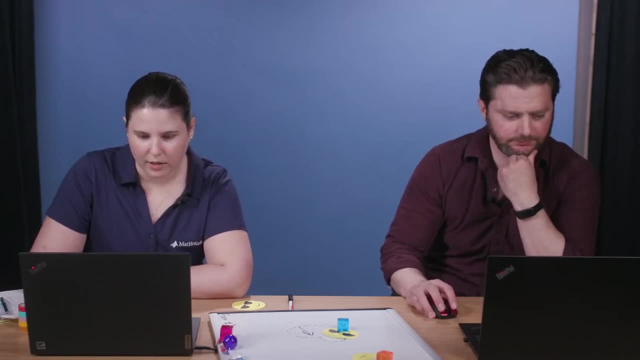 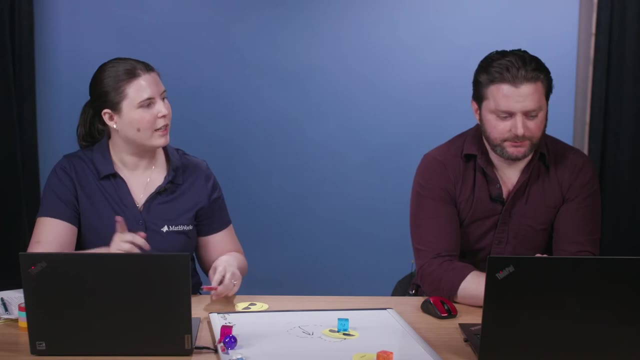 Okay, What kind of algorithms do you use to track objects? Maybe MobileNet, DetectNet, YOLO, thanks. What do we use for detectors? Yeah, And where can they find these for MATLAB? Oh well, there's several different ways. 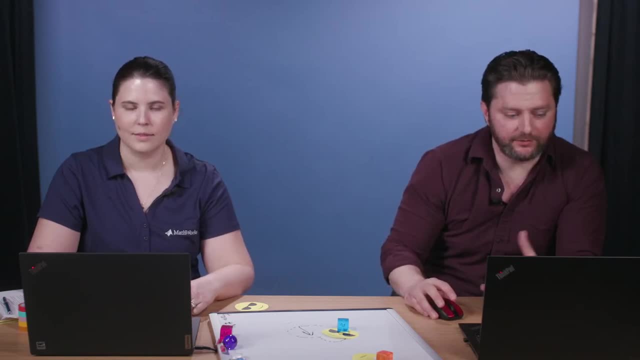 to get the pre-trained detectors. We have different variations of YOLO in MATLAB, On the Model Hub. well, we have, I think, version 2 and 4. currently, 7 will be soon, I'm told. Don't you know? don't hold me to it. 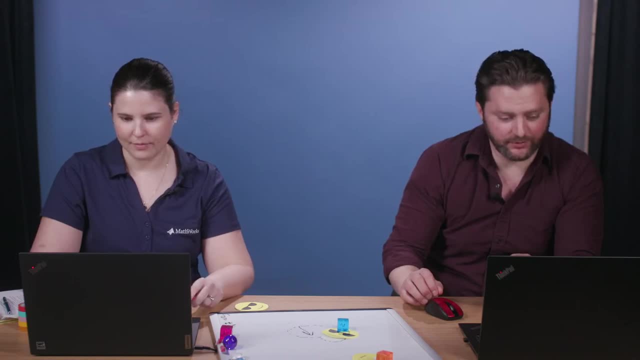 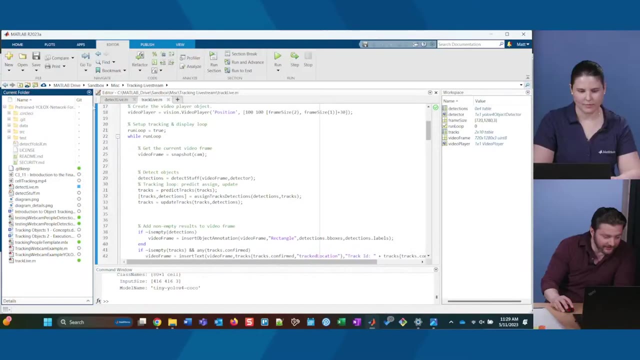 And YOLO X is actually a very new high-performance YOLO model that's currently available on the Model Hub. So, if you saw, I tried it out. I didn't use it for this demo, but I did download it from the Model Hub. 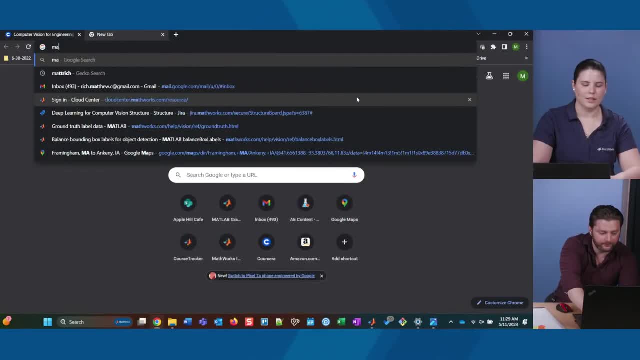 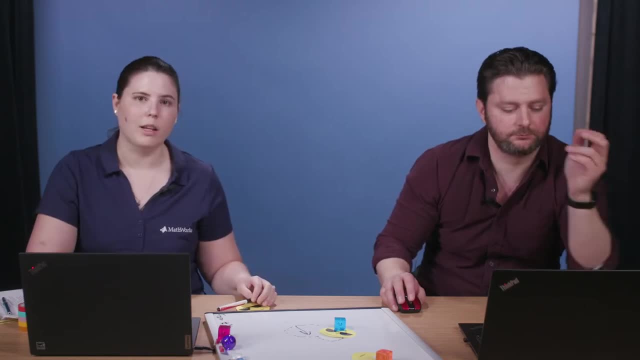 So let me show you that, if I can remember how to get to it. What speed can you handle in real time? That's a good question here. So right now we're actually using a GPU hooked up to the computer to do this real-time imaging. 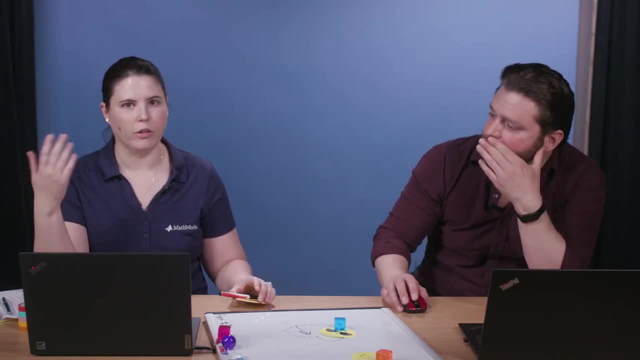 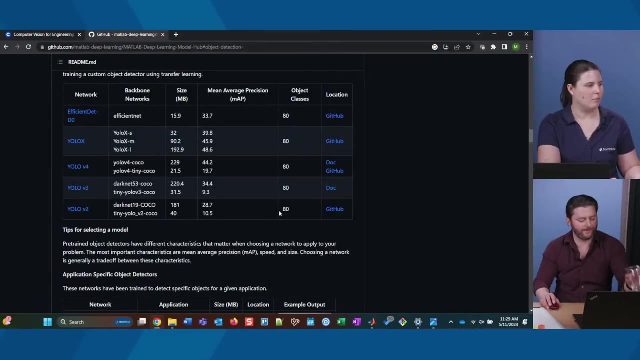 You can see that it's. there was almost no lag. This was all live over the stream. This wasn't. none of this is prerecorded because we have a yeast cell. We don't actually have yeast cells here. So if you have a GPU with a webcam, 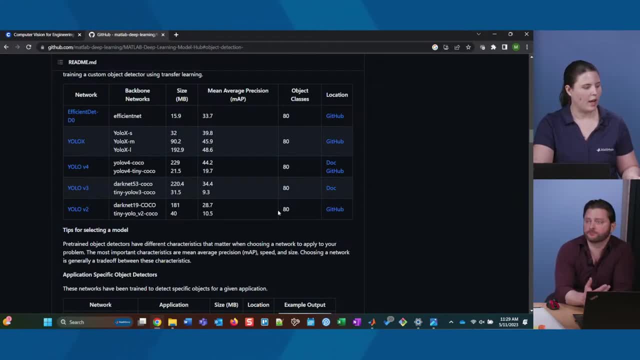 it can be pretty much live If you didn't have a GPU, if you just had your computer CPU. we tried that too. There was maybe like a second lag. Yeah Well, I'm using what we call the tiny version of YOLO. 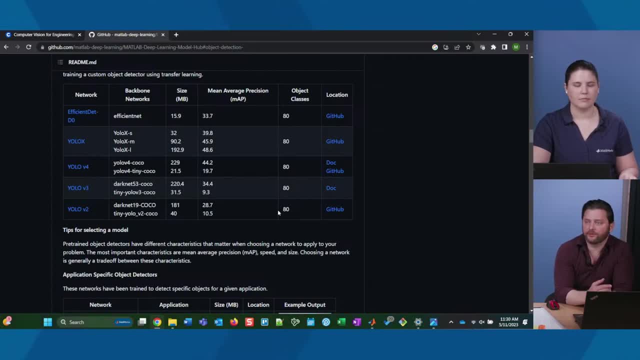 So it's a smaller network. It's a bit less resource hungry. I think YOLO X is in fact YOLO X runs the same. I also ran YOLO X with no GPU And you could tell I mean there was some lag. 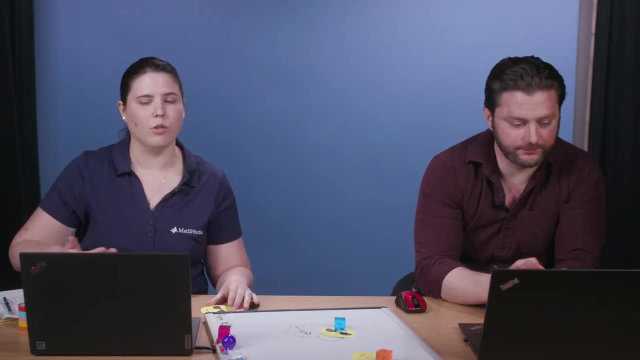 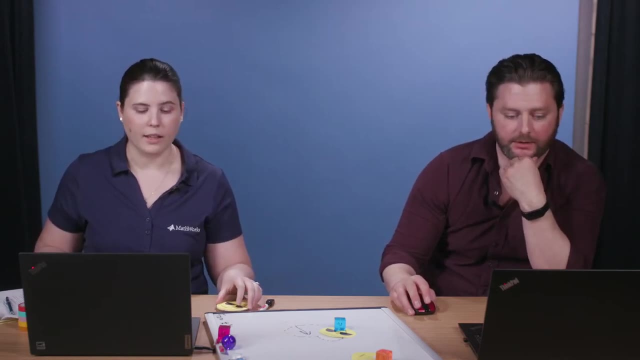 But I mean it wasn't like it didn't work. It's still pretty fast, And a lot of what you want to do for tracking algorithms it's actually going to be for prerecorded videos, So it doesn't matter as much. 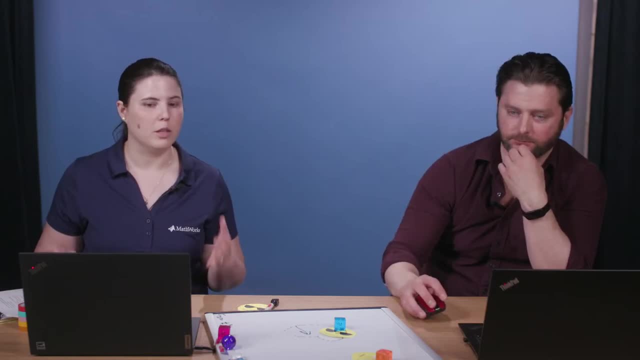 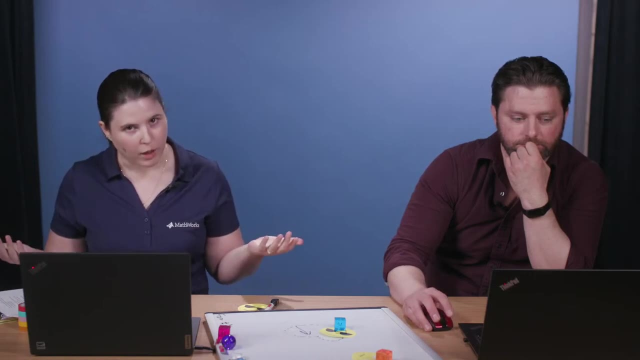 But it really just depends. If speed is more important to you, maybe use a smaller detector model. If accuracy and fine-grained detail is more important to you, you might want to use one of the larger deep learning models. It's just a trade-off. 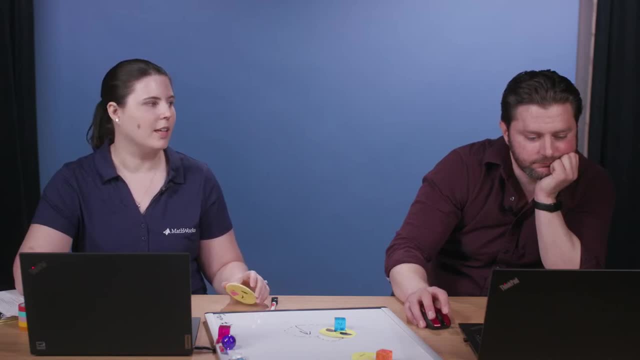 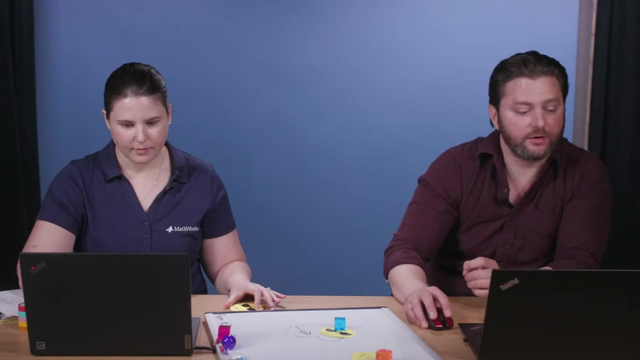 But you can. even with fairly complicated and fairly accurate detection models and a CPU, you still get pretty fast results. I've done it and it's like maybe a second delay. So just going back to the person who asked about what models are available, 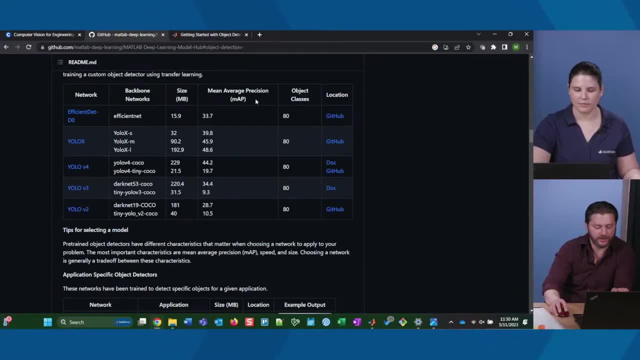 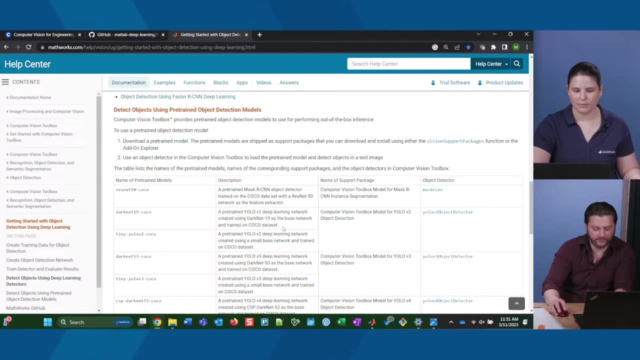 I was showing the model hub. That's where you can go download some pre-trained models that are not currently like completely part of the product but they still will work within the product, And then to get the ones that are kind of more fully integrated. 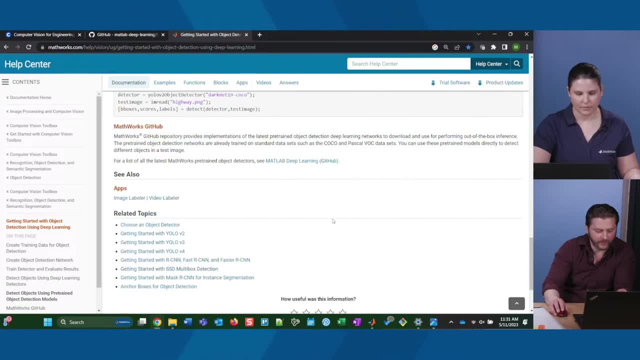 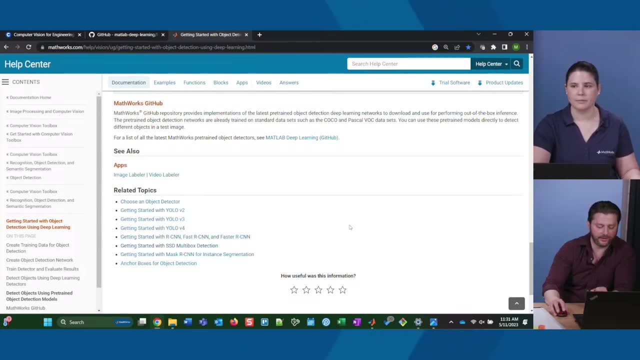 just go to the doc pages and you can see there's. well, I guess this isn't really listing them. Basically we have faster RCNN, various types of YOLO and SSD. So we pretty much cover the one major type of. 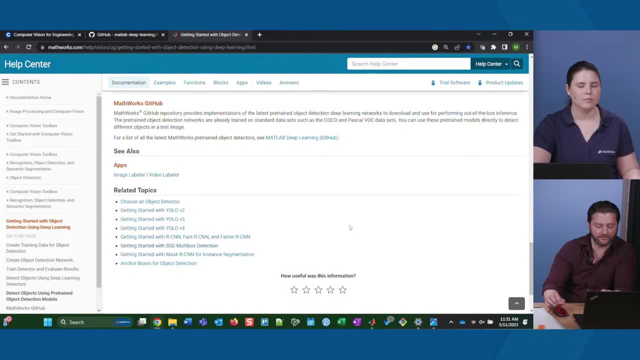 it's called two-stage detection, which is RCNN, And then we have the two popular single-stage detection methods, which are SSD and YOLO. You can also train your own detector, which we do. show you how to do, Not yet. 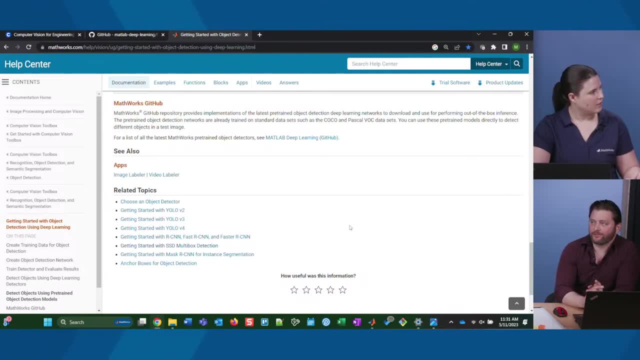 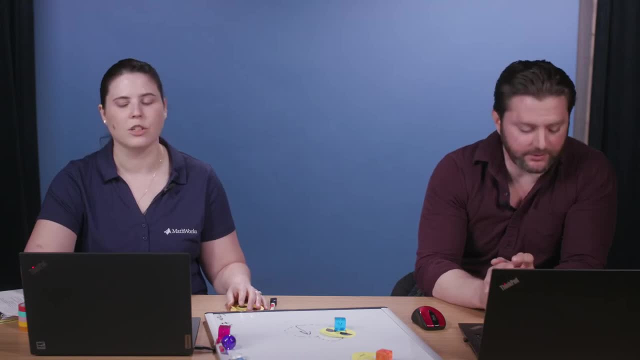 In image processing? Oh, you can't. We do not train a deep learning, We train an object detector. Oh, not for a video, But you do train object detectors, in course. Object detection- Oh, yes, Yeah, yeah, yeah. 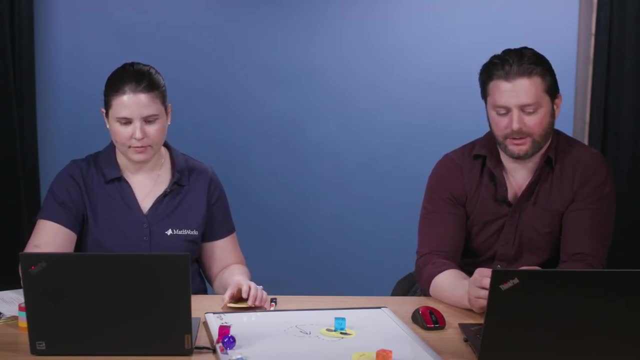 Okay, So in coursework we already have on Coursera, We do show you how to do like feature-based machine learning object detection, And then we will, at some point in the future, show you how to train object detectors your own neural networks. 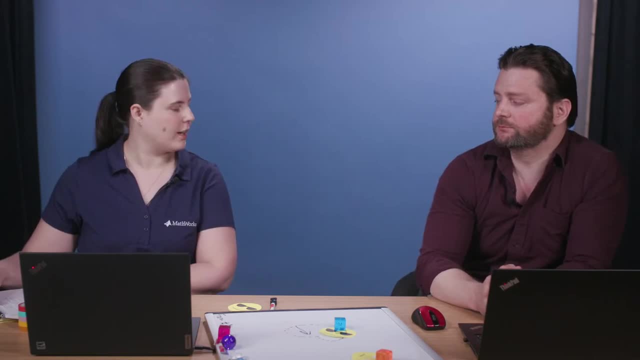 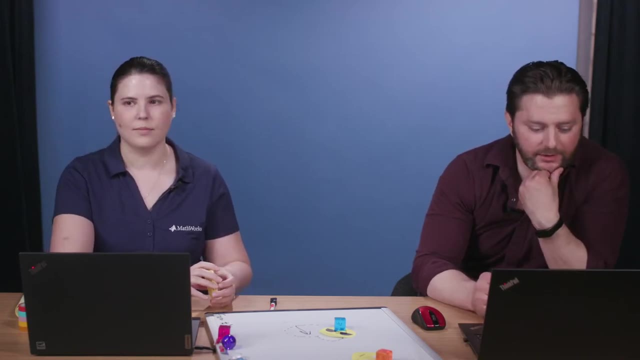 Yeah, And then we will show you how to train the human intelligence power, And then we'll see how to train the information in front of the machine. So you've got data and you can train, actually compute information, such as the자 and data and data. 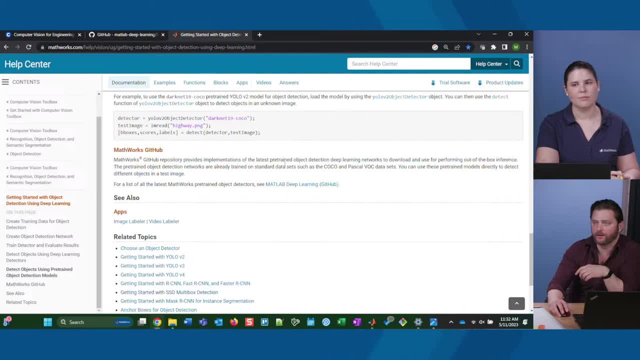 And it depends on the machine, And if it's a virtual machine, like a digital machine, it's actually not going to run. It's going to run, It's going to run. Oh, so it's going to run in the same environment. 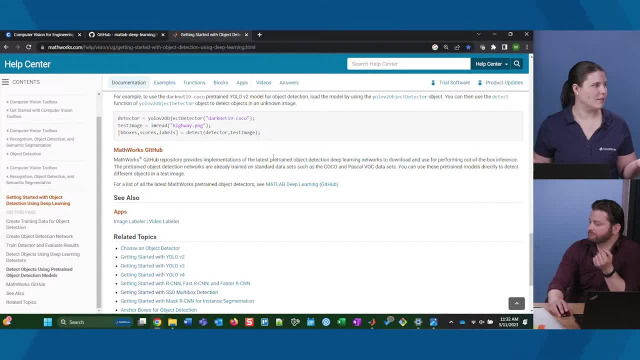 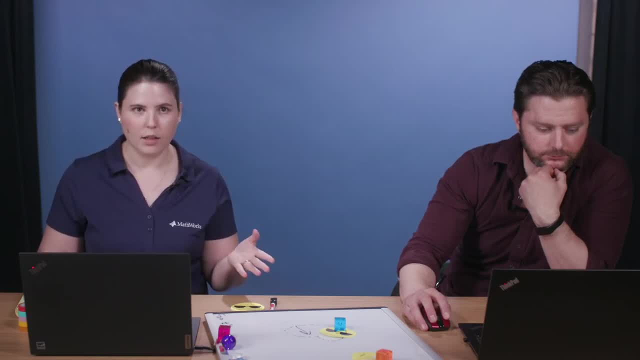 So that's practical, Yeah, And unfortunately we don't have enough information on the machine for trading off, like: maybe a larger model works great on MATLAB, but you need it to be really small so it can go on a Raspberry Pi. 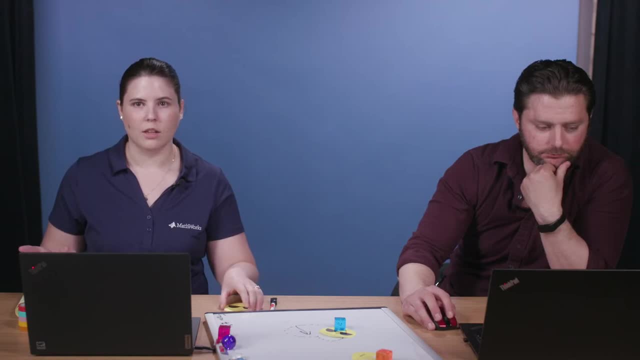 And then we'll talk about some of the trade-offs of that. for like, yeah, let's you know, why don't you train a smaller model? And these models can run without internet connection. This mysterious Brandon Armstrong seems to have already answered that one. 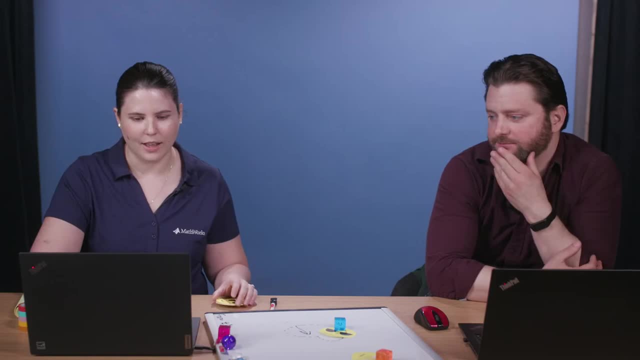 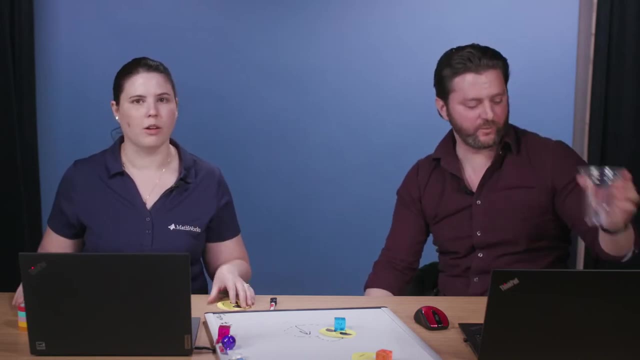 I don't know who that is. He doesn't know what he's talking about. But yes, these models. once you have installed the model, this can all run without internet connection. We weren't actually using the internet for any of our demo. 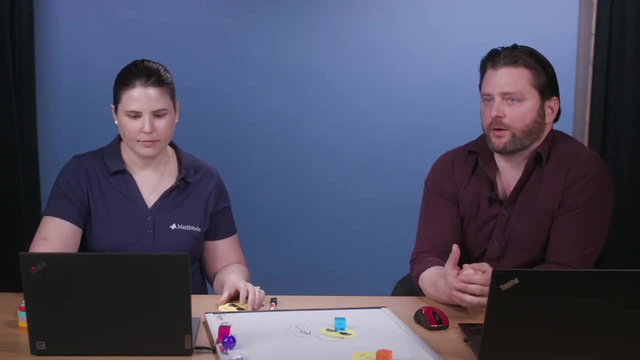 That was all local on the machine, correct? Yeah, the internet is only required to like download the initial model. if you're getting it from the model hub, If you've installed MATLAB, it's already- well, no, it isn't. 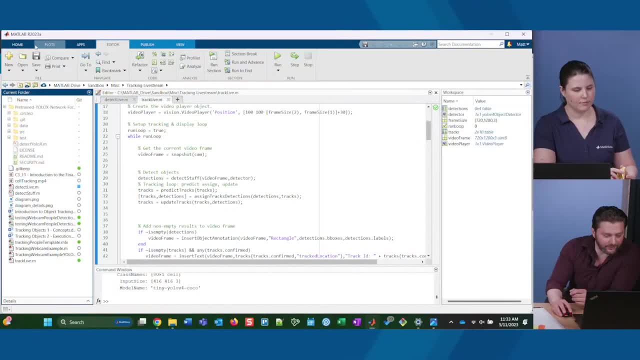 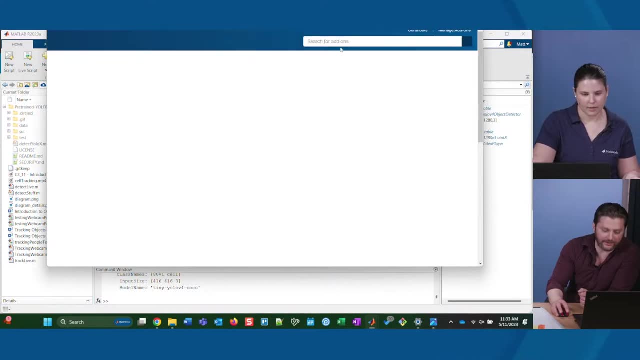 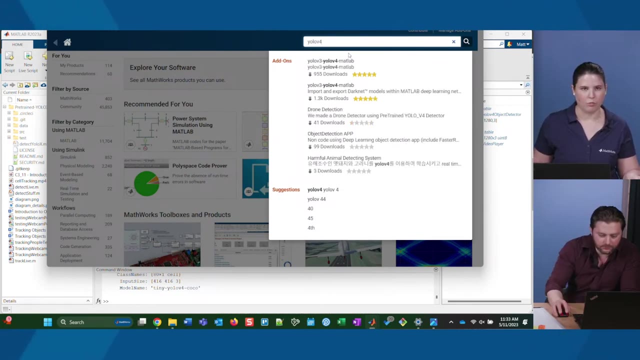 There's. I guess I can show them that too. You may need to go to this thing called add-ons and get add-ons, And then you will download, for example, the support package, for we also have a question about whether you can try. 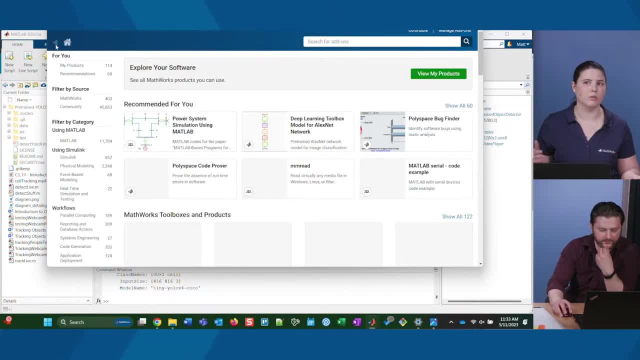 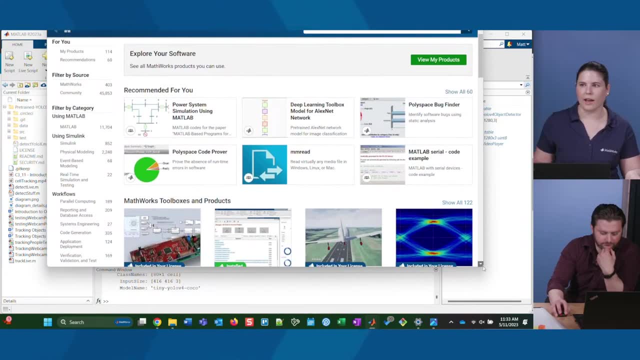 this stuff out for free. And if you take this course, it includes a free license with all of the packages you'll need for the duration of the course. So you can get a chance, without you know paying for MATLAB, to try out all this stuff for yourself. 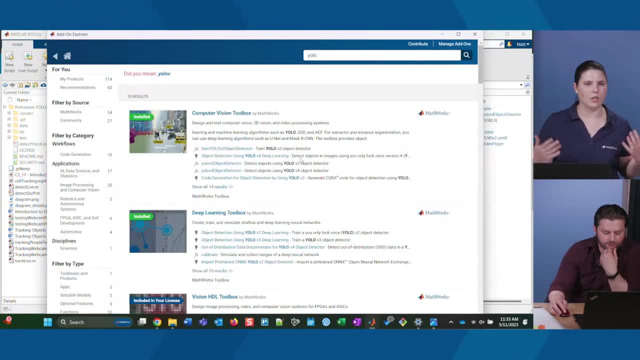 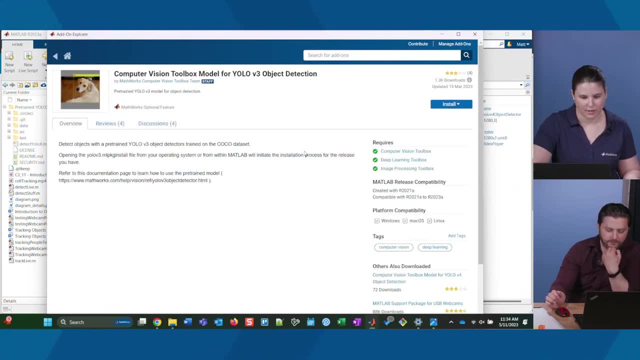 So that's the beginning of each of our Coursera courses. There will be instructions for how to download and install MATLAB so that you can- you know, you don't have to already have MATLAB, but you can download it from MATLAB to do all the material in the course. 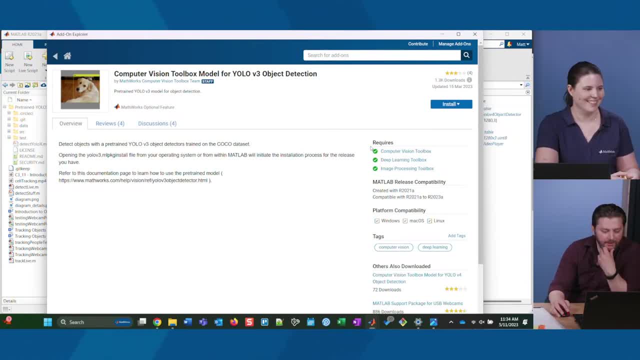 Okay, so I finally found one. As you can tell, I'm a great search bar user. This is the V3.. I haven't installed this one. I have installed the version four. So all you do is you'd find this here. 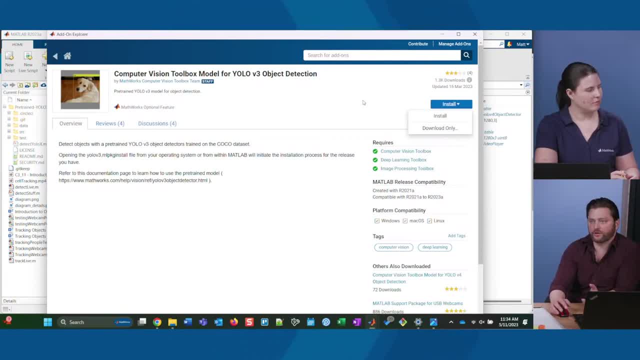 and then you'd click install. The nice thing is, if you try to just use the functions in MATLAB, it'll prompt you to go to this page and install it, So you don't even have to search for it like I did, Do you? we're getting questions about the GPU. 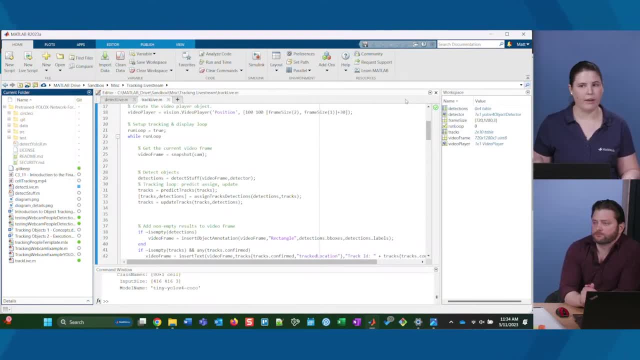 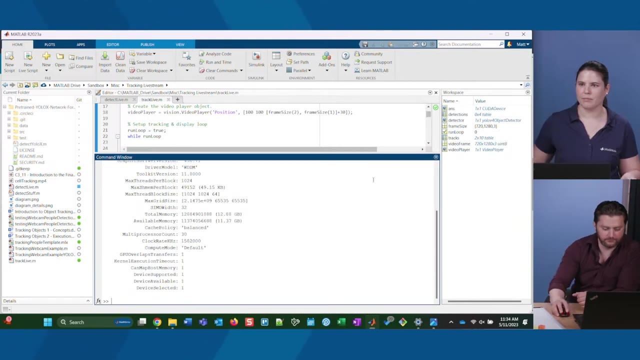 and how MATLAB will automatically detect and use compatible GPU. Do you want to show how you do that on the MATLAB command line, how you find out what GPU you're using? Just this right, Yep, See, now we know all the information about our GPU. 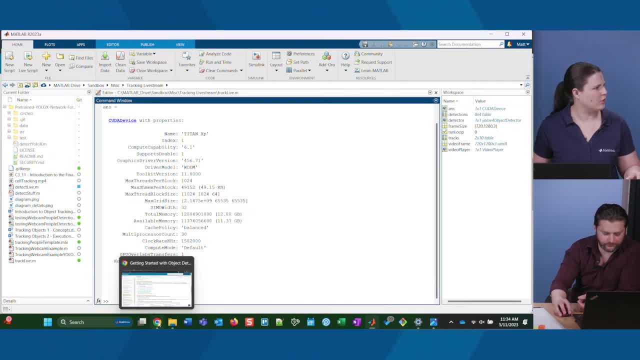 We hooked it up and it automatically found it on the GPU device. We might have had to install a driver, but that has more to do with the GPU. Yeah, you'll have to do it through the GPU drivers. I can't remember if there's a. I don't remember if there's a support package for it, but again, it's very user-friendly. if, well, The MATLAB side of it's automatic. If you are already using a GPU for gaming or anything on your computer, MATLAB should be able to find it. 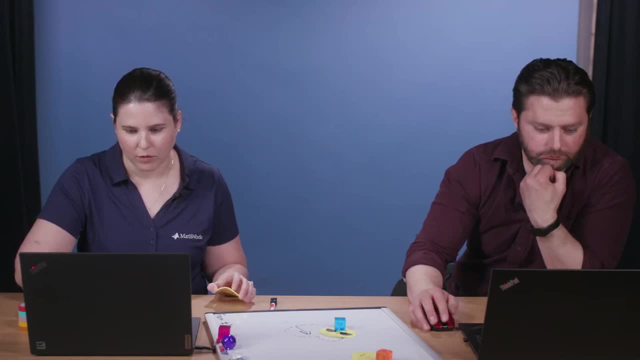 What about detection? in the Tesla and other cars? There's a bunch of things moving at the same time, and what type of hardware does it need? So what Teslas are doing? my understanding is it's really similar to what we're doing today. 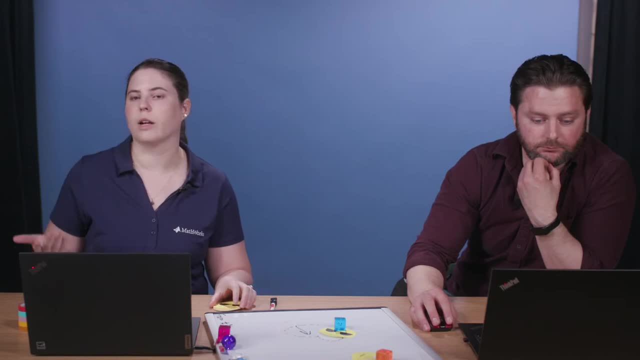 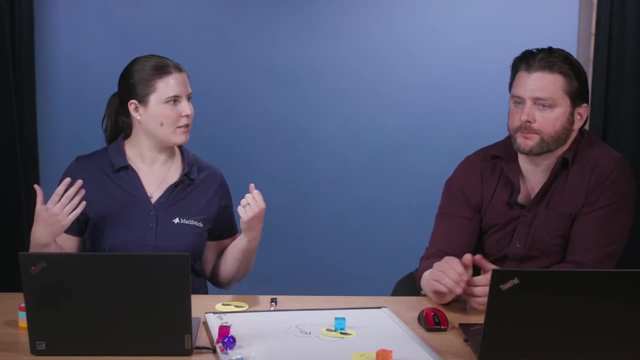 is, these pre-trained models already have a lot, of, a lot of different objects in them. We didn't show that as much because there aren't that many objects in the video like we don't have in the studio. we don't have a bicycle with us. 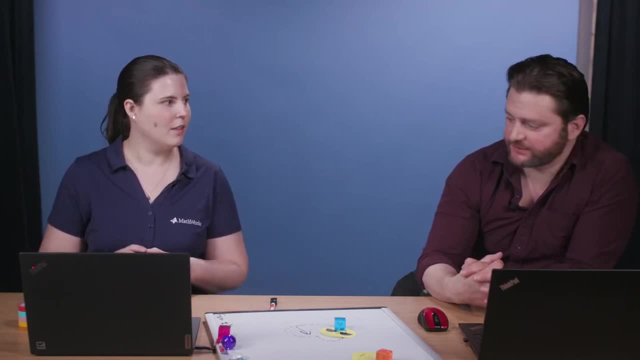 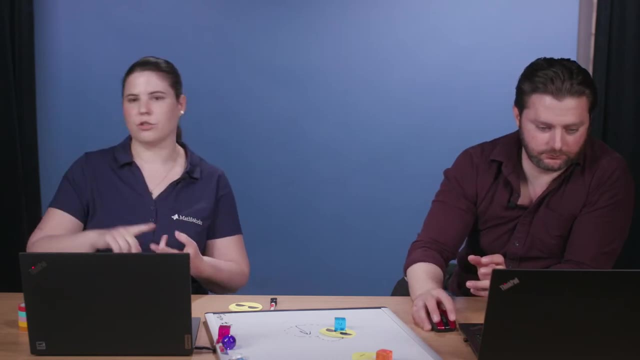 we don't have a car, we don't have a dog. We could have brought some stuff, I suppose, but we didn't. But it will automatically. the same algorithm we're using will show like cyclist pedestrian, backpack dog. 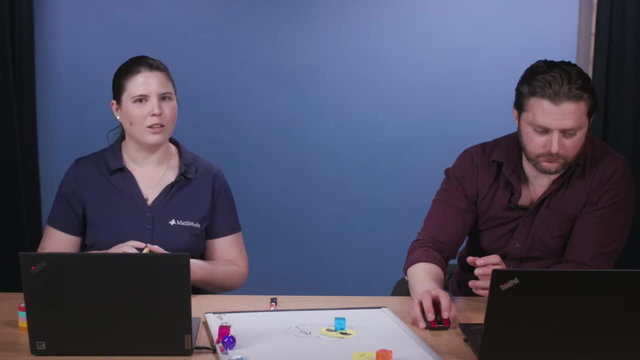 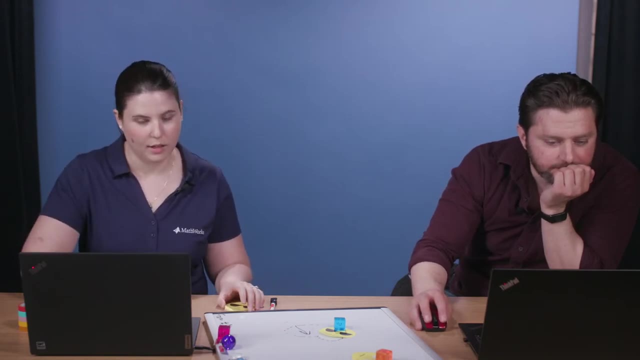 There's even some kind of like out there, ones where it like it, can you know it can detect, like certain dishware, which hopefully no one is throwing dishware at your car, but if it, if they were, you could detect it. 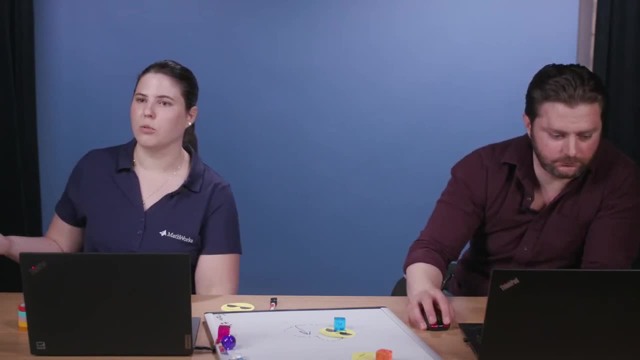 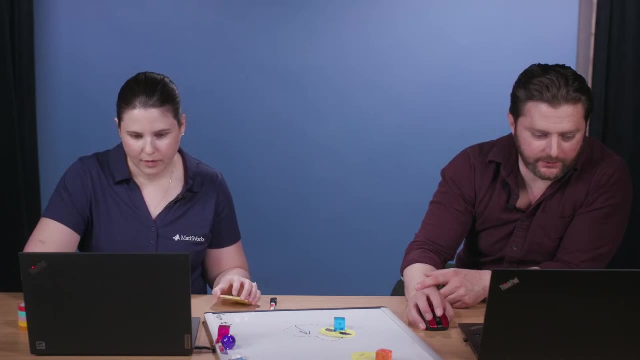 So it has a lot of different types of things, which is important because, you know, maybe you can expect cyclists to behave differently than pedestrians. So this isn't so it'll get all these things, basically The pre-trained networks that we have in MATLAB. 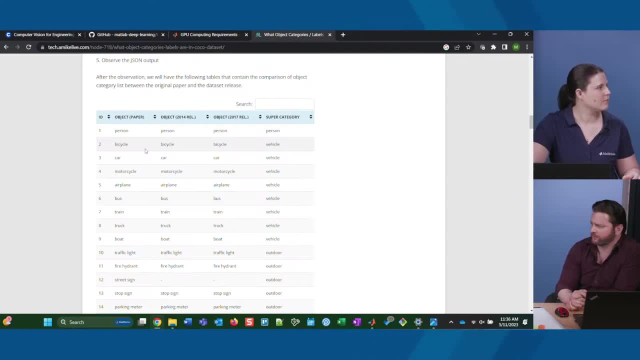 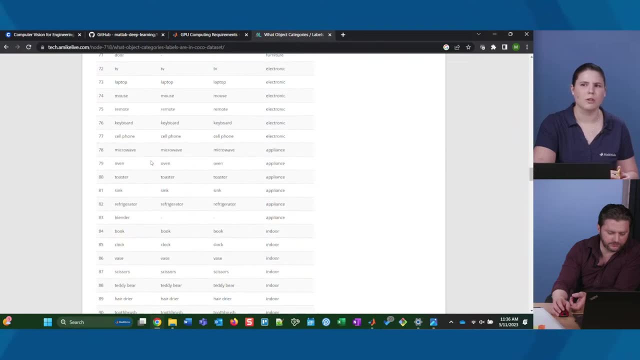 were all trained on the COCO data set. at least the YOLO ones were for sure. So this is your list of classes: Motorcycles, traffic lights, street signs- Pretty cool. Yeah, Snowboards probably won't come up. 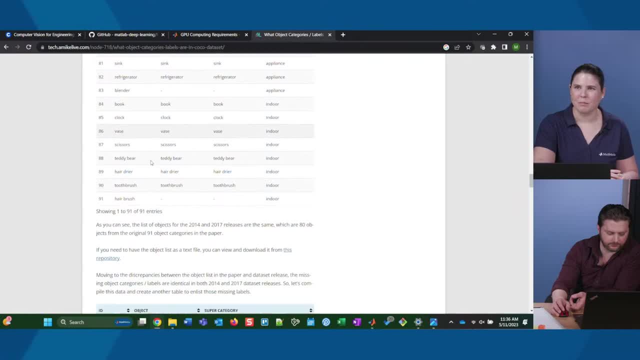 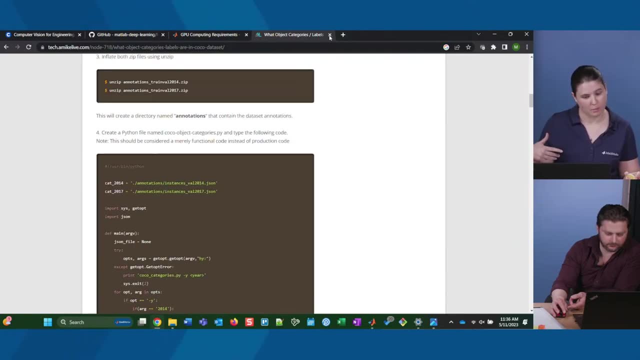 Carrots? maybe not, But if they do you'll be ready. But yeah, you see a lot of things that you can find on the road that would be important. Mirrors is actually pretty useful to show if it's a pedestrian or pedestrian in a mirror. 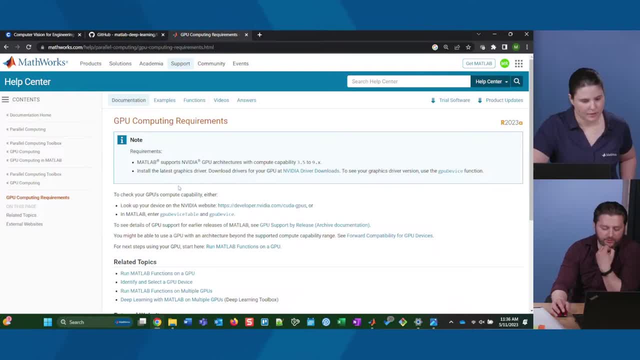 That's really helpful And I did want to double check because I couldn't remember. it's been a while. if you had a support package for GPU computing and you don't, You install the graphics drivers for your GPU, Which, if you're already using the GPU. 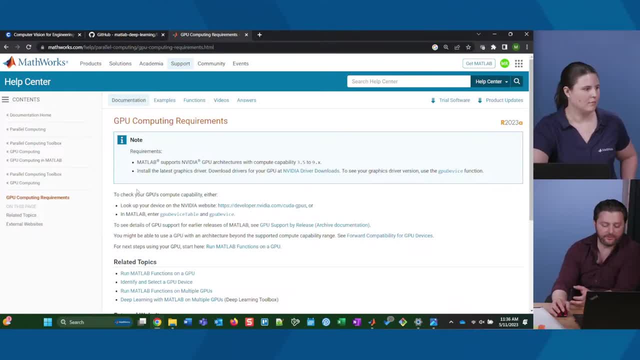 you already have, You already have it. If you have an external one, like I, did you install drivers, plug it in and that's it. As soon as you do something where MATLAB can use a GPU, it will, unless you for some reason tell it not to. 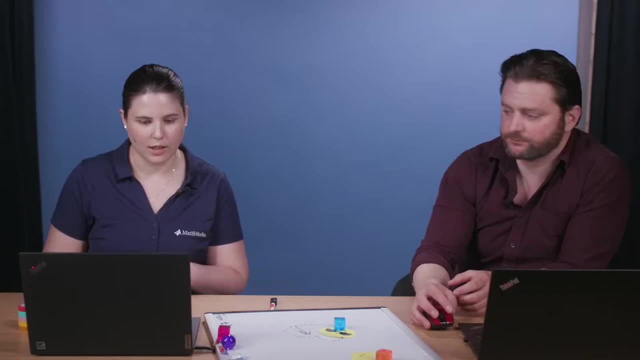 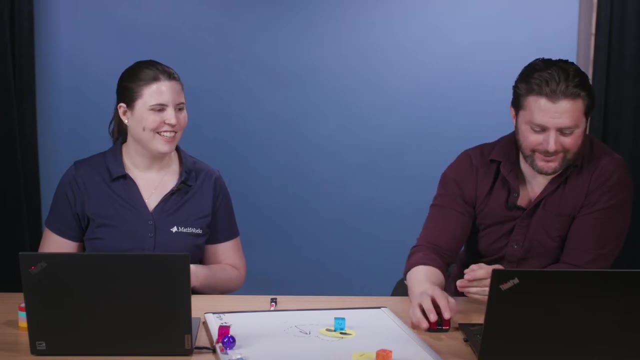 Yeah, you can tell it not to if you want to. Ooh, this is a good question. MATLAB offering a labeling tool? Yeah, MATLAB has a labeling tool. It's a very good labeling tool. I hear very good things about it. 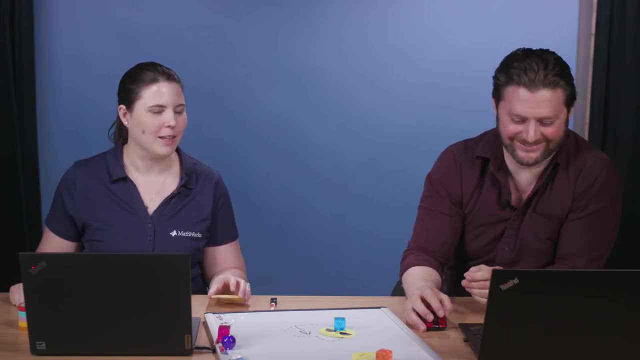 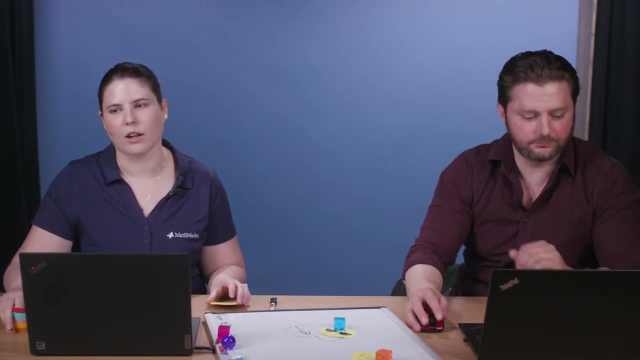 Brandon Armstrong loves it. I actually am a big fan of the labeling tool. I'm sort of dorky about it because I resisted labeling things for a really long time because I thought it would be a pain, and I spent a lot of time trying to figure out workarounds. 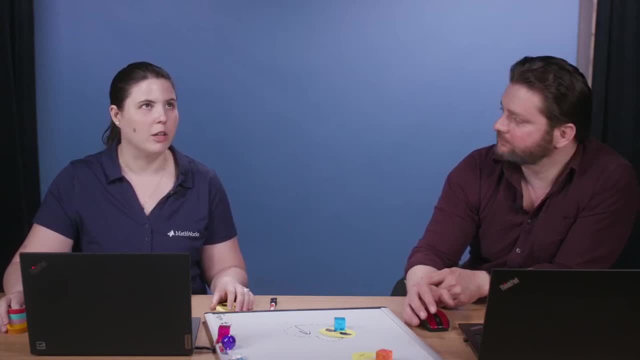 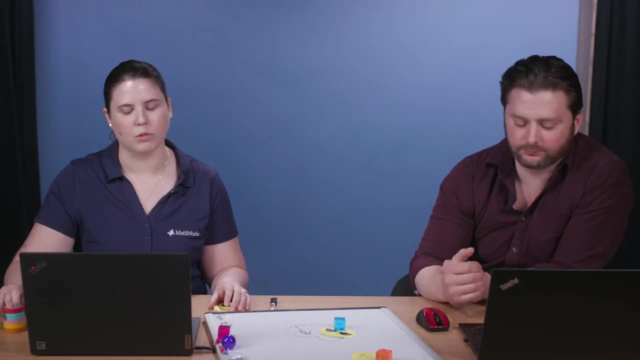 and then when I actually did it, it took me like I don't know 35 minutes to label whatever. 19 times 60 is like a lot of images, and it was really, really fast, and so I wish I hadn't been putting it off. 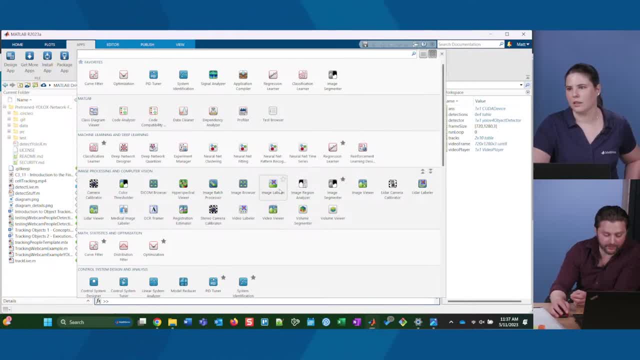 That app for your information is in this apps menu. here, and I think you're referring to the image labeler, We also have a video labeler which is pretty similar functionality. if you want to do that, They work really similar. 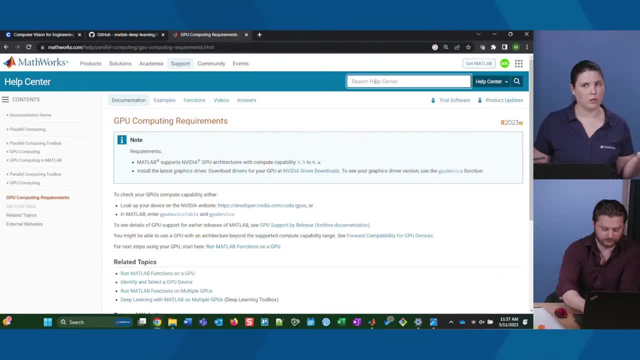 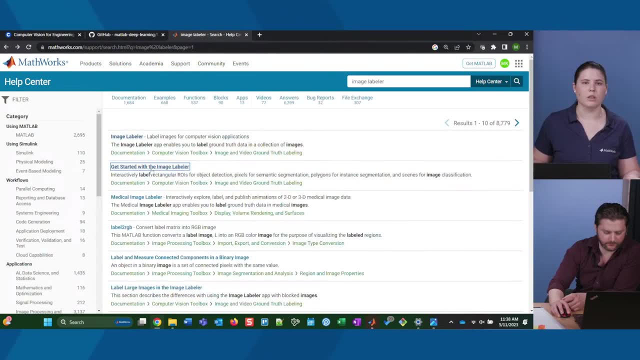 If you know one, you can know the other. and we do explain in course two of the specialization which is computer vision for engineering and science on Coursera. In course two we actually tell you how to use the labeler app. 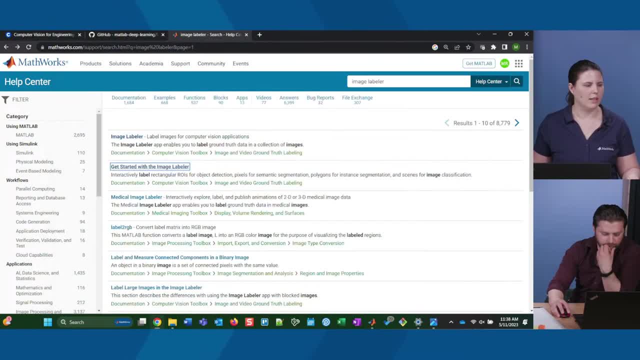 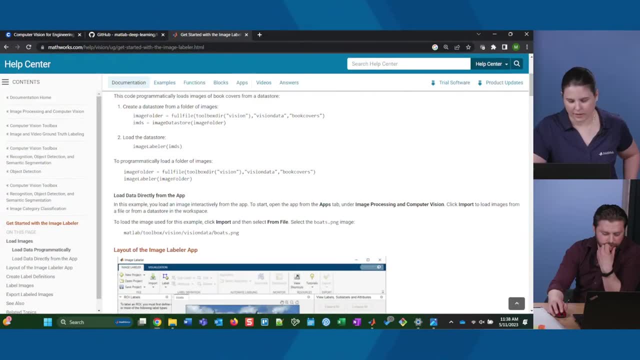 You get to practice using it on the example in the videos, I think, labeling railroad crossing signs, and then you get to practice it finding lumber defects. but yeah, you get to practice using it. It's really easy to do. I don't have a live demo of it. 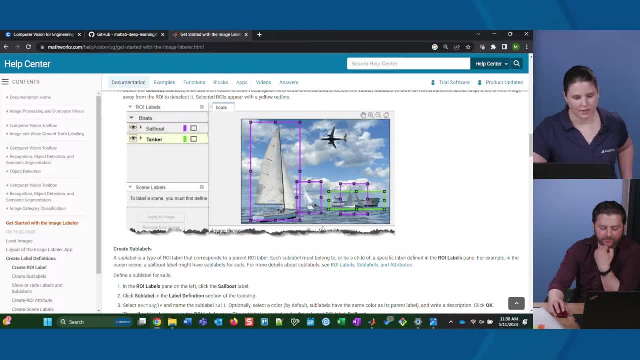 but if the doc page kind of gives you the idea of what you do, you draw your own labels. There's some actual in the video labeler. there's some neat functionality to actually try to estimate where the subsequent thing will be in the next frame. 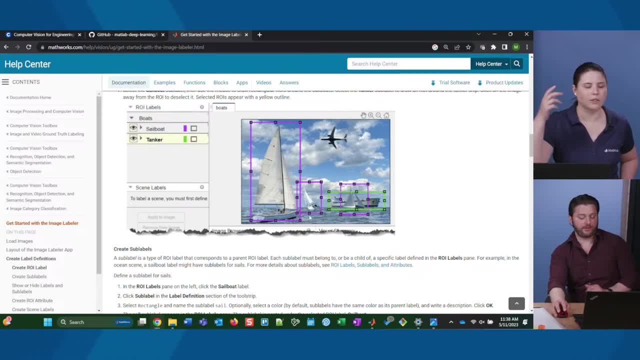 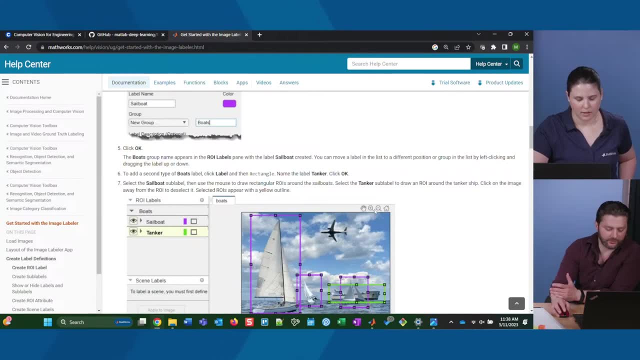 and auto box it for you. Yeah, so if it's close enough, you don't have to individually label every single part of the video. It's very, very user-friendly, pretty intuitive. We've got videos on it and there's good doc pages. 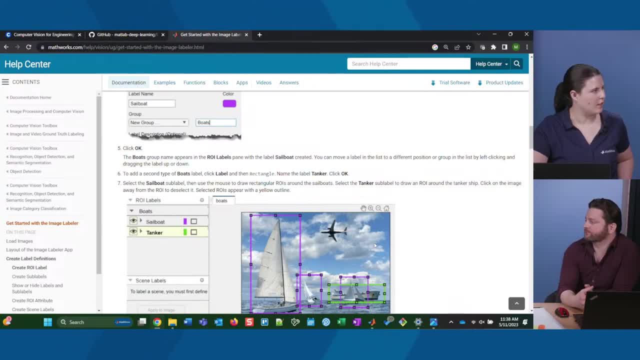 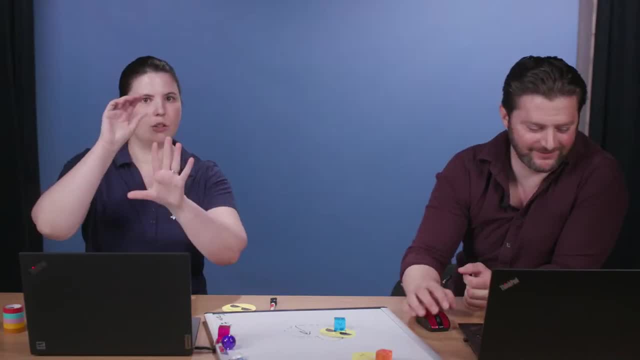 Can we detect different things at the same time, like persons and cars? Yeah, there's a great example in the course where it's a person on a bicycle wearing a backpack and it detects persons, bicycle and backpack and they're all overlapping. 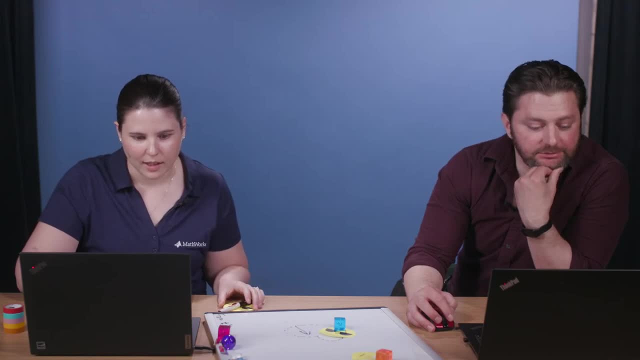 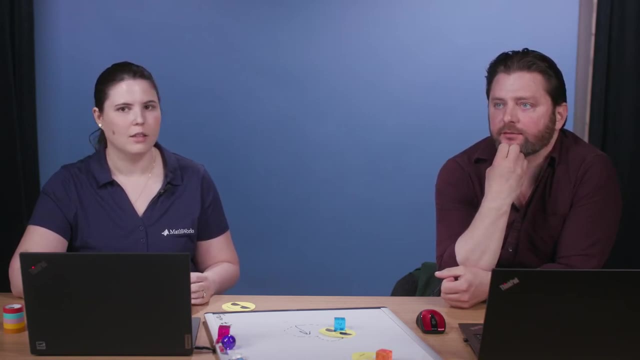 I could probably find it if I try. Yeah, Labeling tool. Can MATLAB be used for sentiment analysis? MATLAB can be used for sentiment analysis of text, for sure. In fact, we do that in another course of ours. It's in a. what is it? 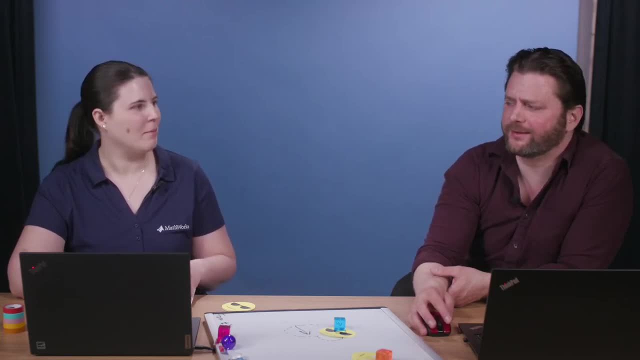 God, what's that? one called Practical Data Science with MATLAB or something? It's another specialization we have on Coursera, and I can't remember which course it is in, but I think it's probably in the course Predictive Modeling in Machine. 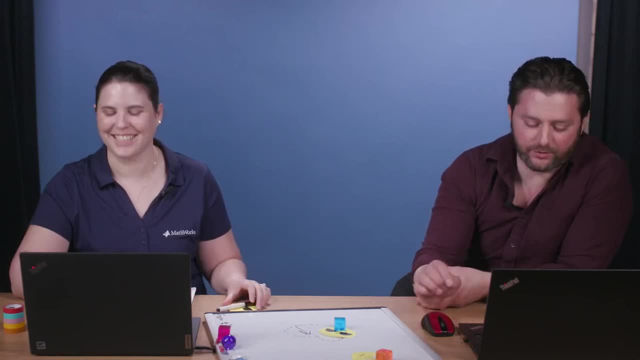 No, it might be course two. It's somewhere in there. It's in that specialization. You can do sentiment analysis with text. We do it with Shakespeare, sonnets and some other things. I think you mean facial sentiment analysis, and I believe MATLAB can do that. 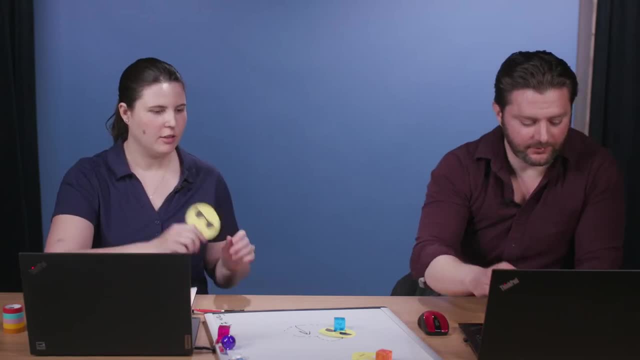 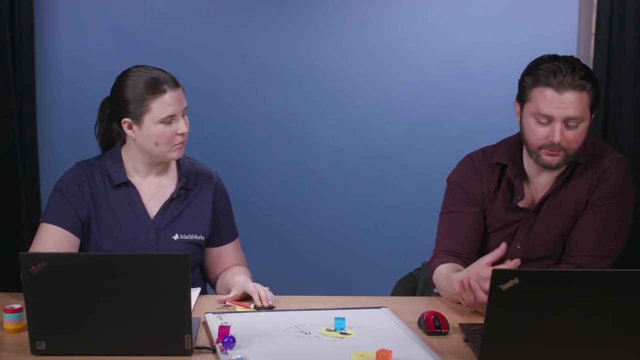 I haven't tried that. I'm sure you can. I should do that. We could find out, you know? I almost want to say one of these: Yeah, there's a pre-trained model for that. Yeah, Or you could hypothetically train your own. 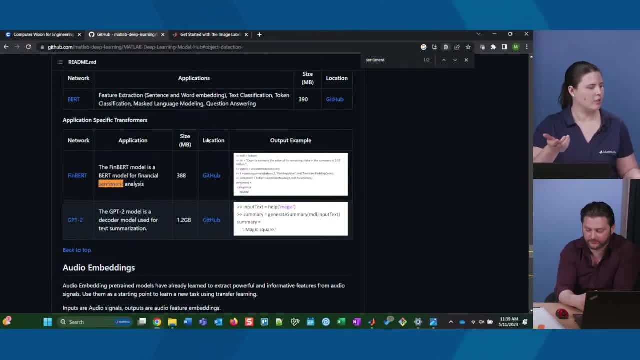 if you have the time and resources. I have used the facial detector a lot, which is very similar where it basically looks for that's face based on features. it detects around the eyes, around the nose, around the mouth, and it can track one person's face over time. 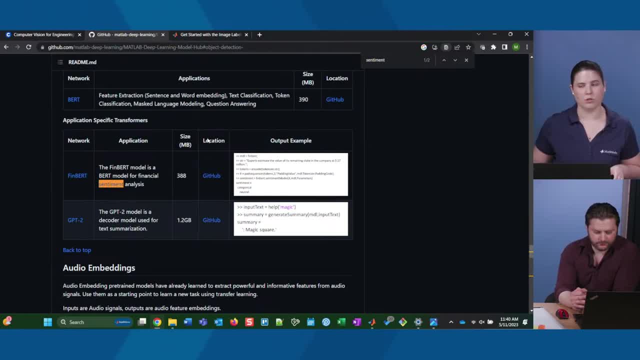 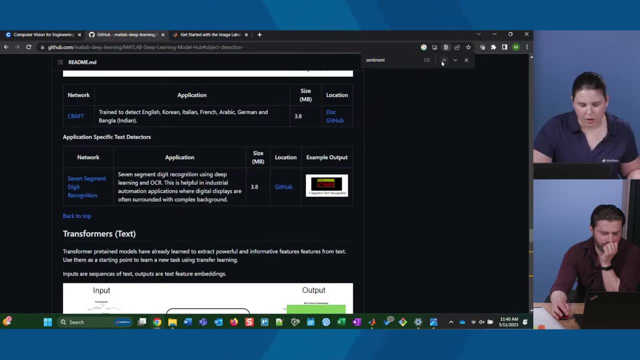 So that you know if you wanted to make your own sentiment analyzer instead of using the pre-trained one. that would be pretty useful for that. What about? is it at all possible to use the NVIDIA models or TAO toolkit inside MATLAB? 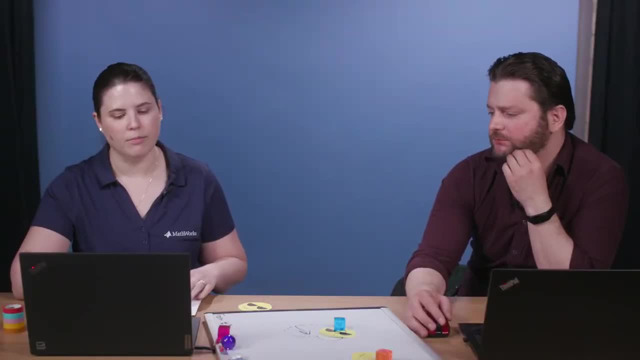 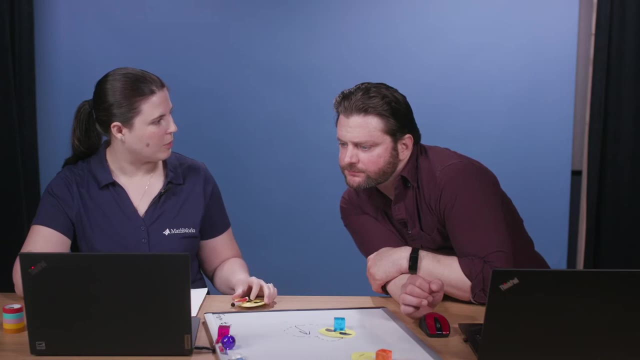 So I think you would have to deploy. I don't know, We'll get back to you on that one. I don't know the specifics of NVIDIA models. I don't know that off the top of my head. Do you know that off the top of your head? 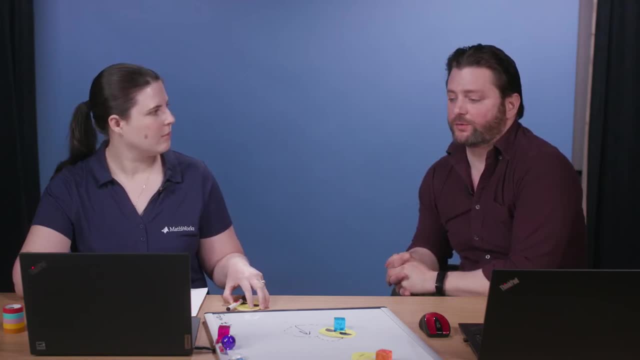 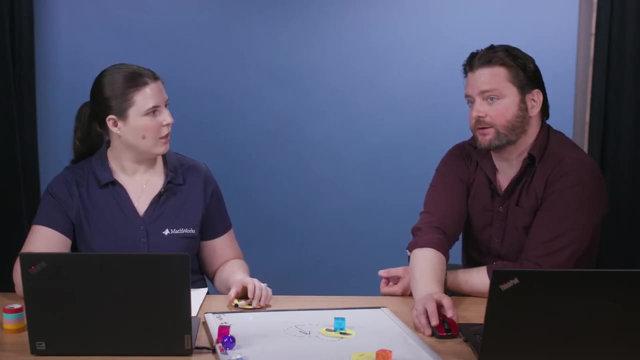 The only thing that I think of with NVIDIA is that it makes the GPUs. So if they're talking about, can we use NVIDIA GPUs? yes, that's actually the only type of GPU we support is NVIDIA. Oh well, that's handy. 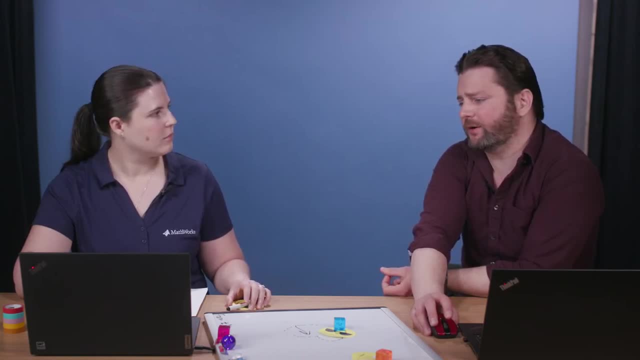 If there's specific models they want to import. I haven't heard of that, but we do have some tools to import third-party models. Yeah, I have done that, But we would have to get back to you on it. I mean, yeah, you'd have to ping us. 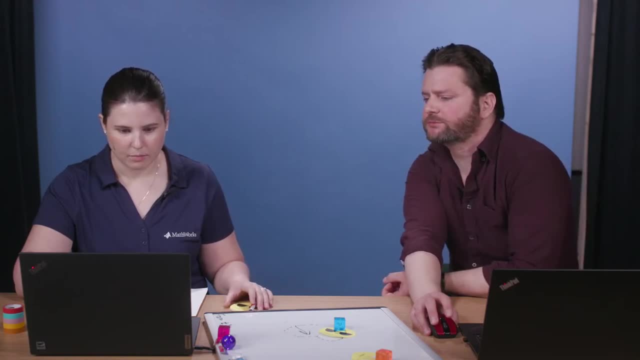 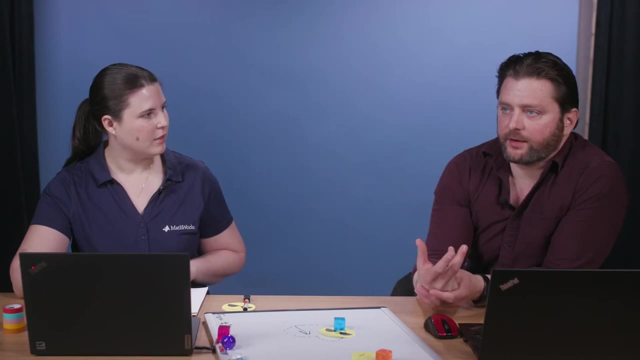 because I don't know exactly what you mean: A license to run on an embedded system. Do you know anything about embedded systems? That's kind of out of my wheelhouse. There's not a license to run your model on an embedded system. 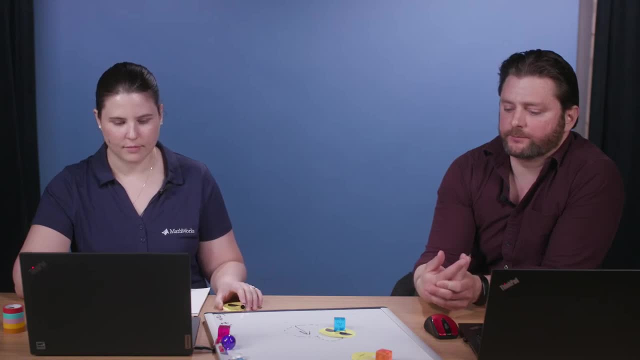 but there would be a license to generate the code to go onto the embedded system, But there's not a separate license to run it once it's there. You would just have your license to generate whatever GPU code or compatible code you needed. What are? 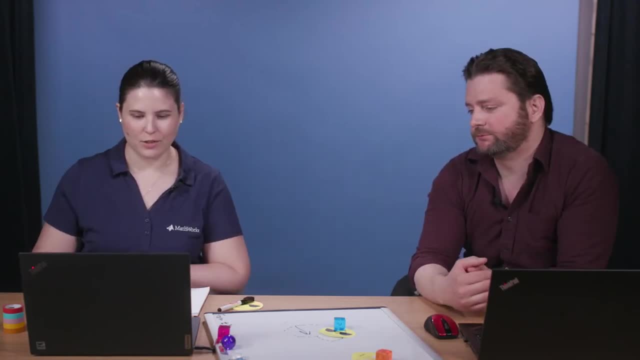 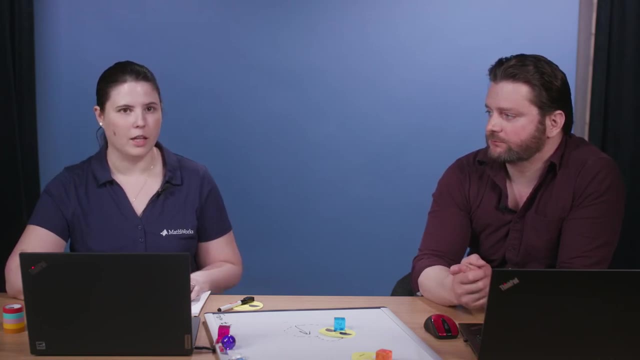 Oh sorry, And then you could put it on your embedded system. What are the advantages of doing these real-time detections and tracking in MATLAB instead of the example in Python? I would say right off the top of my head, MATLAB has support. 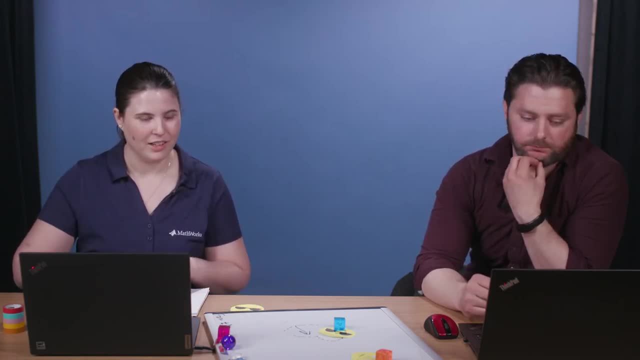 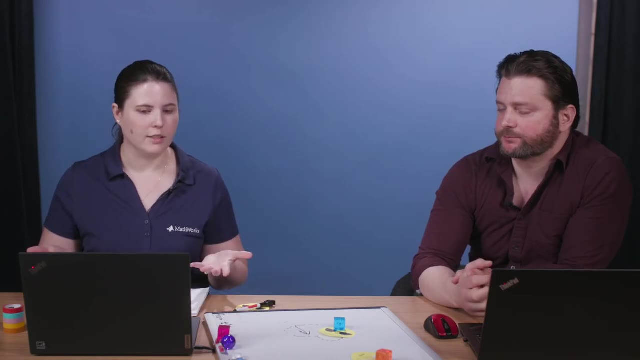 So if you can't get it to work, you can contact someone at MathWorks and they can help you out. I have used that several times myself when I was figuring out these concepts for the first time. It's all centralized and there's a lot more apps available. 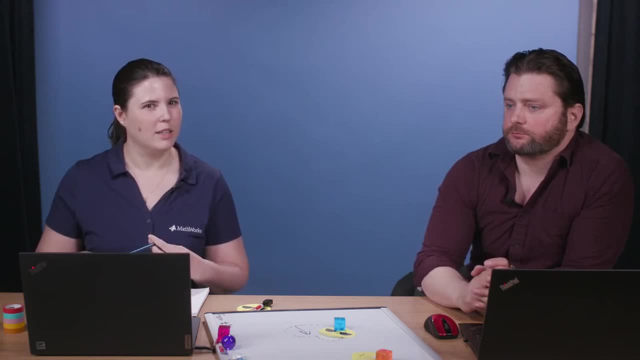 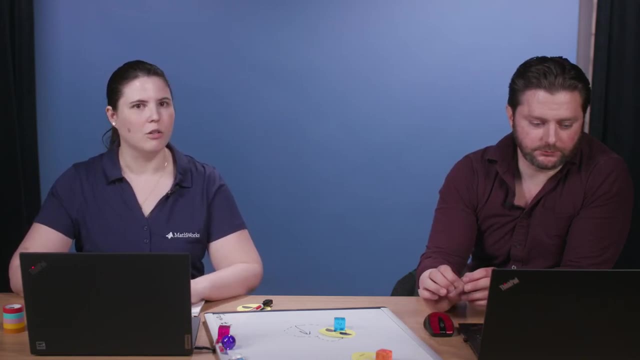 that, since most of Python kind of relies on third-party stuff, doesn't get updated very much. There isn't a lot of good app work, So it's just For me it's an issue of availability whether the code is super sketchy. 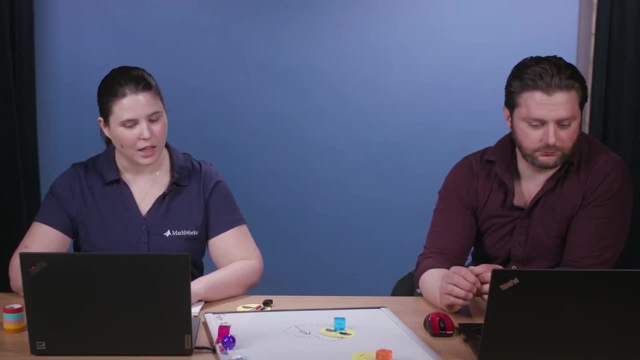 which sometimes third-party Python packages can be, and ease of use. But you know, Yeah, I would definitely Plus one, the support aspect and also just the larger product. It's not even just that there's apps. I mean, if you're doing research in a lab. 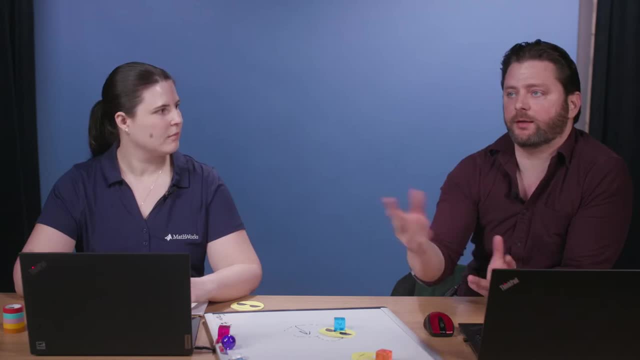 and all you really care about is one deep learning model or you're going to make your own. I mean, hey, maybe you don't need MATLAB, but you could still use it. But if you're a working professional or you're going to work with anybody else, 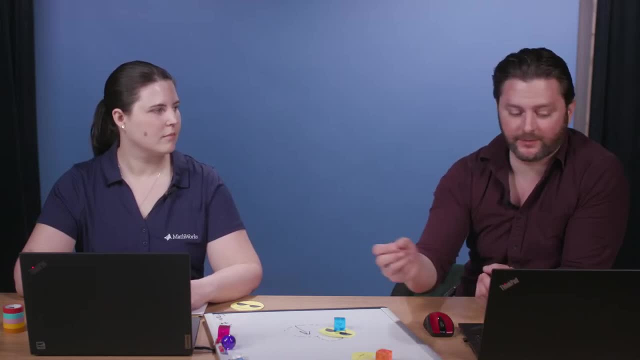 what MATLAB offers you is this ecosystem. It's kind of an end-to-end product, right, Like you can do, Like I was mentioning, CodeGen. you can deploy, you can do testing. We have all sorts of other products and toolboxes that integrate very well. 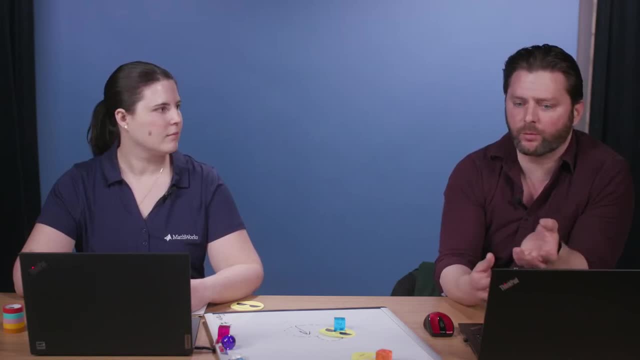 with the deep learning toolbox, So you don't have to do any of your own work to get different things working together. We make sure they work for you and then, if they don't work for you, you contact us and we make them work for you. 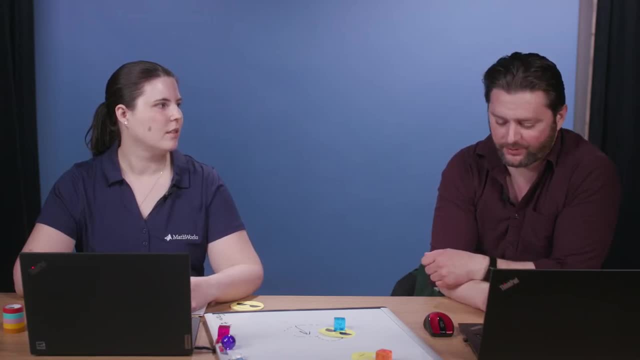 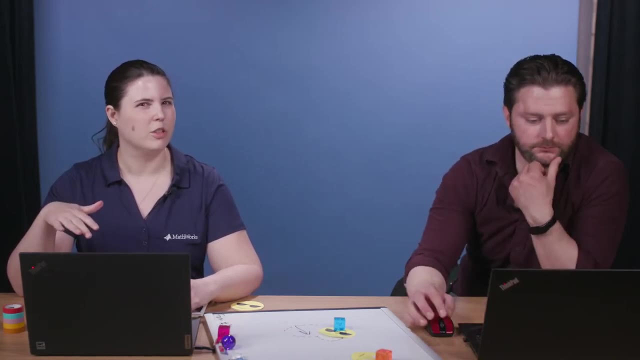 Whereas you don't always- Well, you don't get that kind of support most of the time with third-party stuff, And there is something to be said for the MATLAB ecosystem and community. Two of my first three research projects back when I was still a biomedical engineer: 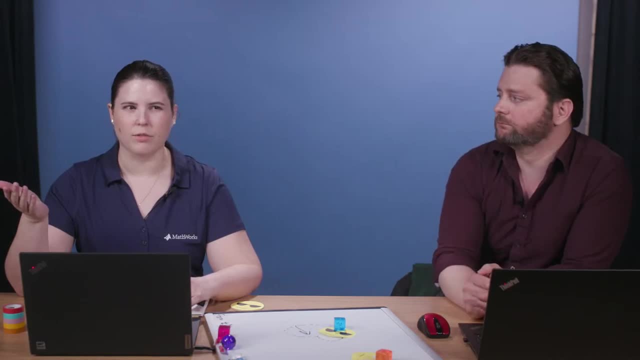 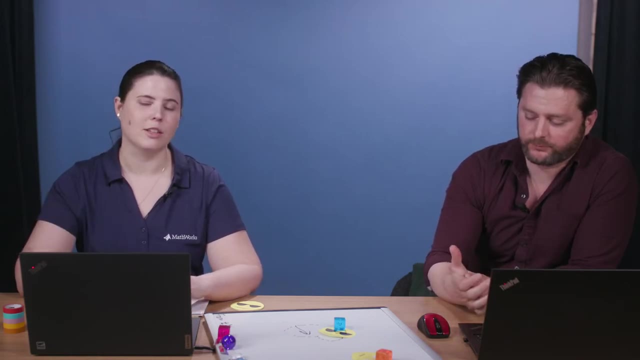 were somebody wrote this code that does something very specific in Python and no one else at the university can use it. Megan, can you translate this into MATLAB? Unfortunately, this was before there was more code generation capabilities, which now MATLAB can do a lot of that automatically. 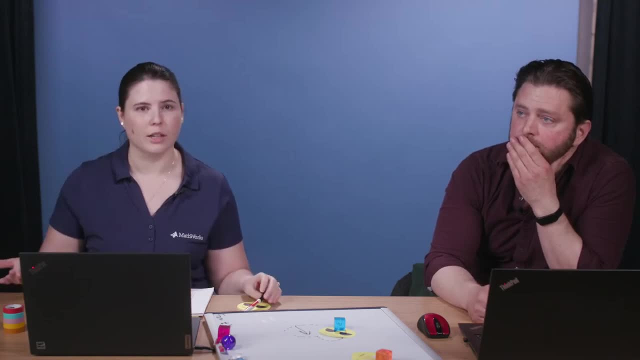 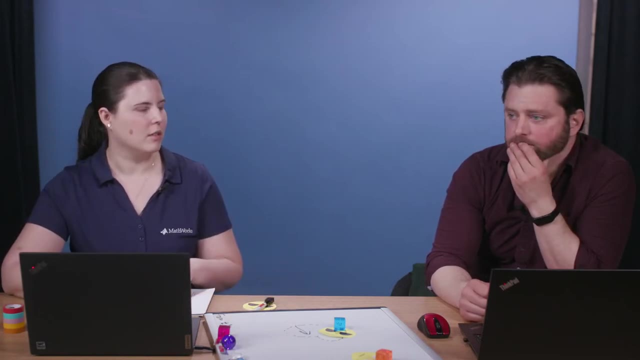 But a lot of what I was doing as an undergrad and grad student was putting it into more usable form using MATLAB's graphics, user interface, things like that, And so there is some sort of back and forth, but it is helpful to have other people. 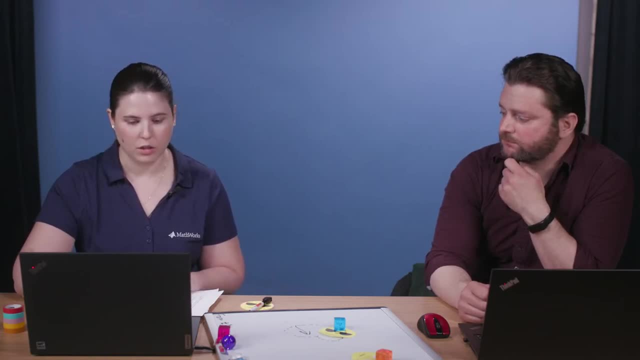 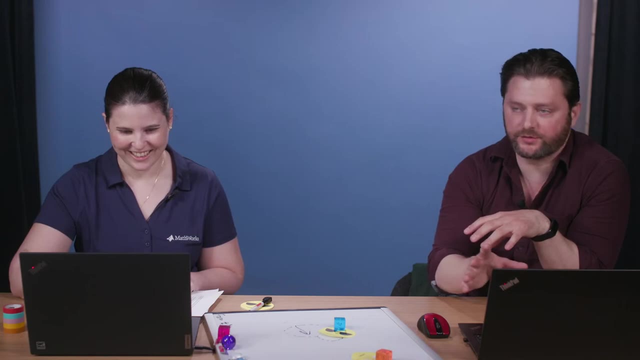 at the university be able to read and understand and use your code. And for a good section of industry I'll just say the word simulating. We're not really doing it here, but all this computer vision stuff that we're doing, all the deep learning stuff. 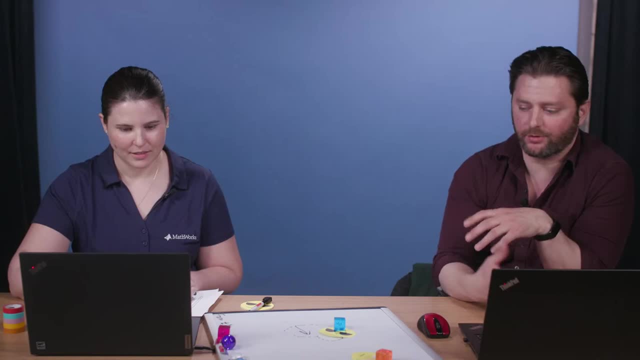 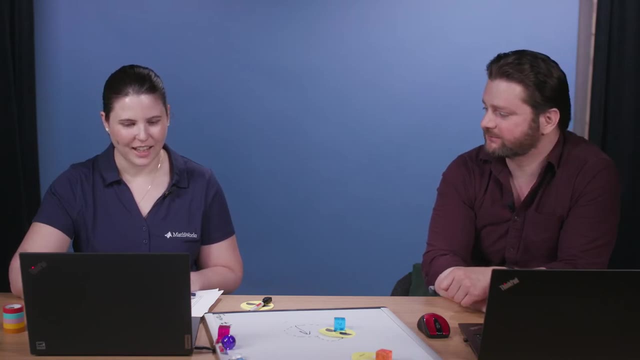 you can do it within that modeling framework. You can do all the hardware in the loop, software in the loop, model in the loop, all your favorite testing methodologies and model-based design stuff. Have you tried your algorithm with objects that reflect itself? 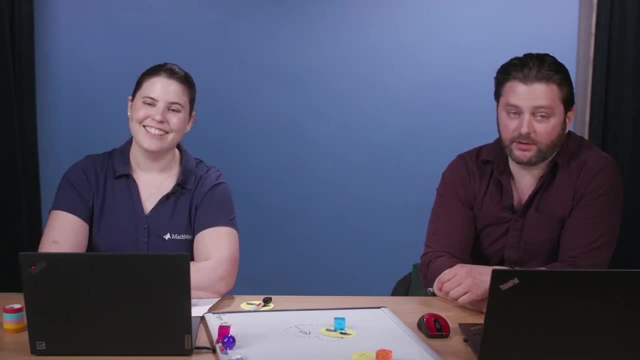 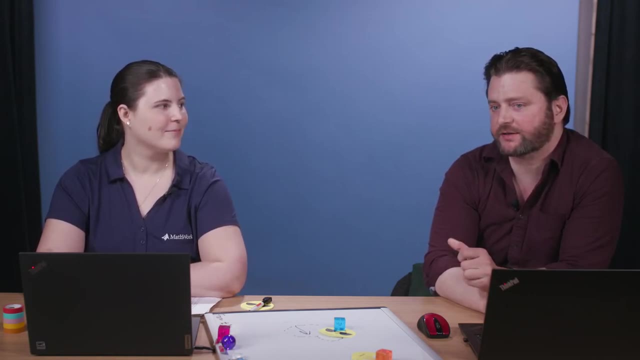 windows, silver fridge, et cetera. We didn't do it on purpose, but we were practicing a little bit yesterday in a conference room and it does occasionally pick up reflections of us in the window, So we didn't have a window behind us. 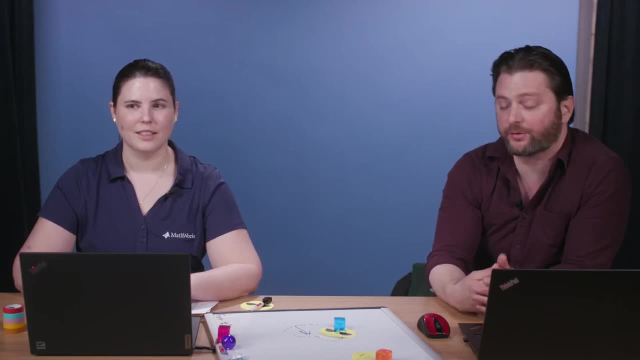 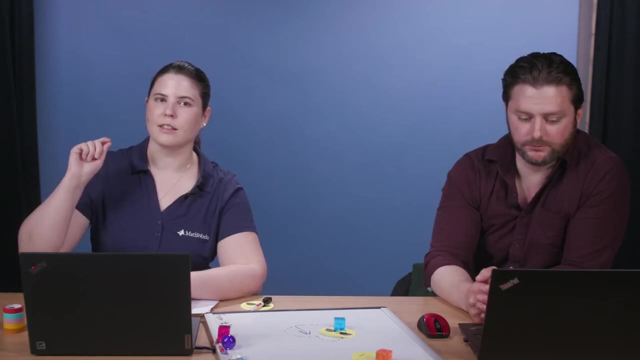 but when we put the reflectors, we could see that the reflection was there and that's what we were looking for. So it's a little bit more complex of an algorithm that's used to do this today, but had there been human looking reflections? 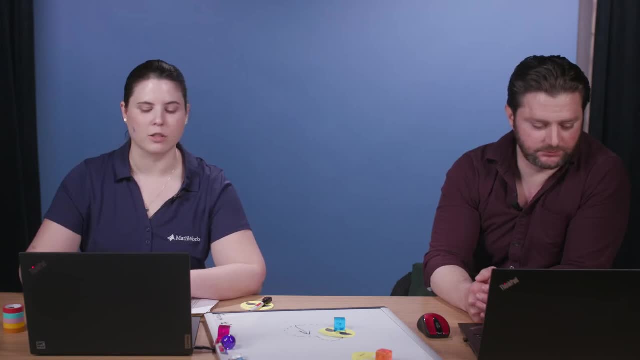 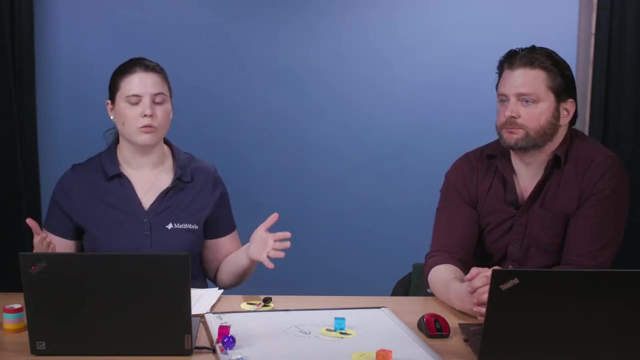 the model would have most likely picked those up. It detected them and then, if we stayed moving, it tracked the reflection as a different person. So it never mixed us up with the reflections, but sometimes it did think the reflections were a person. 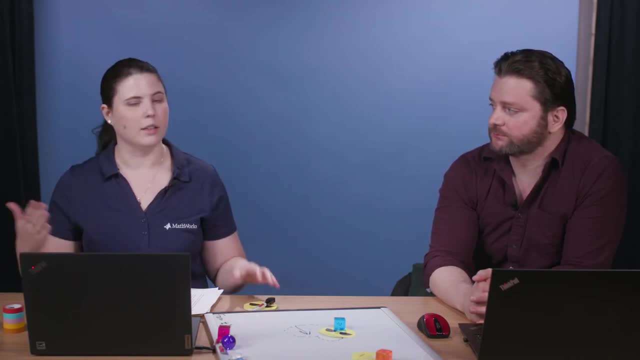 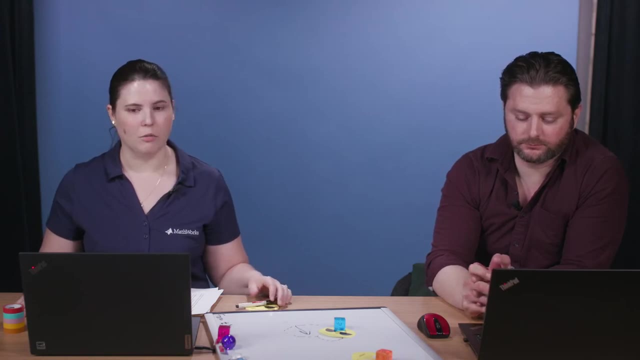 And you saw that YOLO can detect mirrors to make it a little less sensitive. so something has to be really persistent to get tracked if you wanted to get rid of the reflections. but we actually thought the reflections were kind of cool because it's like oh it, you know we 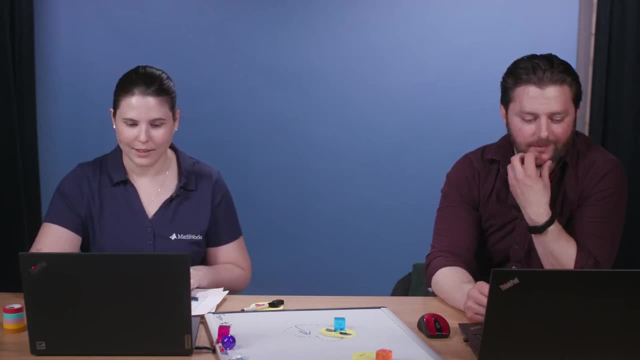 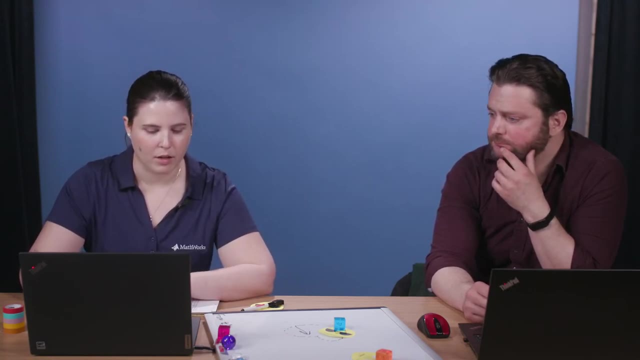 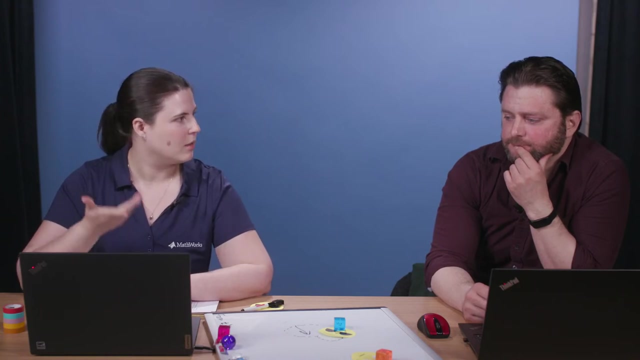 didn't get a chance to practice this with four people, and now we can see. then there was a question about Julia, which I've never used. Julia, I come from academia, so MATLAB is by far the most prevalent, but have you ever used Julia? no, yeah, isn't it a graphics thing? that's about my level of familiarity with that. 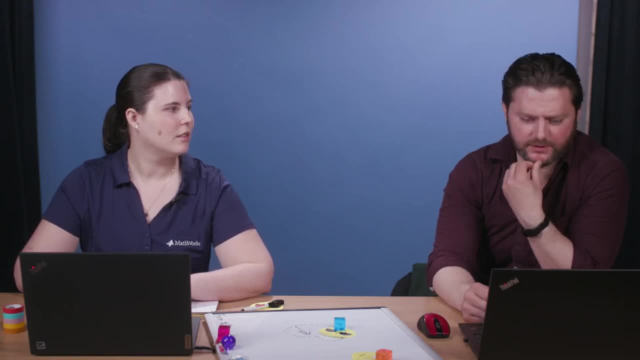 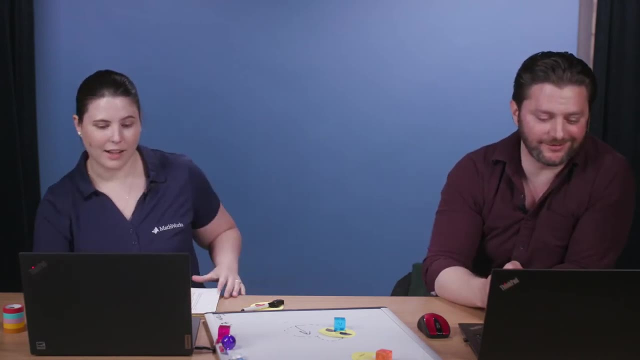 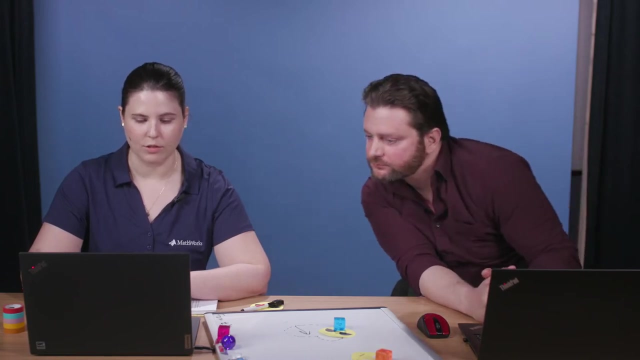 I thought it was a package for visualizations. I didn't know that Julia had anything to do with computer vision or deep learning, but that's again. I guess neither of us can answer that. Brandon has answered it too, as you said that you can continue to. oh no, that was with when answering questions. yeah, so.